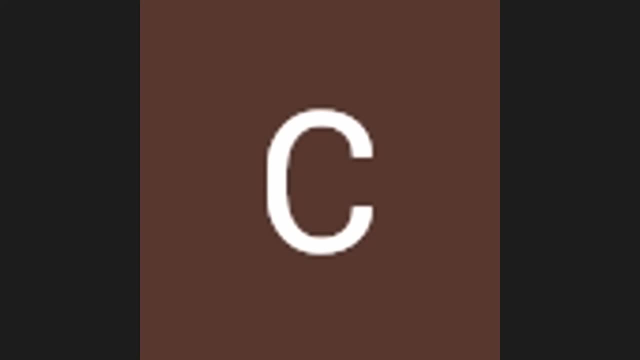 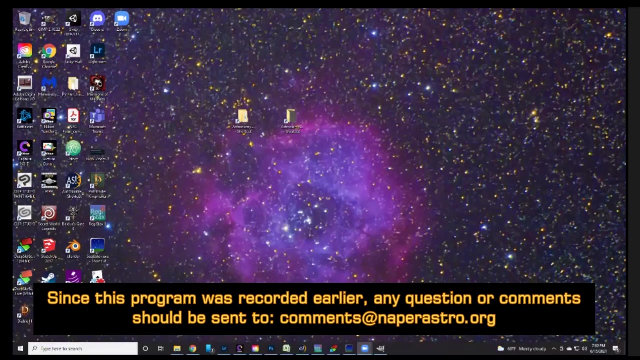 off my video And then I will be sharing my screen. So please remember tonight, if you do have questions, post your questions to either the Facebook chat or you can also send your questions to the Naperville Astronomical Association's groupsio email box. 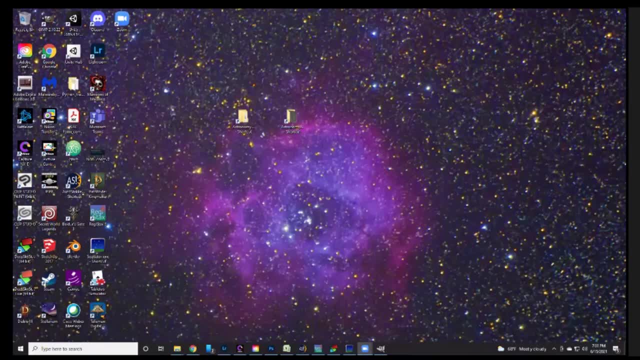 So I would like this to be an interactive presentation. So, again, please do submit your questions for that Also afterwards. it's being recorded and will be posted up to our YouTube channel, the Naperville Astronomical Association YouTube channel. Please go there. 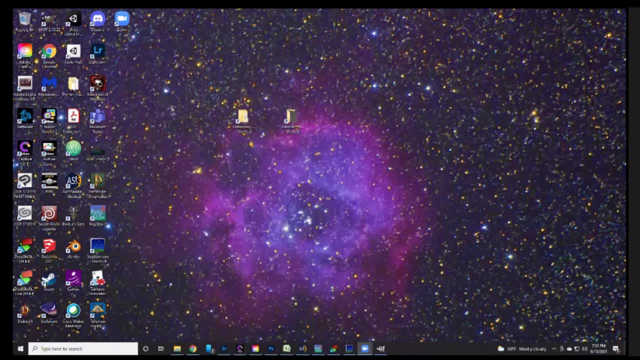 for your later reference as well. Please like, share and subscribe to our channel. So I'm going to get right into it. the first, a bit of a lecture about, uh, taking your images. um, the first thing is why raw format images versus jpeg, and something i've covered before in one of our earlier presentations. 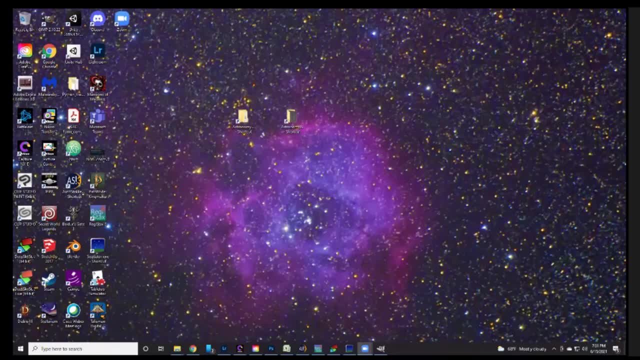 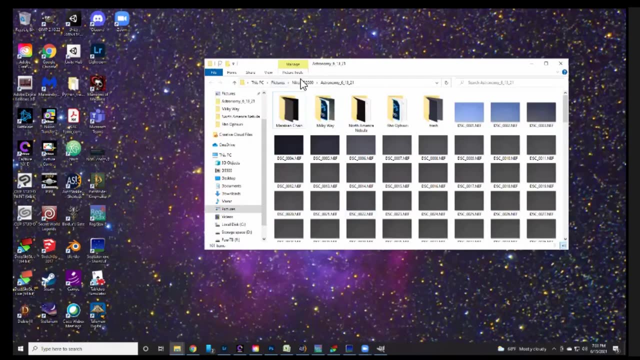 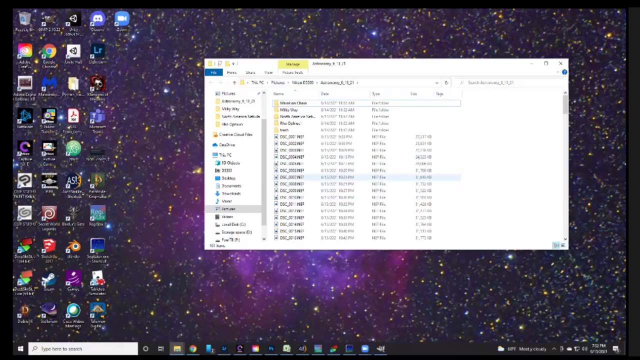 uh regarding this, and there's a couple issues about that. uh. first, uh, the images. yeah, they're big uh in raw format, but you can see here they uh are pretty large-sized files, but disk space is cheap these days, so, uh, it's not as much of an issue as it used to be, and so uh, 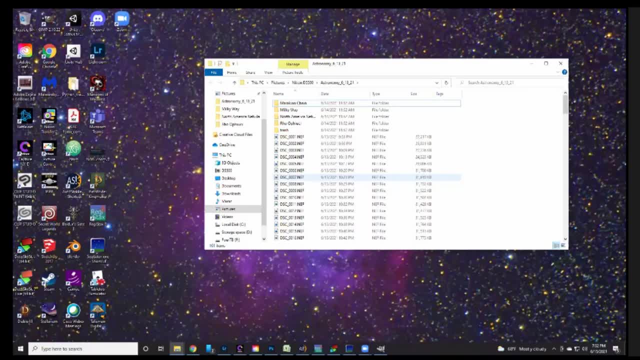 you're. the second issue with raw versus jpeg is the more important one, which is what we're talking about tonight. so jpegs are typically processed and they're not- uh, they're not, uh, they're not in your camera. so whatever logic they put to trying to process an image to make it look as 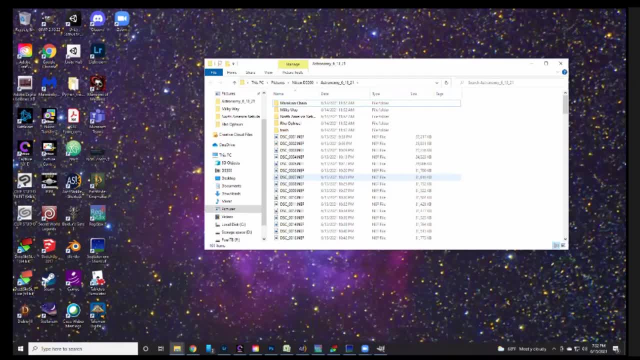 nice as possible. they apply that and you lose data. so therefore, if your images are jpegs, you're going to lose some data and you're not going to be able to manipulate your- your images as well as you can with raw. so i use a nikon d5500 camera and the raw format is dot n e f, as you can see here. 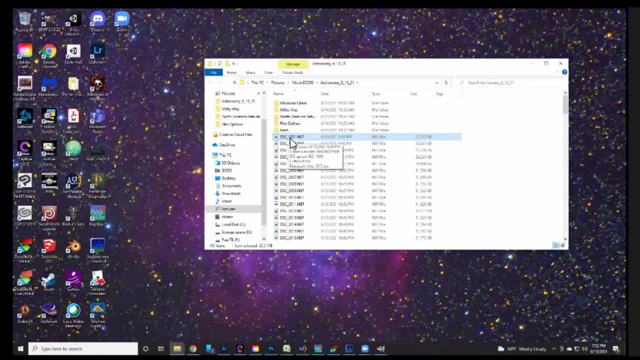 uh on my screen. uh, hopefully you see that. uh, let me know if you don't, and uh, anyway, so so that's what my camera uh produces, uh, dot nef. that's the raw format and that's nikon specific. so canon is different. every each camera has pretty much its own uh raw format. uh, so you'll have to. 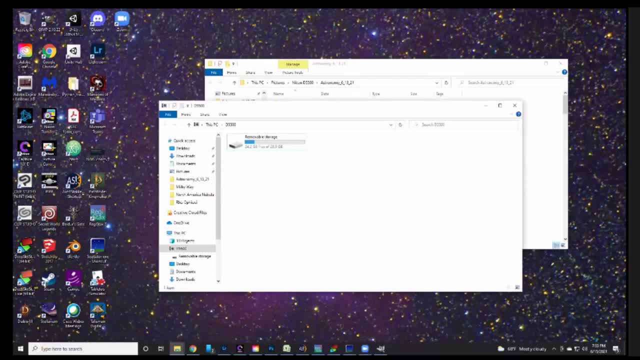 just see if your camera does that. so the start of my process, of course, and i'm not going to make us sit through this all, but you can see the last time i went out, imaging i- uh, this is my camera card that i'm pulling up, right? 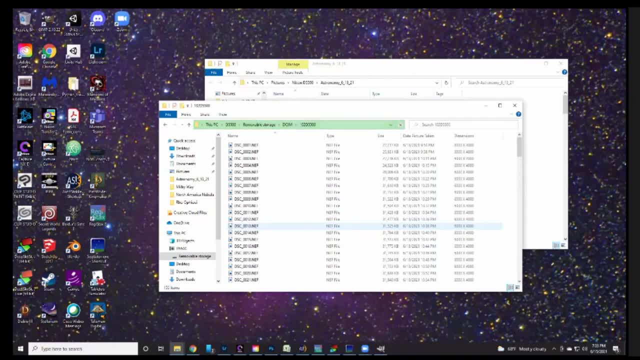 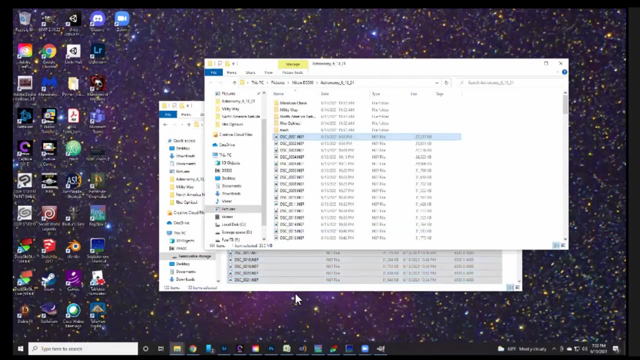 here. i took a lot of images that night. uh, not horribly so, but there's a lot of them. so if i, if i select all those 155 images, that's not too many, but there's sometimes where i'll have over 300.. but uh that what i do then is take those and move them off the camera, mainly just to create the space. 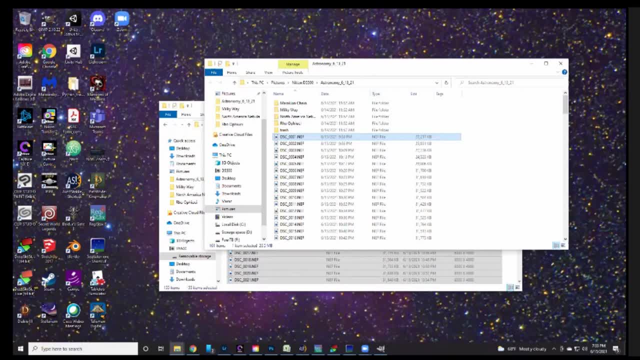 and to get them on to my hard drives in my system, which are, uh, faster heart ssd type hard drives, so whenever you're processing them it's going to be a lot quicker. so, as you can see here in this folder, i right away try to remember what i was imaging that night and create folders appropriate for the. 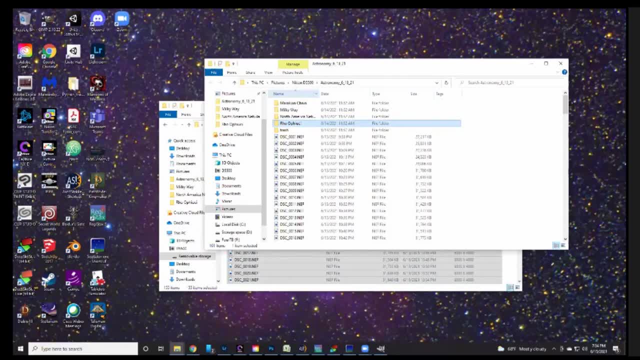 targets that i was shooting and then, um, that way i you know, i can go back later and do a search for targets if i want to do something else with it. uh, and you can see, i have a trash folder because almost every night ago, uh, imaging, i end up with some trash uh images and uh, this particular night, 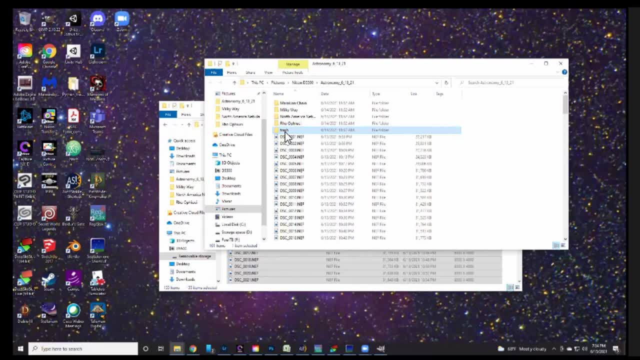 that i'm showing you on my this particular folder. uh, almost the entire night was trash, so i had very little uh quality images. unfortunately, it was a beautiful night, but that's what can happen. so that's one of the first things i do uh when i start my pro uh processing on my images. uh, one of the other things i do uh. i'm gonna start off with. 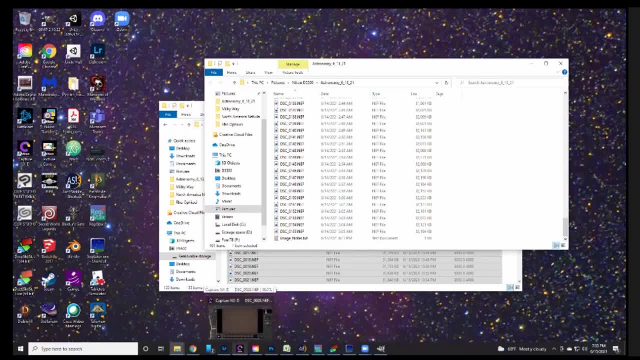 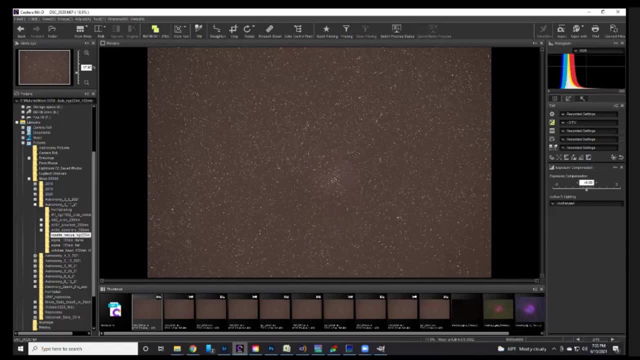 talking about some of the software i use. i used to. when i first started doing natural imaging, it was just simply use the software that came with the camera. so this is the nikon product called capture and it- uh, it basically lets you do an image review whatever comes out of the camera. 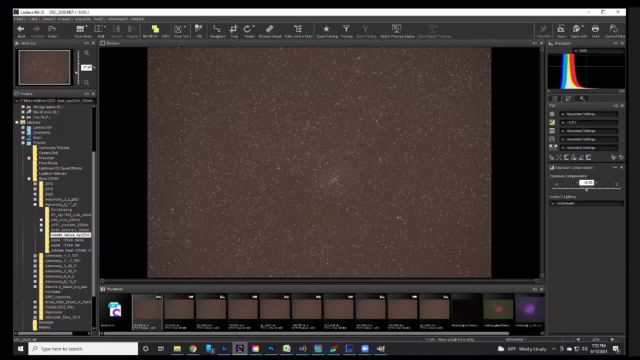 and uh, you can see, here is an image, uh, that we'll actually work with later, a little bit later tonight. uh, in the software, and with it being a raw format image, you can see that i can still go over here and make some minor changes to the image. 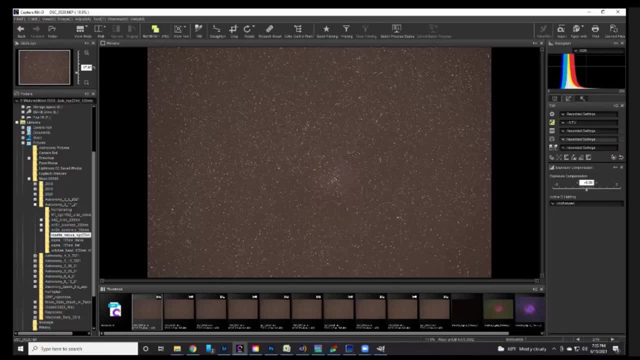 uh, as much as exposure, i can do the white balance, i can change some of those basic settings, uh. and also, let me know if you can't turn on my screencast. but the, you can change those and it's very simple, very basic editing, uh, you can't do. 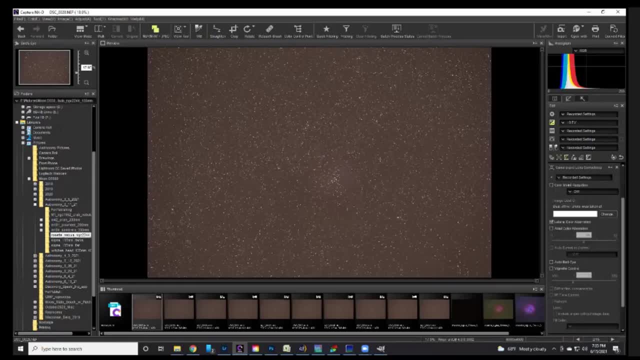 a lot. uh, there are some additional buttons here that you can go through and try to do some some of the manipulation that most people will do with their astro images. uh, it's not the best tool, but it's. it's a tool that comes typically with everybody's individual. 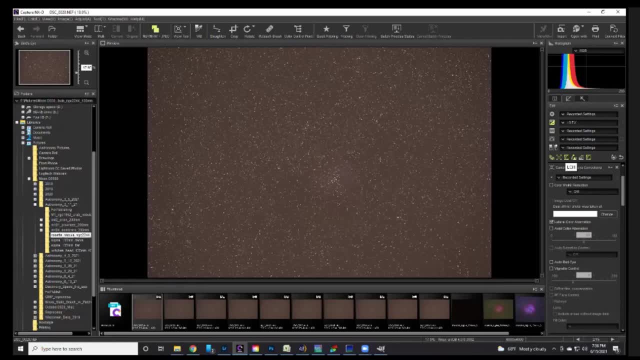 camera. so, uh, it's, and it's great for processing maybe a single image. if you got one image, that's, you know, maybe all you need to do. and if you, if you did, capture your images in jpeg, this may be all you'll need as well because, like i said, the camera will have already processed a. 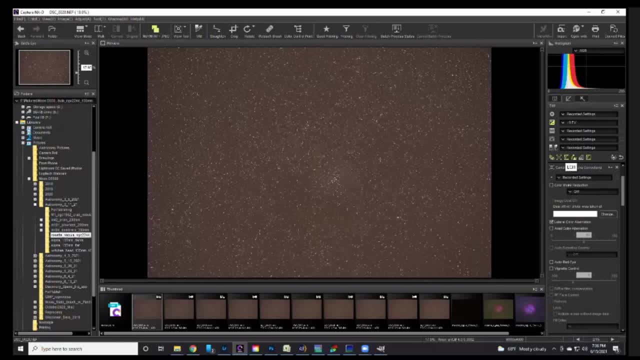 little bit and you, but you won't be able to change too much with this and you won't be able to do a lot of detailed stuff. so, uh, and again, it may be sufficient. if you've got really good images from the start, then that may be all you need to do. uh, so one of the key things that i do would like to. 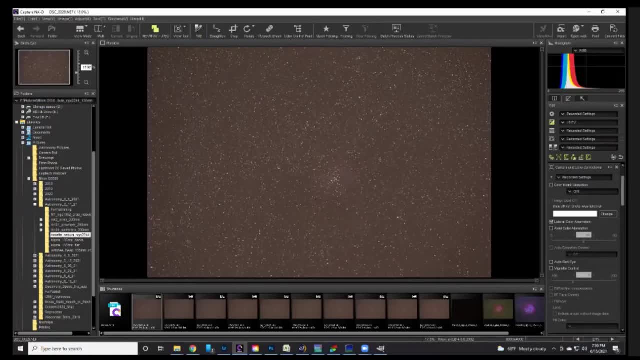 show on this app is this histogram, and this is the histogram. uh, this is one of the key things we're going to keep working with all night tonight. uh, during this presentation, this histogram shows you, uh, the image data that was collected in the three bands- the red, green, blue and, uh, and this is. 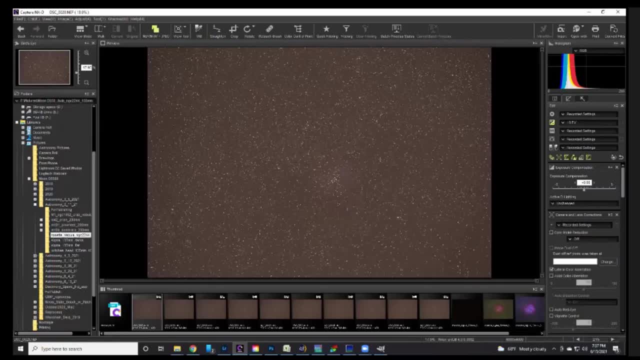 actually what would have been displayed on the back of my camera. the night i took the images. so, uh, what you want to do. if you notice it's broken up into four different quadrants and when you're taking your images, you want that- this diagram to try to get in that. second to the from the left side of the uh of the graph. 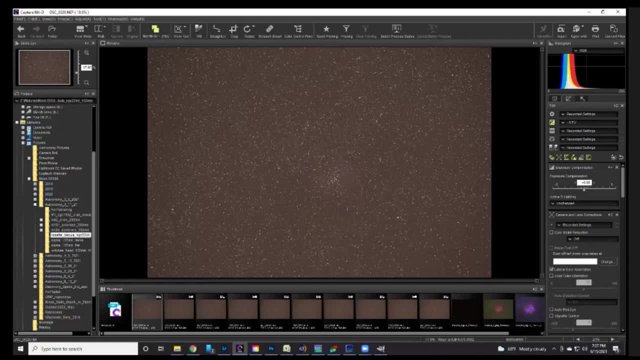 so on the left side of the graph is your darks, which you can see here is zero, oops, zero. there we go, and then on the right is 255.. so zero being the blacks, and color or white is 255.. so, uh, if your images are in this second quadrant, uh, you're probably going to have some halfway decent. 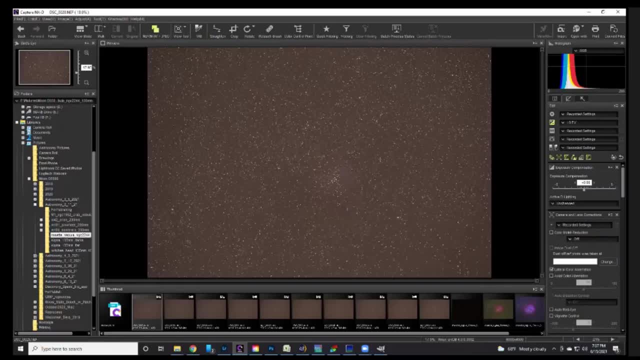 images and something to work with. if it's all the way to the left, it's really too dark, it's going to be really hard to process that image, but you still might be able to pull something out of it, especially with some of the tools that we can look at a little bit later. so, um, uh, i think that's. 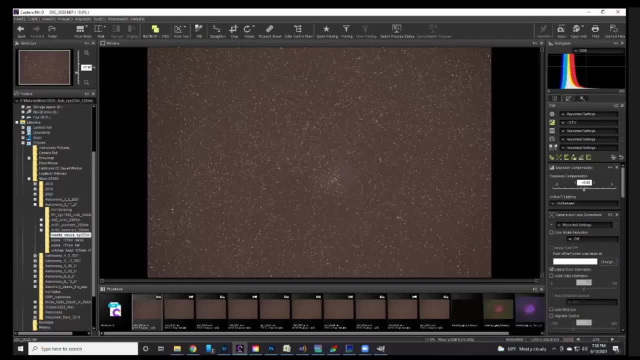 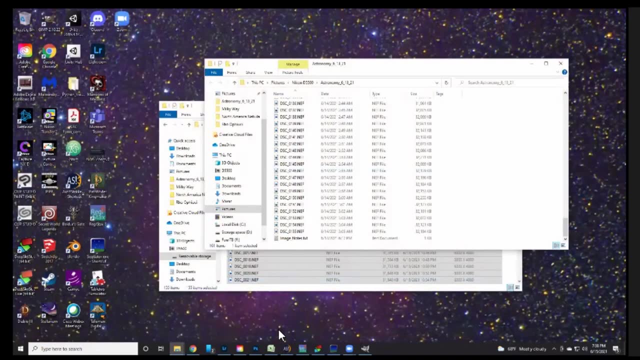 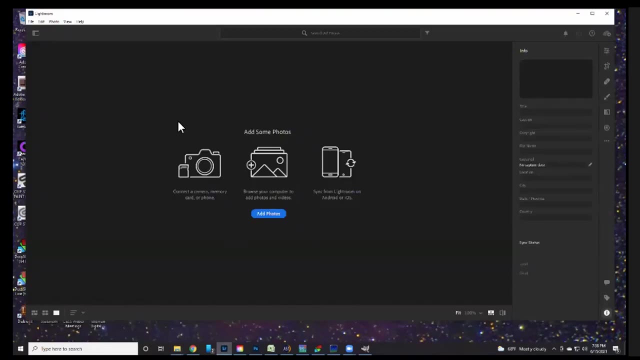 pretty much all i want to kind of cover on that. this is again. i'm not going to spend much time with this product. this is again specific to nikon um, so one of the first things that i do and i would capture. but i also have another product which i like to use which is called lightroom, and what i 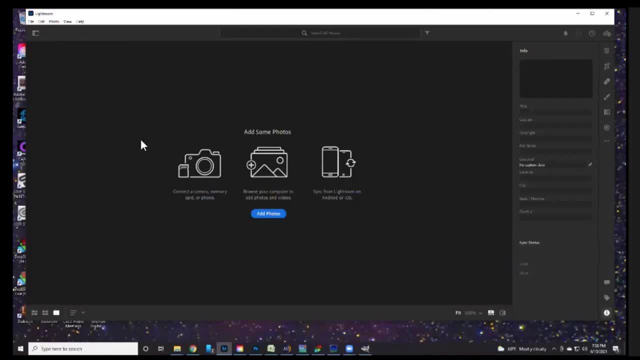 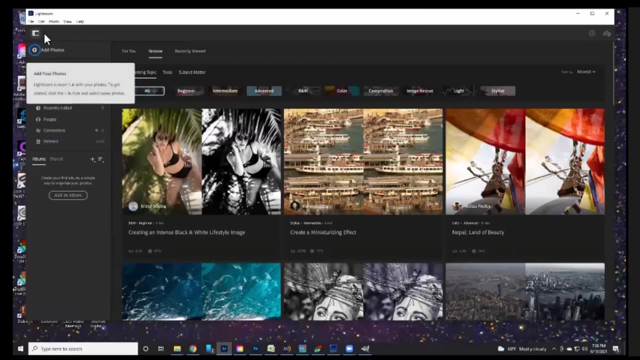 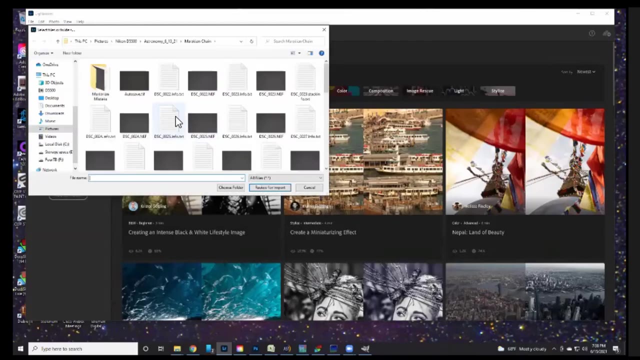 would do would load up all those images. so, uh, i will do this a little bit here. it's because, what i, it's a little faster. uh, i'm sorry, i put the wrong thing there. um, what i, what i will do with a night's worth of images is to uh, 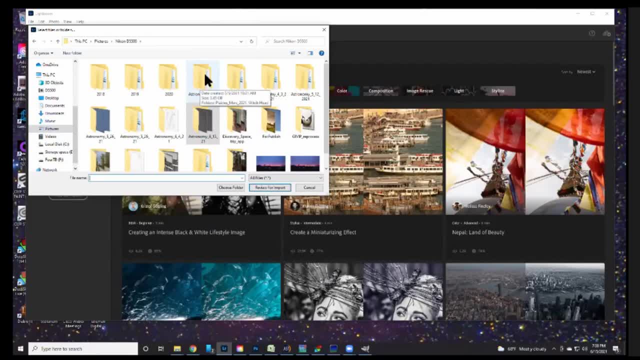 first of all, i did forget to mention i was going to go over the folder structure. i do notate when and what i did normally, so, uh, that's in general, what i do with that, uh, the. so what i will do is load up all the images that i want and, as you can see, i've already stacked. 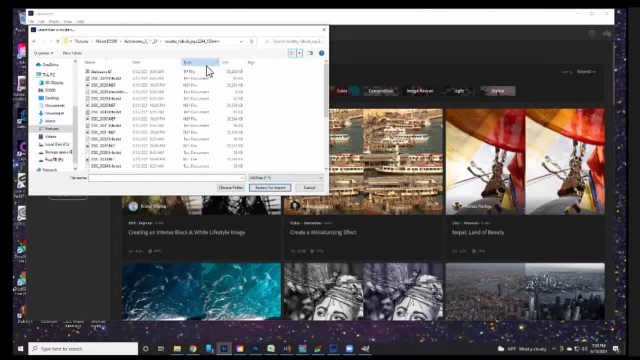 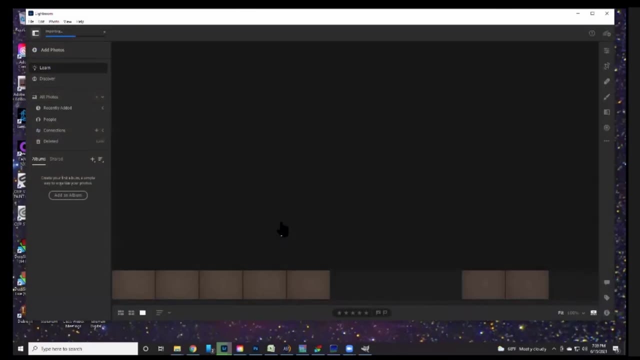 this once before. so i'm going to switch it to details and sort it by the type, and then i'll be able to load up all my raw images here. so i only took that night of this target only. let's see me: uh, 10 photos, only 10 photos. so, uh, that shouldn't take too long to load up. and what i'm looking for. 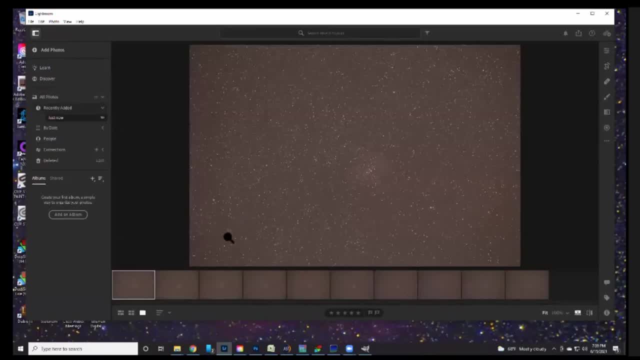 when i'm looking at these images in lightroom. so lightroom's an adobe product. it's- uh, it's- a pay-for product and it'll let you do just a little bit more than that nikon product and it is getting constantly enhanced by adobe and you can do some more fancy stuff with it, but not as much as some. 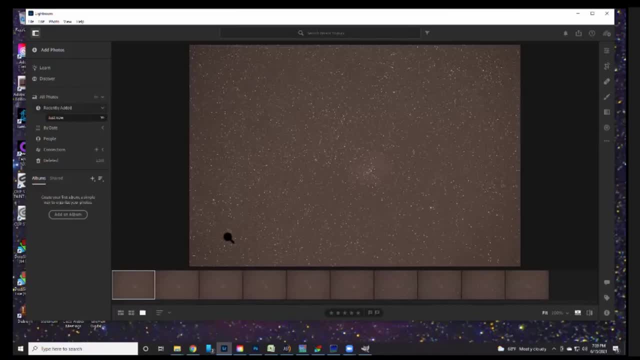 like photoshop. so, uh, what i'm doing when i first look at my images, uh, is how well aligned all my images are. so this is what i call my image review, and, uh, so what i would do is just flip through the images and see, you know, do i have any streaks from satellites, from planes going through, or do? 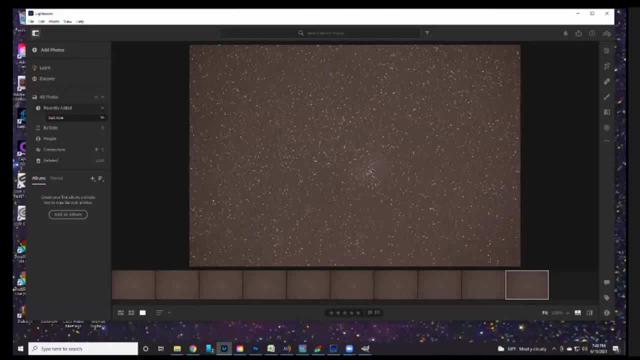 i have any kind of clouds in the image, whatever it may be. so what i will do is i'll pull those out, i'll put them in a different uh folder. most of the time i'll have a setup image or two, in other words, where i've taken an image where i don't quite have my target centered properly, or or i'm 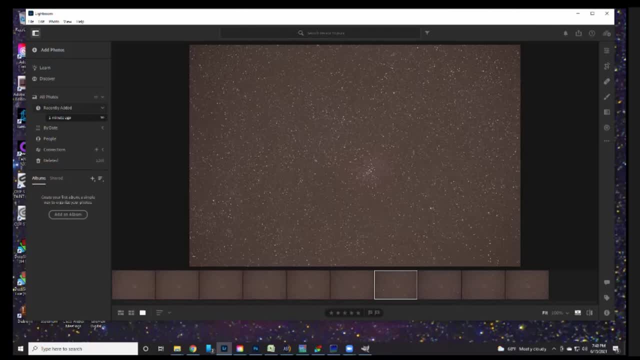 making small adjustments to try to get it in the center of the image. so, and again, i keep those just in case, but i typically i'll end up throwing those away. um, so, image review is just simply to try to make sure you're getting it down to your first, you know, your best images that you have, and then 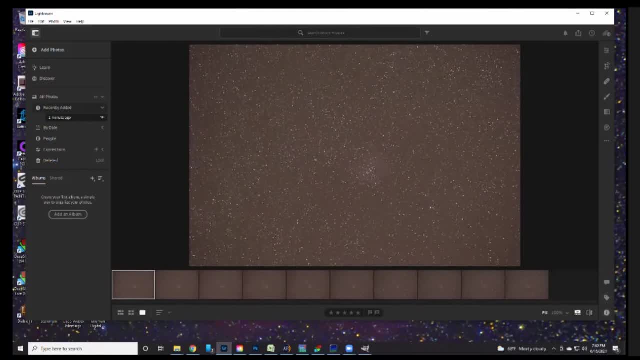 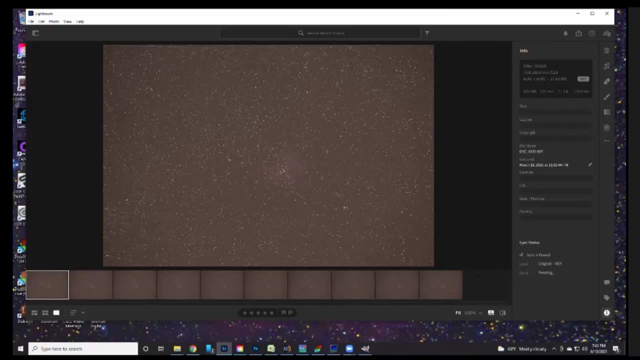 come into play later. another thing that i do during this part is: uh, i will take note of what i use to capture this image. so, in this particular case, on on here on this light room, it shows you that it was shot at iso 400, the focal length was 135 millimeter. lens that i used with a f2 2.8. 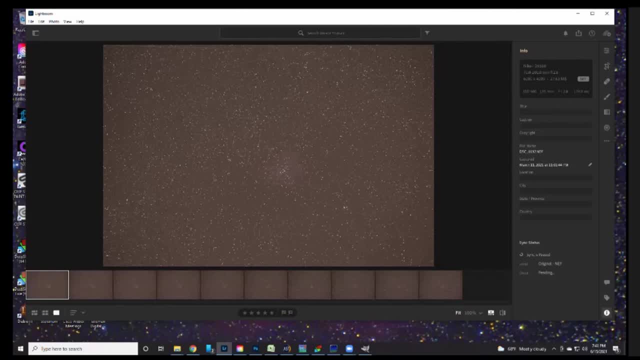 focal ratio and then i took 179- probably actually a three minute exposure- uh to capture this uh image. so i notate that only because i end up posting a lot of this to sites that have detailed information about images. sometimes i do, sometimes i don't, but 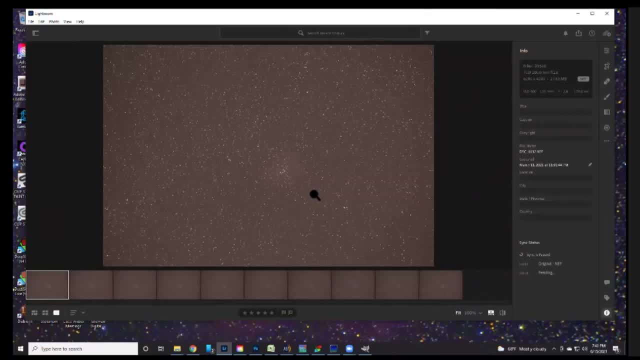 a lot of people will post that information for other people who want to go back and and try to capture those images as well or create their own version of it, and so i just simply notate that in a notepad uh file and i keep it with. 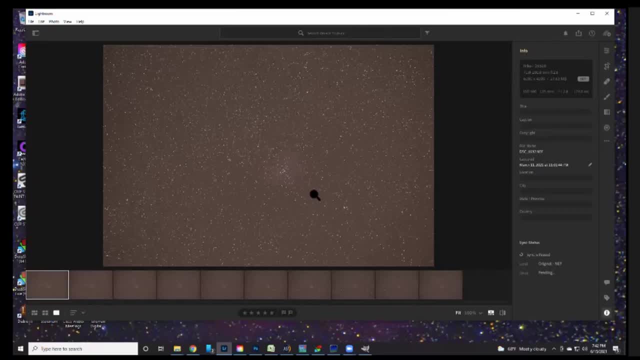 the pictures and uh, what i'll you'll see later. i i name a lot of the images with that information embedded in the name of the file, just so i can keep track of it. and uh, and it comes into play later with what i call my final step, which is reprocessing, which 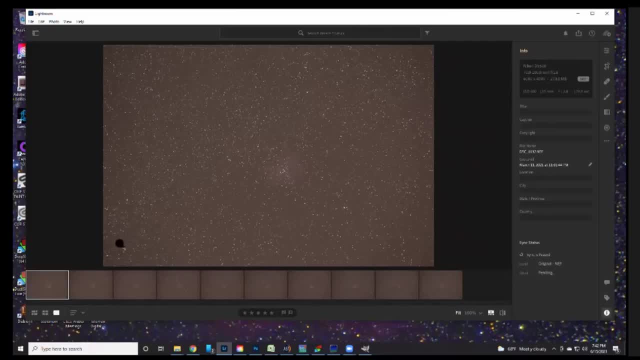 i'll cover when we get to that point. but um so, light room is, uh, again of a basic product. I do like it for at least reviewing and I will edit like even my vacation photos in it, because it allows me to do enough with that And I do even take my vacation type. 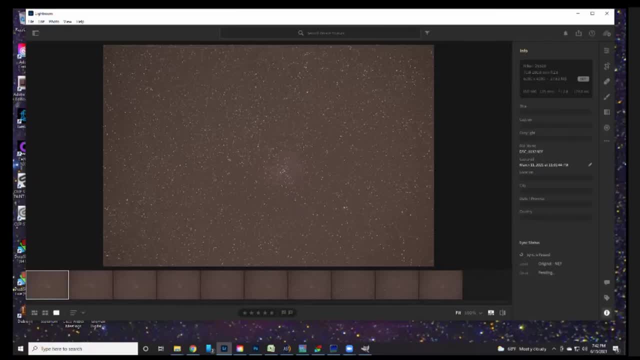 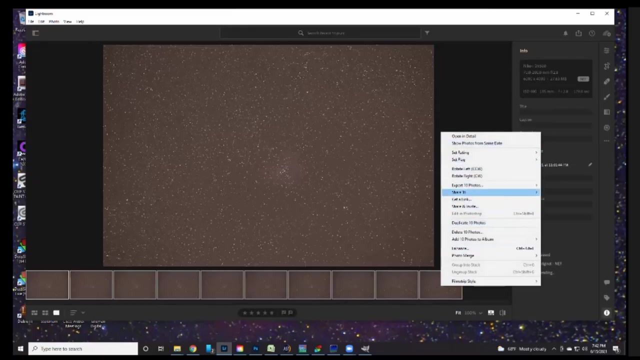 photos in raw format because, again, you can do so much more manipulation of it. So if someone's image their face is in shadow, you can actually go in and set it up so that you can lighten up that image. So for now I'm just going to get rid of that And in here it says: oops, delete 10. 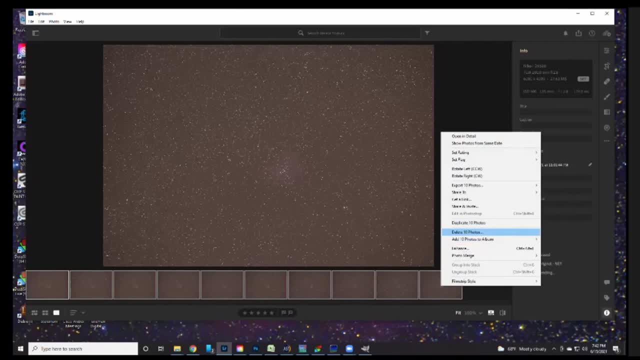 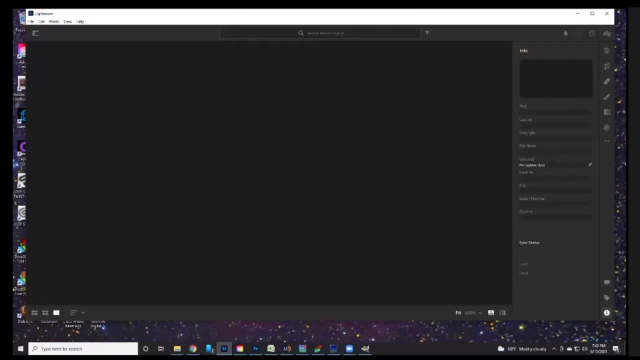 photos. It's not really deleting it from the file or from the hard drive, It's just deleting it from the application. So that's Lightroom. I don't know if anybody has questions about that, but that's the basic original tool I use to just do my image review And typically after I've notated. 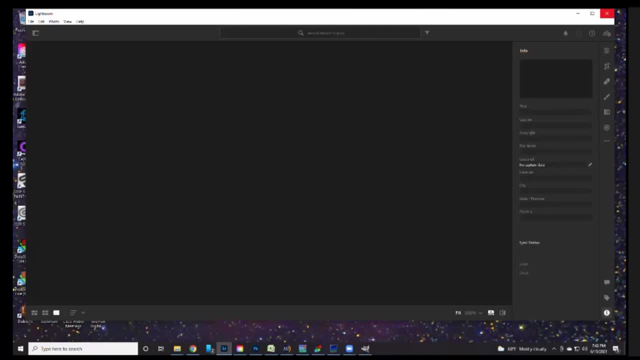 all that information. I can just tap right there and I can becomes a professional. So I can and make sure I have my best images. I move on to the next step, now one. the next step is: do I have one image? that's only really the only good image I have. 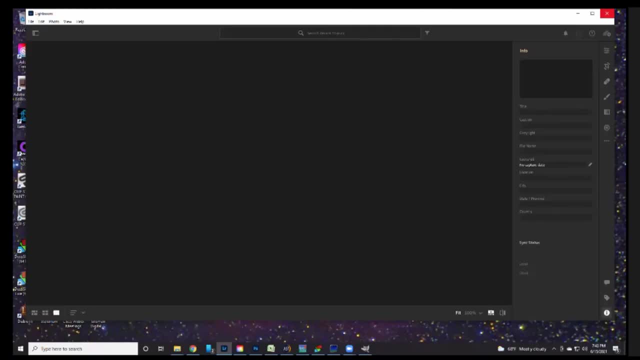 and am I going to just process a single image, which is possible, or do I have enough images, like in this case? I had ten images and I'm gonna actually stack them, so there isn't too much of a difference between if it's a single image or multiple, except for with multiple you're going to do. is that a? 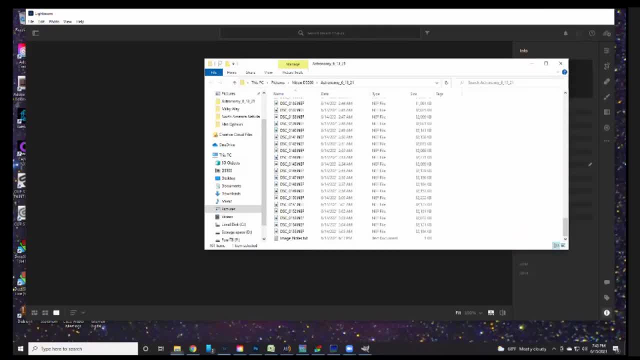 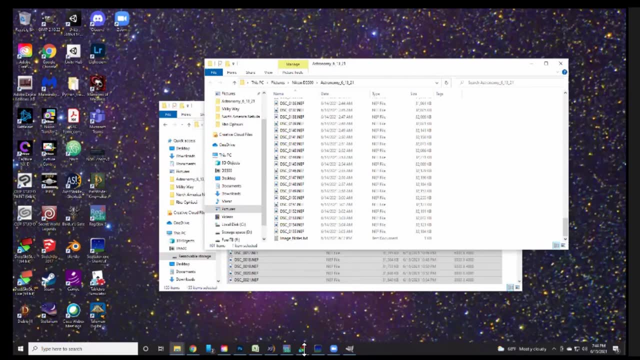 stacking step. so that's what we're going to go to next, since we have ten and ten images there of that target, we're going to go back, go to a stacking process. so the most commonly used stacking tool that most people use is called deep sky stacker, and that's this product, but there's another one out there that's. 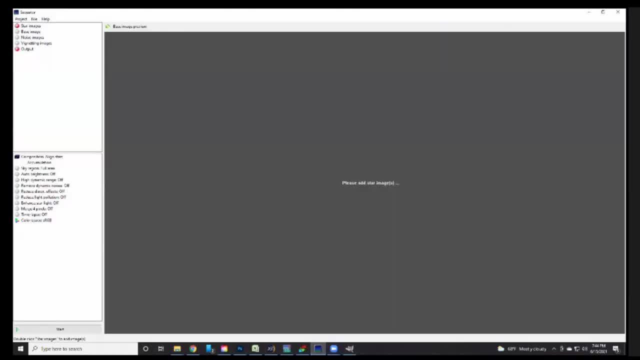 becoming more and more popular, which is called sequitur, which is this product. they all work very, very similarly. I don't know if I have necessarily a preference one over the other. I use deep sky stacker, it seems, more often than I do a second tour, or if I'm saying that right, hopefully I 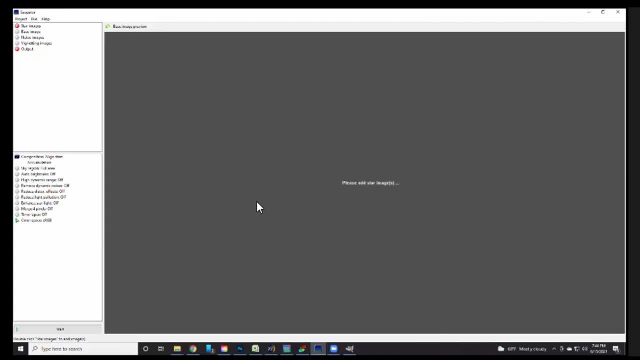 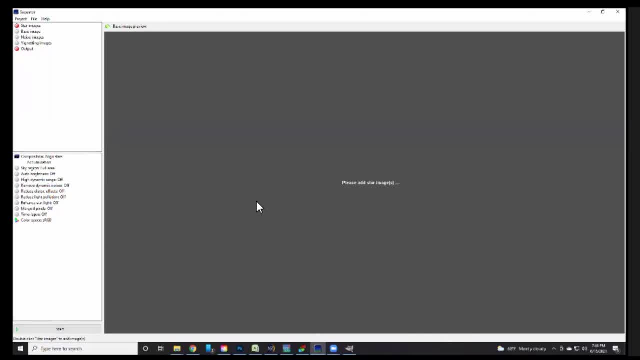 to be a little bit wider and your image is going to be a little bit wider and more colorful. but it sometimes it over does it and almost posterizes your image, which makes it look kind of fakie. so it depends on your, your starting image. if it's really dark I might go to sequitur and use that. but 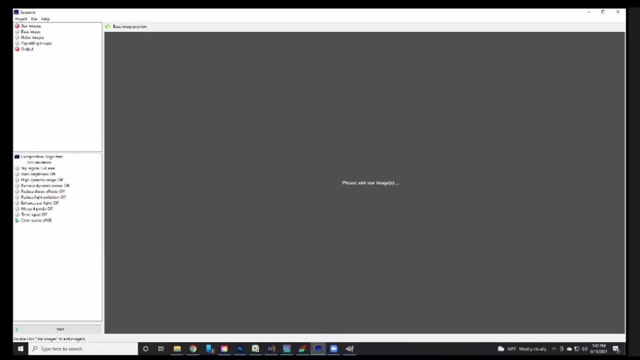 for the most part I use deep sky stacker, so I'm not gonna use secret or tonight, so I'm gonna close that. just know that there's other stacking products out there and and you can even manually do do stacking in something like Photoshop. but there's tools. Why do it the hard way, Unless? 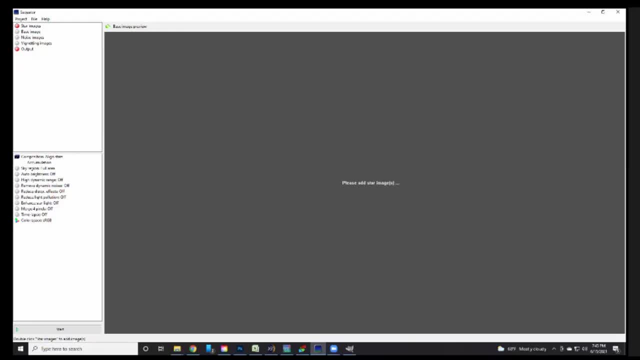 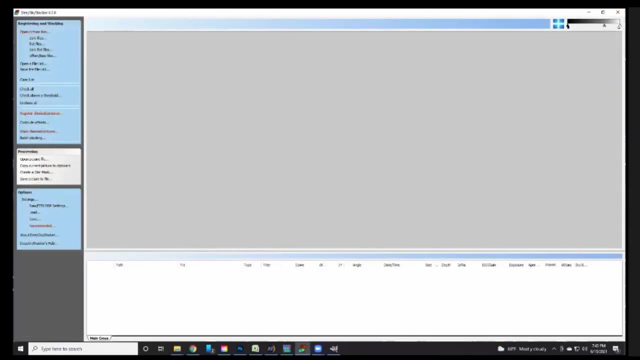 you're just so married to Photoshop that you want to do it there, but I don't see why There's pre-made tools for you to do that. One thing I did forget to mention is if we're talking about deep sky objects, which is what we were just looking at in Lightroom, versus a moon image. 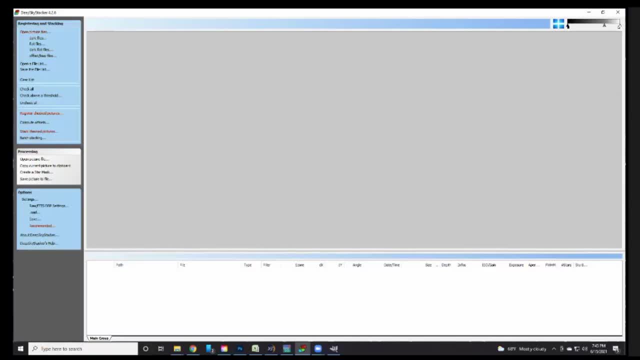 The moon is so big and bright that you may have a movie. Processing the moon is quite a bit different, because you actually have surface detail on the moon that you're going to want to align properly. There's two products that are typically used for that. I'm going to show you that before. 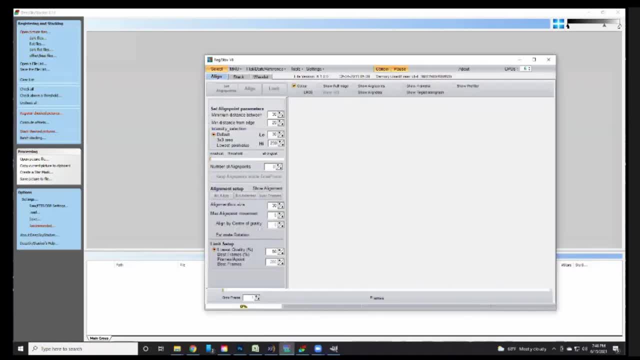 I get into the guts of Deep Sky Stacker. There's one product here which is pretty popular, which is Registax. You can use Registax to process single moon images. There's a whole process in this. I'm not 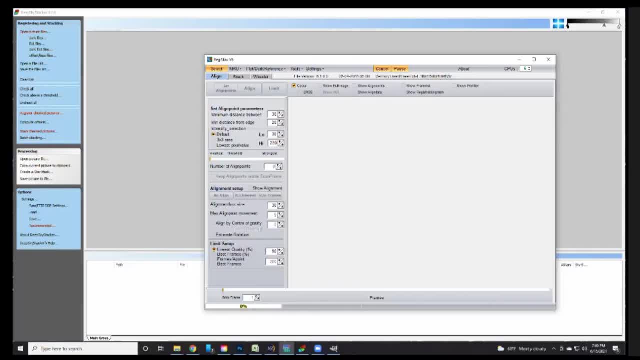 going to cover that tonight, because I don't do that much lunar imaging. I do some, but not very often. You could have a whole presentation on Registax alone. As a matter of fact, there are plenty of YouTube videos out there on how to use. 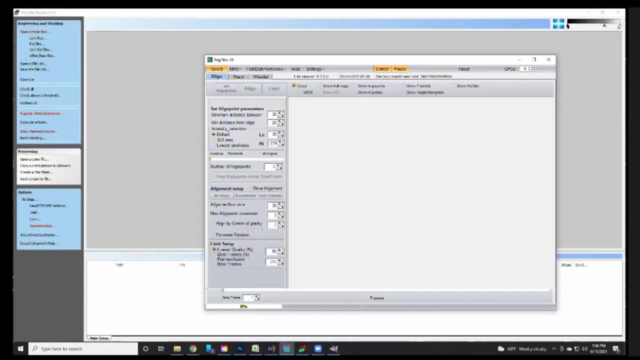 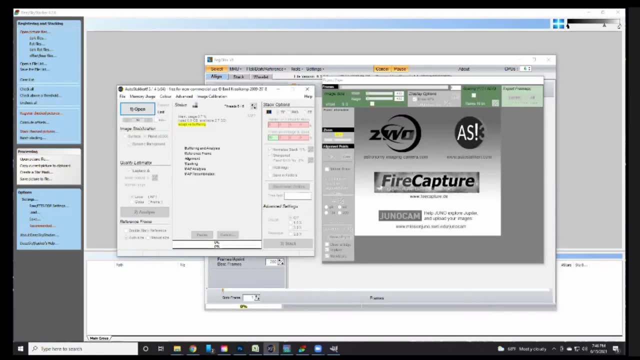 Registax is one of them. There's another product called Autostacker. Again, these can either take a single image or a movie that you've created. Actually, I should say either an ABI, My camera, my Nikon takes moviesmov. None of these products like mov, so I end up having to find some kind. of a converter that converts it to a movie. I don't know if you've seen that. I don't know if you've seen that. I don't think you've seen that. I don't think you've seen that. These are pretty. 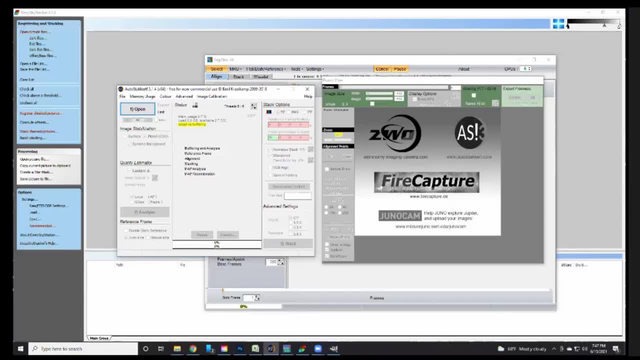 common. So you can actually use that to make something like a little electronic object or a little sort of mini object. It's pretty simple. You can also convert it into either an MPEG, MPG or ABI, So that's typically what these two products will accept. but you can use them to do lunar stacking. 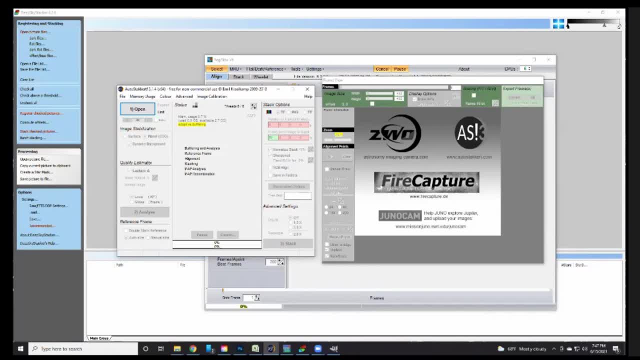 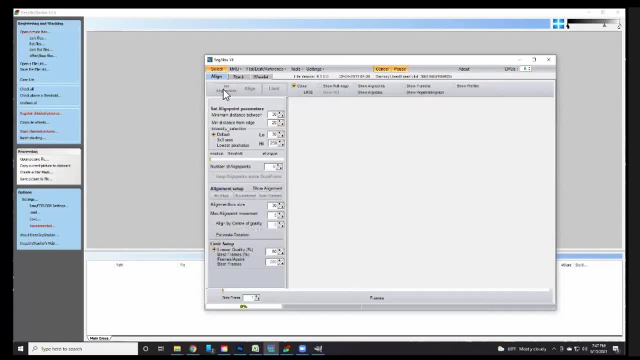 You can also use it for planets because, again, you have some. depending on your image, you may have some enough surface detail where you could use these two products to do that. So there's some basic processes you do go through. it's just- uh, i'll kind of real quickly go over the registax process, which is you would 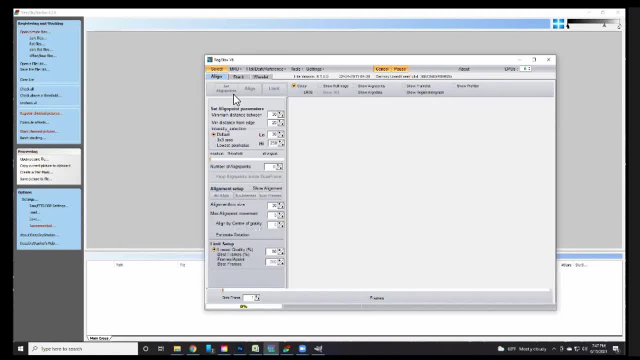 load up your image into this again. i'm not going to do this. you would load up your image, you would go through the set of line points which basically puts targets on your image, and then it'll assume that that bit of that set of pixels that that target encompasses is going to be the same on. 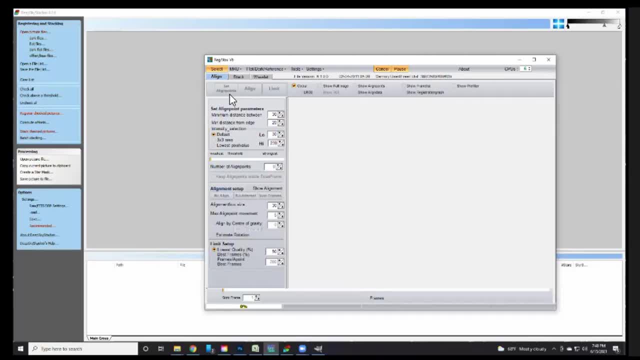 each of your images and therefore i'll try to find those pixels and align them. so that's what set alignment points. so first of all, it figures out where to put alignments, or you can manually do it if you think you are good enough with your mouse and targeting, or if you have some quite. 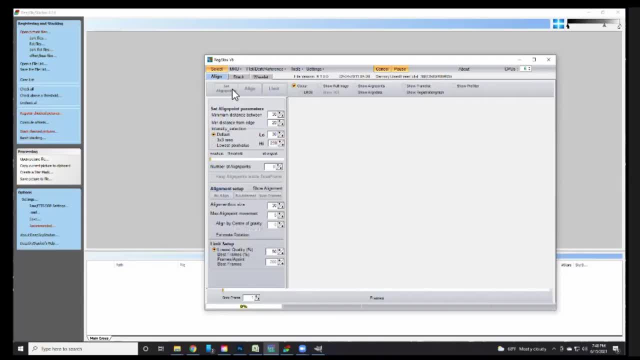 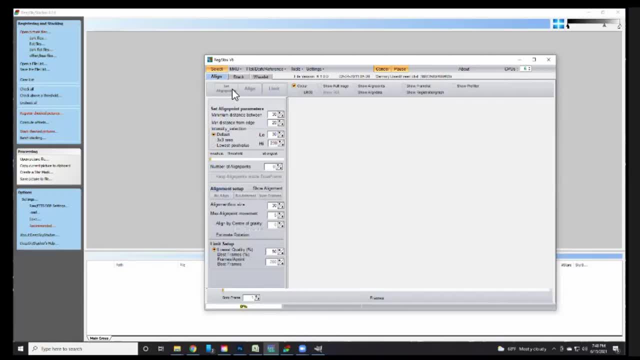 the great red spot. you can see it in your image and you want to target it and make sure that that specifically gets aligned so you can manually set alignment points. then you would do a line, you would click the next button, which is a line, and there's a whole bunch of these sliders and 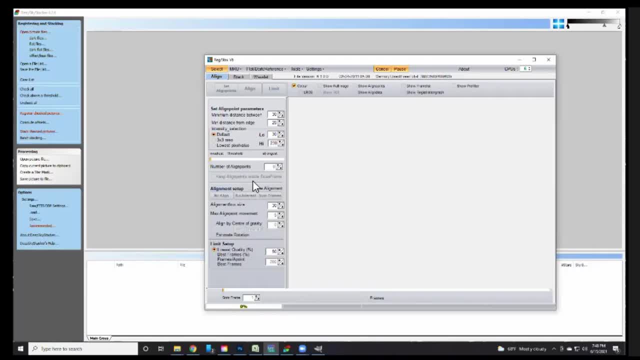 adjustments that you can do to try to help make this go smoother. uh, so, again, again. there's a whole video that you could do on just running register stacks, because there are a lot of different elements to it, so you can set limits on what you know if you how, how, like your contrast. 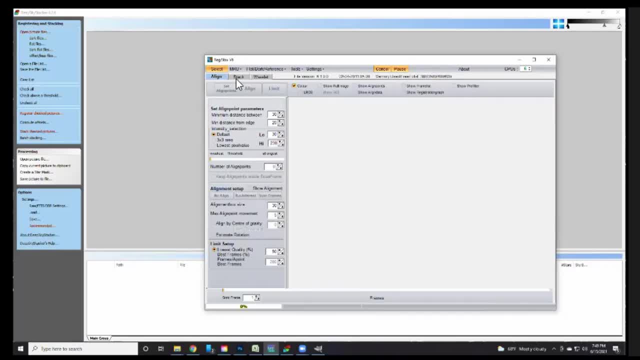 and stuff like that. again, there's a whole bunch of stuff. then it switches to stack and it does more stacking and gives you more options like: should i do a gamma figure? it's pretty complicated. and then there's the final step, which is wavelet, which allows you to. 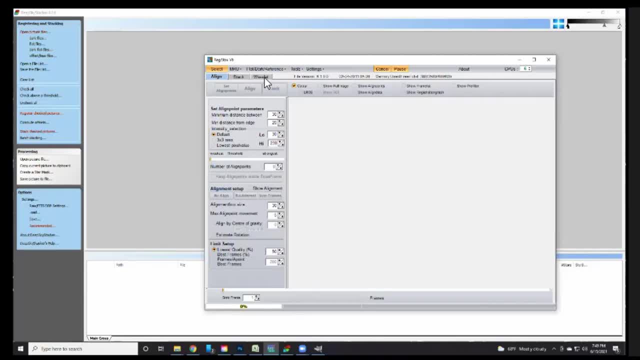 to again make finer adjustments to the uh. now you can adjust the rgb if there, if you need to. although like something with the moon, it's pretty much black and white almost uh and uh depend on your image and uh, but it with something like saturn or jupiter. there is a little bit of cover. 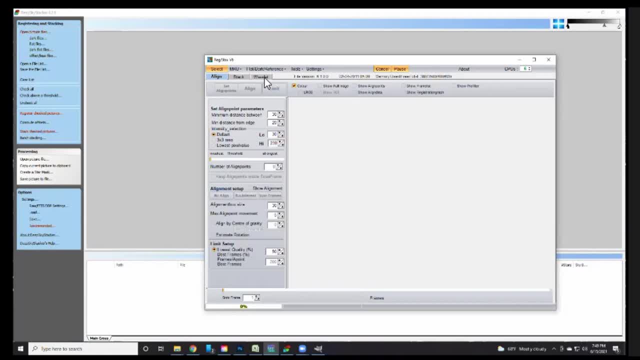 color, excuse me, uh, to your image. so then you can adjust your rgb levels on the wavelet side and do other things like trying to to remedy grain and stuff like that. so, uh, that's again a real, real quick version of how register works and how doing planetary or lunar imaging works. i'm not going 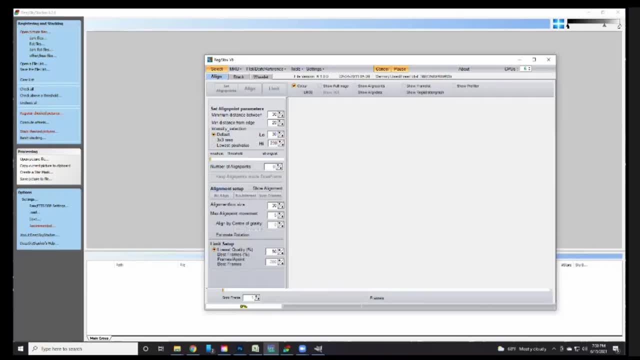 to cover that again tonight. um, that may be for someone else to cover, or uh, if you want, go out to youtube and i'm sure you can find a video on how to use register or auto stacker. hopefully, if anybody does have questions about that, they can post those. 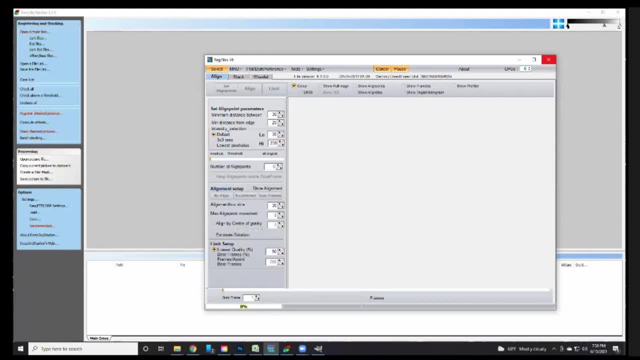 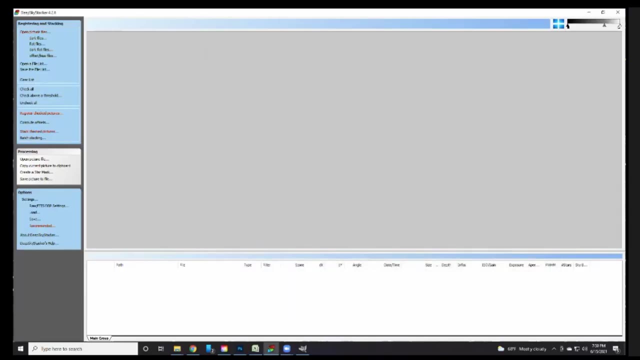 into again either facebook or onto the yahoo groups. uh, all right, so unless i get interrupted, i didn't sound like it with questions. i'm going to move on to deep sky stacker. go ahead. we actually do have a question about deep sky stacker itself. okay, wondering how it compares using the uh. 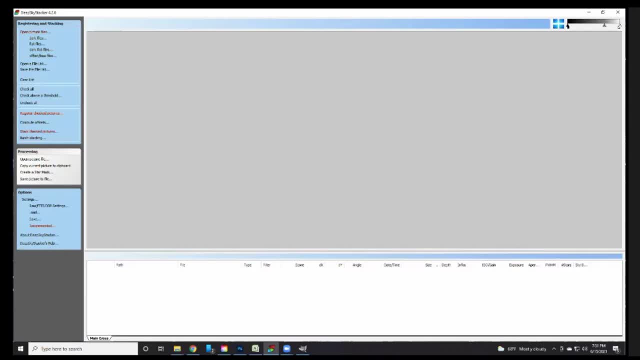 automatic stacking that photoshop can do too, if you've done that before. so if you, you used either or both of them. to compare i uh, yeah, so i have not used photoshop's auto stacking. uh, my understanding is that it it does a pretty good job. uh, it didn't used to and i've done a manual. uh, stack in photoshop, uh, so i. 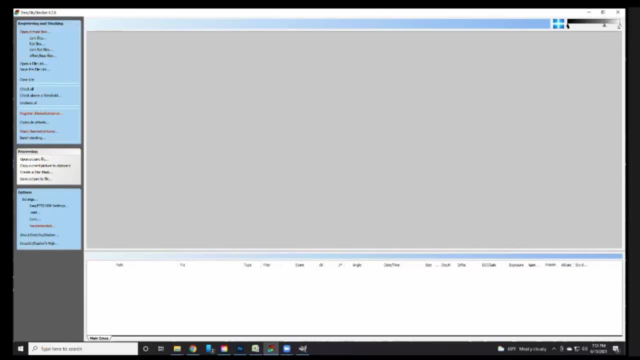 don't know if i can directly answer that, and i know i'm pretty intimately familiar with deep sky stacker, at least more so than the process of photoshop, even though i'm going to end up using photoshop, uh, tonight. i i don't know if it's how good it is, i, i don't know, so i'm afraid i can't. 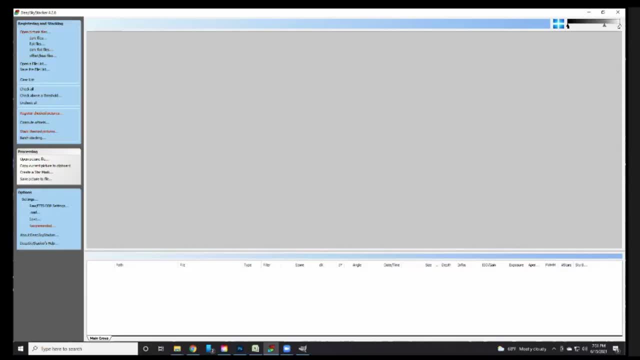 really answer that, but i know deep sky stacker works really well and, uh, for the most part, meets my needs. i know that's not much of an answer, but hopefully that that addresses that question. all right, so, uh, any, if there's no other questions on that, we'll move on to deep sky stacker, uh and most of the targets. like i said, uh, that i do. 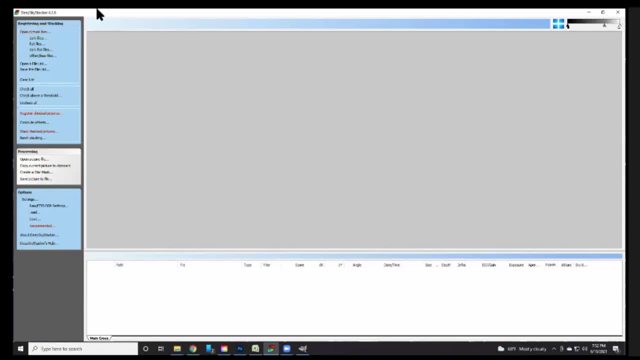 shoot are deep sky objects. i enjoy going after those. so what we're going to do, you pretty much go down this left side of deep sky stacker to do your image processing there's. there's several options on there, but one of the things that i've found that's really important is that you 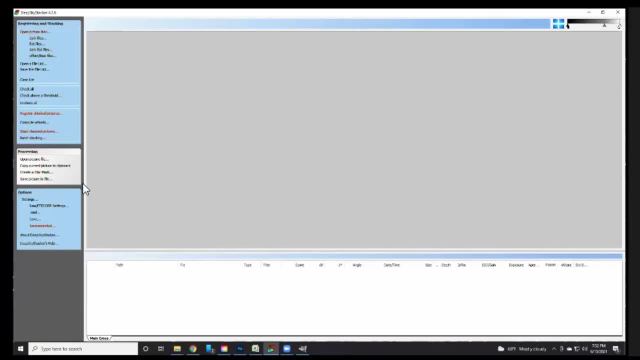 can do at least a little pre-processing, uh, and something like lightroom to increase your contrast or exposure, increase that to make it lighter. but most people say, no, just go ahead and take it straight out of the raw file, don't bother. uh, it's, you know, you're gonna introduce you. 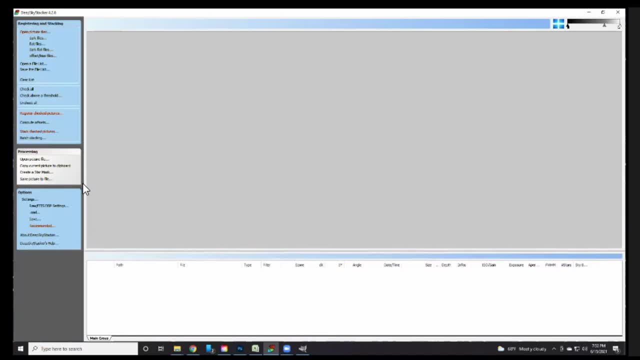 you have the chance, if you do a pre-process before deep side stacker, of introducing uh artifacts from whatever your pre-processing is. So but if your image, like I mentioned earlier, if your histogram is way to the left, you may need to do that just to get deep sky stacker. 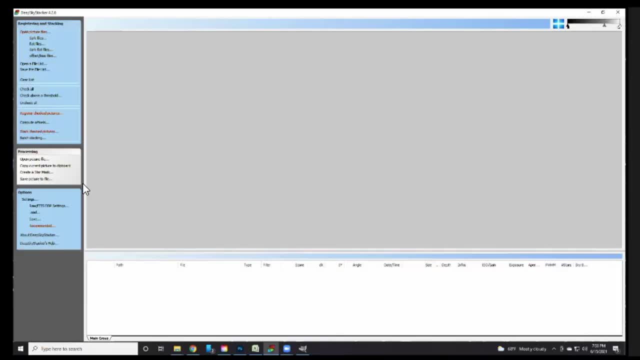 to work properly. So it's kind of choose your battle type thing, whether you think your image is good enough to have deep sky stacker work or if you think you need to do a little pre-processing to make it work. So and take the risk of introducing potential artifacts. 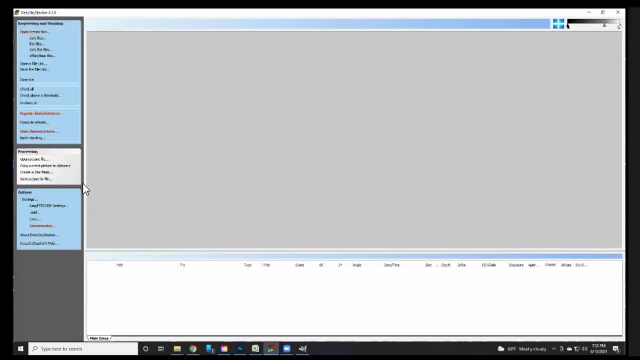 that may or may not, that probably are not really in the image. So in general I work with my raw files right out of the camera. I don't do pre-processing- I used to- but I think what I've come to find is: 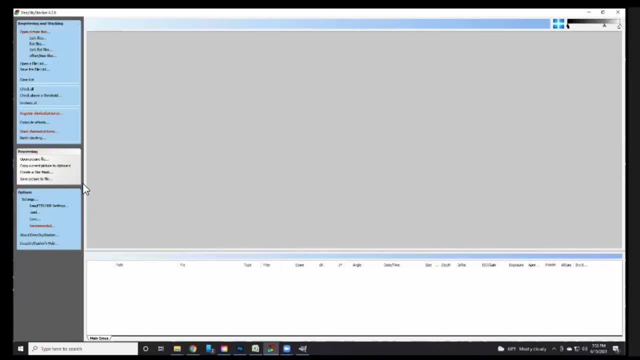 if you're looking for an image that has higher amount of contrast, you're gonna probably find out that it's better to start with a dark image coming out of deep sky stacker and then handle it in your photo editing product. You'll have a much richer image, I think. in my opinion, 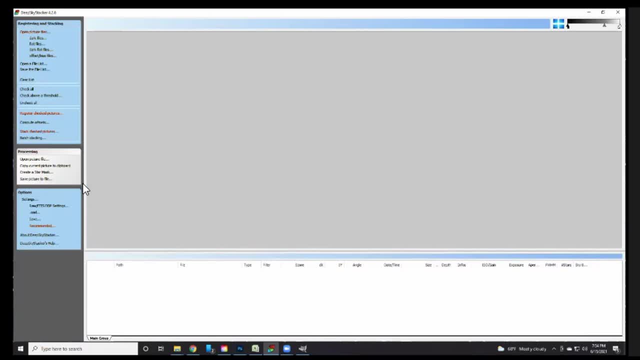 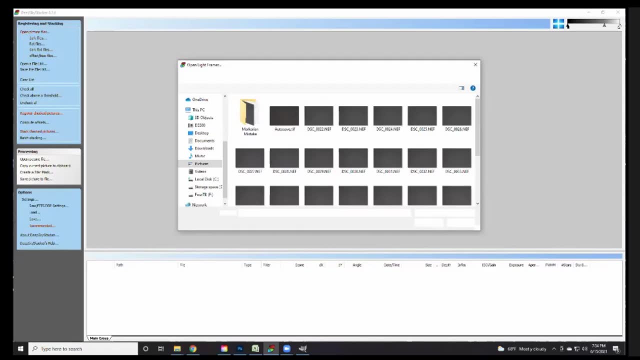 So again, whatever for whatever that's worth. So what I do is again: normally I just work down this left side fairly quickly. We're gonna again do this relatively quickly tonight. I'm going to go back to the picture. that other folder took this earlier this year, um on 311, and we're going to work on the rosette. 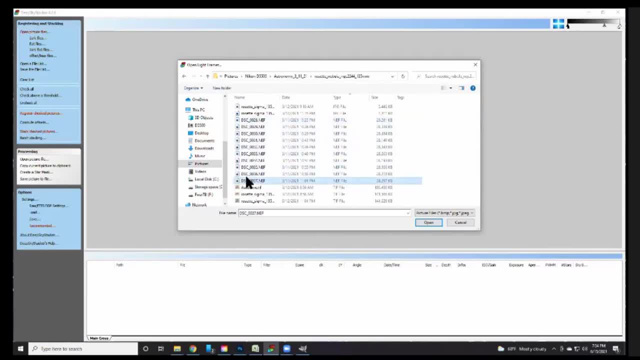 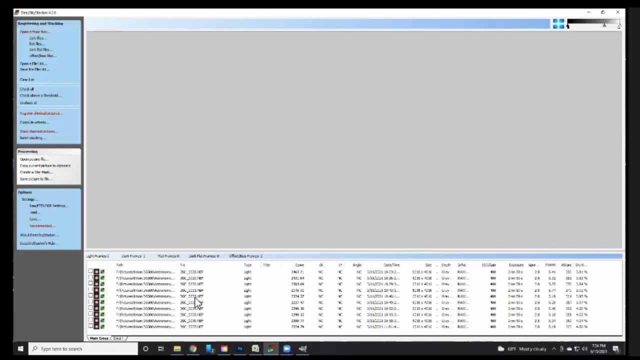 nebula is the image that we're going to do and stand my fingers on the right key, so we're going to select all our images now. uh, one of the odd things about deep sky stacker is it doesn't automatically check. it says, oh, these are your light frames, but i'm not going to automatically. 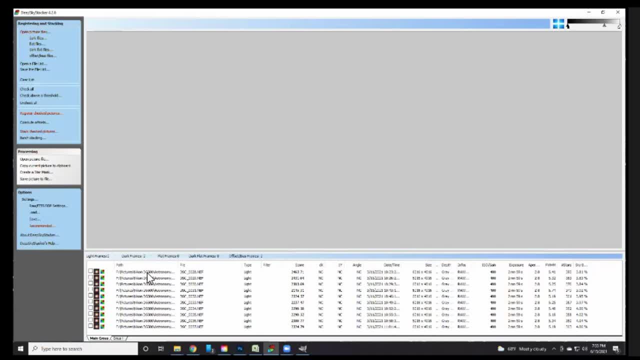 check them and you might wonder why. and that's because, uh, i've already done what's called score these images and if you notice this column right here, it's called score and it's basically telling you how good is the image going to be for the stacking process and it basically does a rating. 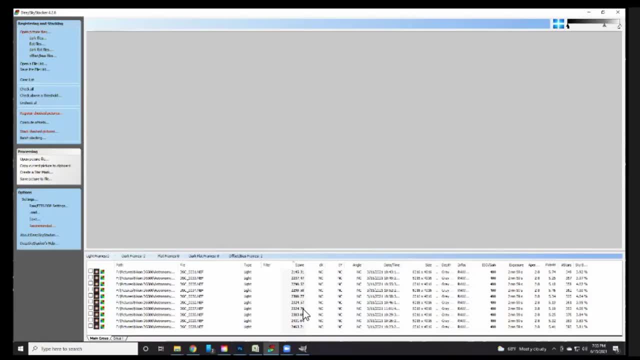 based on how many stars it can find if the stars are in similar alignment. so i've already kind of done that, because i've already done an image review and gotten rid of anything that has really either clouds moving through it or something like that, because that can introduce. 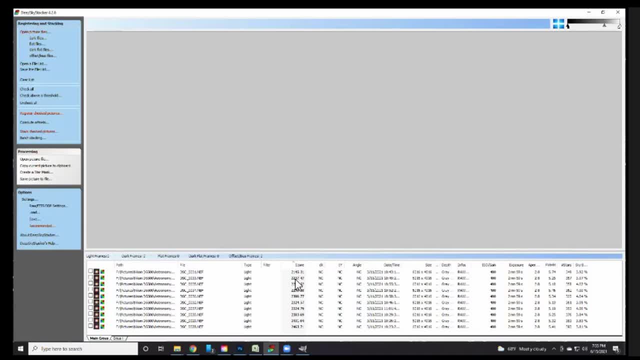 additional data you don't want. so, if you notice, most of these scores are already pretty similar, right? so, uh, they don't automatically check all these images because maybe you don't want to use them all, so you do have to come down here and say: check all so that you can do the next steps. 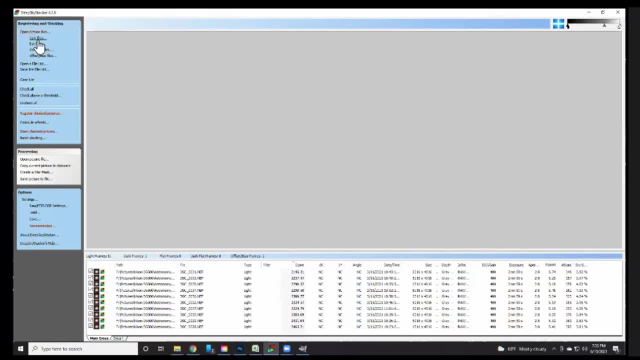 now one thing: people argue both ways that should you do dark files, should you do flat files, should you do dark flat files, which is interesting one, and the offset, uh, uh one. so should you do your lights, i mean your darks, your bias frames? uh, some people say yes, some people say no. uh, depending on what camera you're. 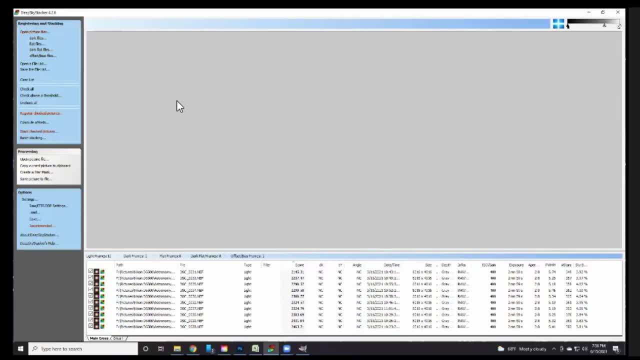 using and and the quality of your images. so if your camera has a lot of- uh, let's say, hot pixels in it, you're probably going to want to do a your darks at the very least, because that'll show up in those darks and deep sky stacker will know those are hot pixels and it will try to eliminate those. 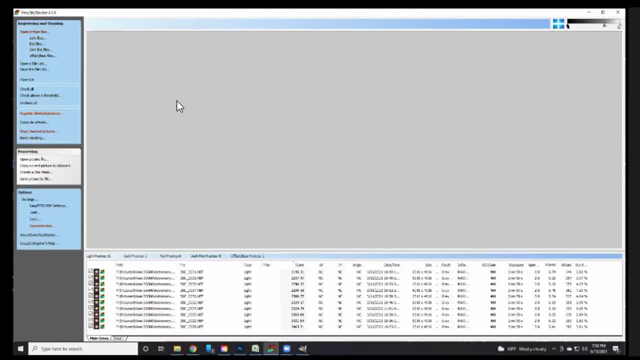 but if you're like me and get, i got lucky- my my, actually, i think. just recently i just started noticing the first hot pixel on my, on my sensor, uh, so i am going to probably start having to do a lot more of the darks than i used to, because i didn't. i had a nice clean sensor. 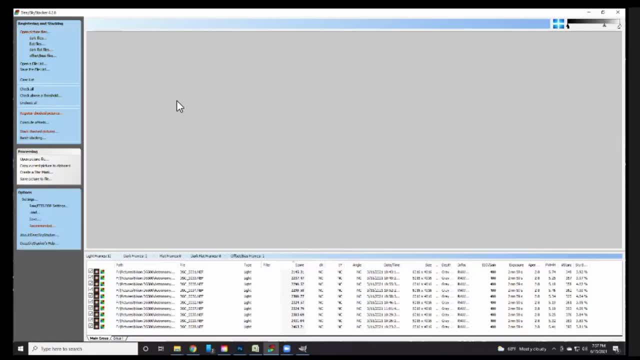 and i had my image, never really had hot pixels, uh, so i didn't didn't always do darks and i, but i i have done them, but i don't always do them, uh, but i might start having to uh. so now flats, uh this, if i would have done, uh, my flats, which are basically just, uh, so darks are. let me go back to dark for a 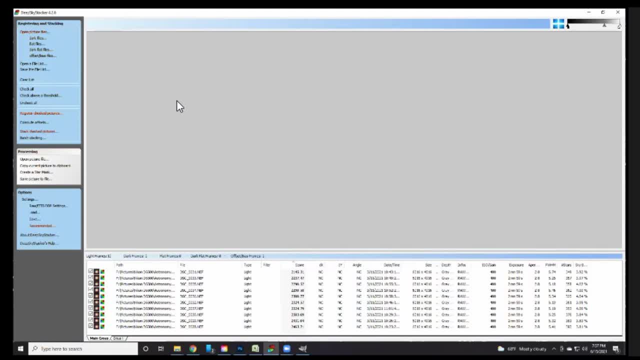 second darks are taken, uh, with your- let's say your- lens cap on and at the same temperature, preferably at for the same amount of time, with the same exposure. everything basically the same as your, your light frames. you want it to be all the same. so if you're taking two minute subs and you got, 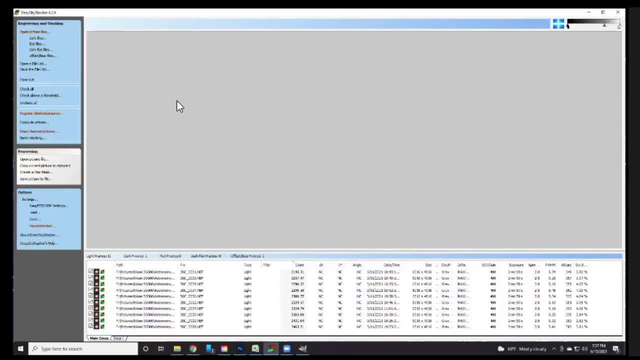 10, that's 20 minutes. so you should take- you know you should take- at least five to ten darks of the same, so you're going to potentially, you know, increase the time that you're. you're photographing nothing, basically you're photographing the lens cap, so you're going to increase your time. 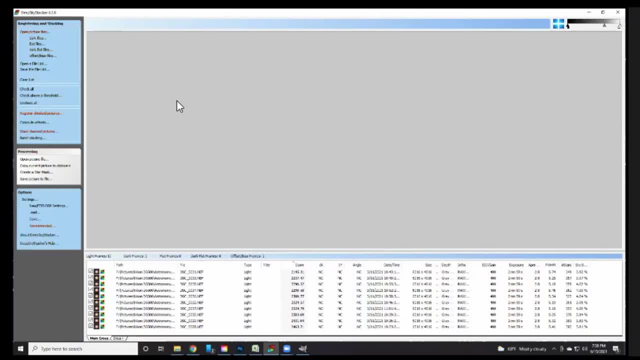 wasted on one particular target, especially if you're switching your iso or your exposure length uh during the night for your for each target you try to shoot in one night, and some people don't even shoot multiple targets in one night. i do, i i try uh mainly because 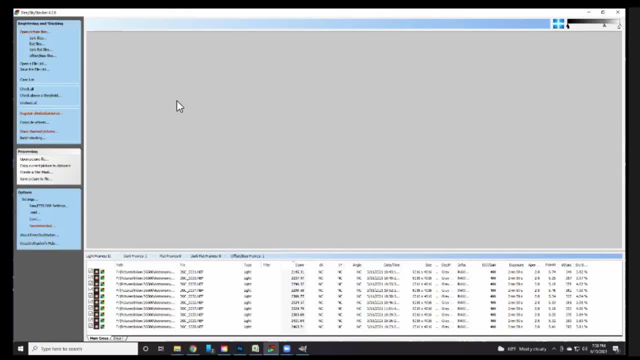 you know, as things move up in the sky, you'll get a better contrast up in the top of the sky versus down in the horizon, where it's going to have light pollution and what other you know atmospheric interference, so, um, anyway, so that takes the dark sticker the the hot pixel. 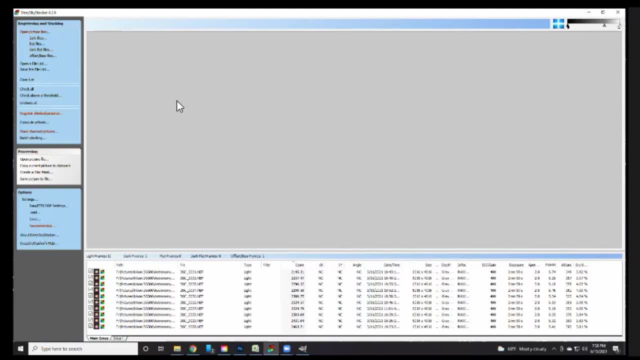 type issue or amp glow or something like that the the flats take care of. what i just had happen to me the last time i went out was i had a big old dust spot that was clearly evident on my images. uh, the flats would have, uh, made it clear. now the flats are basically you're holding a white object. 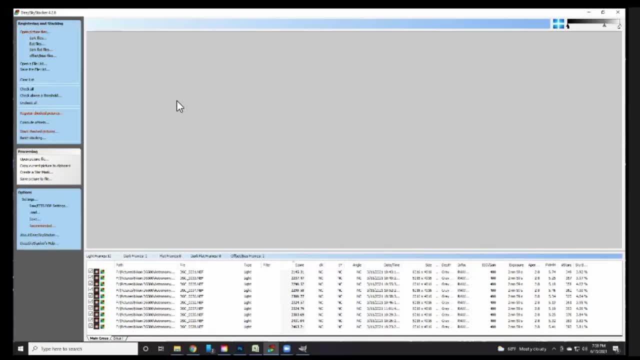 something that's nice and flat, that doesn't have any shadows being cast from it, and, uh, what most people do is like just a simple white t-shirt over a flashlight, in front of their, in front of their object, not in their lens. and they do. you don't have to take the same length. 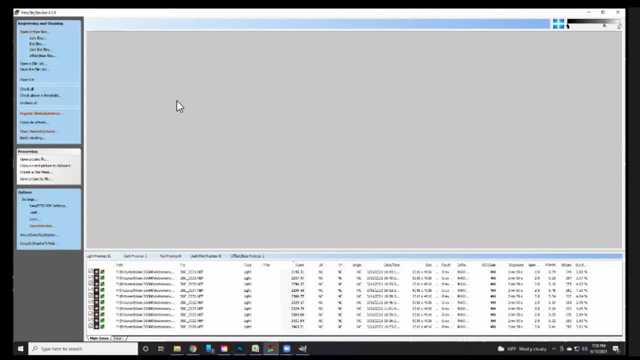 of time you can take it as fast as you can. you should take at least 10 to 20 of those and and that'll help with something like dust spots. so, but again, do i do that all the time? obviously not, since i did see that i had a dust spot on my last images i took. so 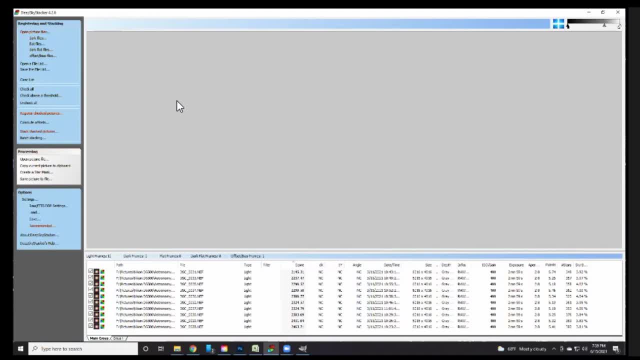 so in this case i'm not going to do it again. i'm going to show you some of the steps further on. but you can load up your dark files and you can load flat files in there and try to enrich your image in the in the uh for your final outcome to be better, so you can look at the images in in deep. 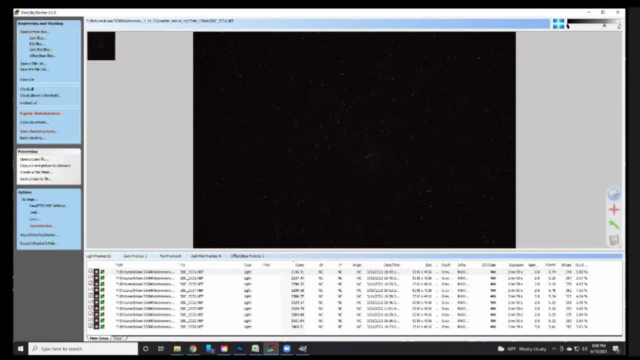 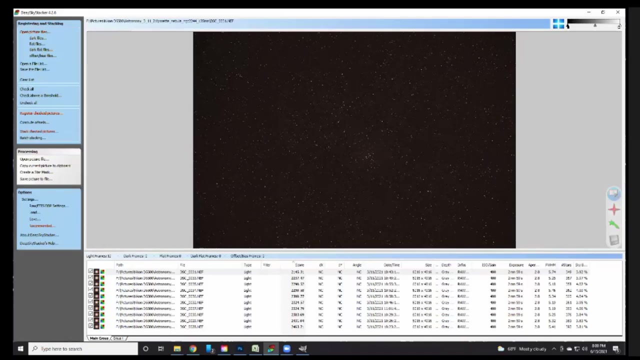 and you can see, uh, some stars here, quite a few stars in this image, and you can even adjust the slider up here in the upper right hand corner to try to expose more images or objects in your image. so you can adjust it, you can. that's the mid-tone that i just adjusted. so this is the darks, the mid-tone, and then the light. so 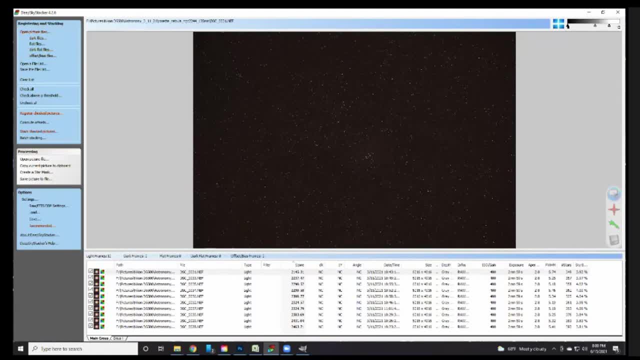 you can uh, drag those around to try to get more stars to show up, or more even your, your target might show up if you adjust it. so, but you can see my target really well. if you know what you're looking for, it's right there. but uh, again, you can't really see it. but uh, just now. 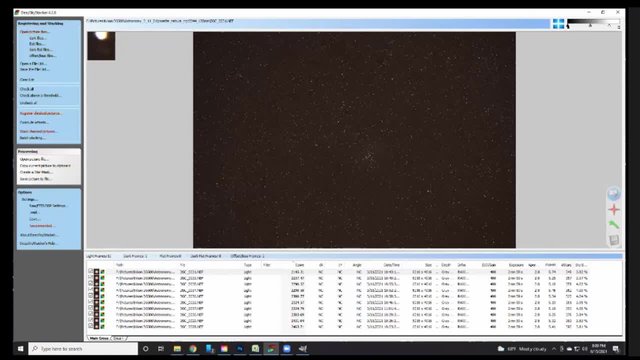 this isn't actually editing the image, it's just for display uh and uh. if you have a specific target in in the image, let's say, if i was looking at the uh orion nebula in here, you could put it over the the inner stars of the. 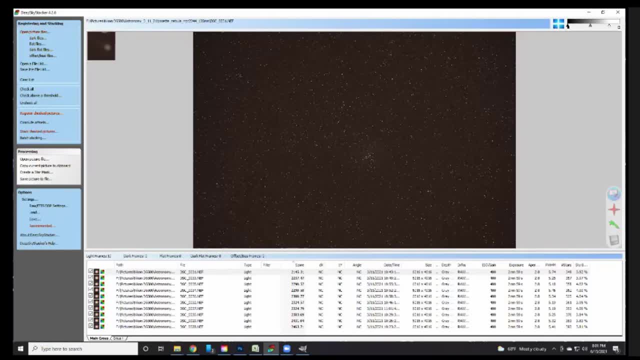 uh, the orion nebula, and you can then see how sharp your stars are. so you can see in the upper left hand corner, over oops, over here, well, as it moves around, as i'm doing that, but you can see that my stars are at least nice and round, which is a good thing, and you want them to be as pinpoint. 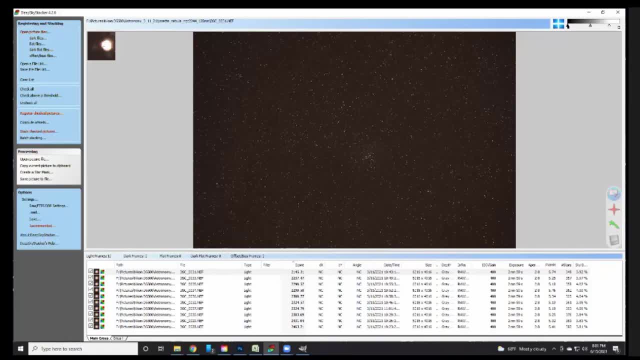 as possible and nice and round, not bloated. they're a little misshapen, you can see, but uh, so that's a good thing. uh, again, this allows you just to review your images. it's another way to do it. uh, now i i said i use lightroom to record image information about it, but it's also in our deep sky, stacker, you. 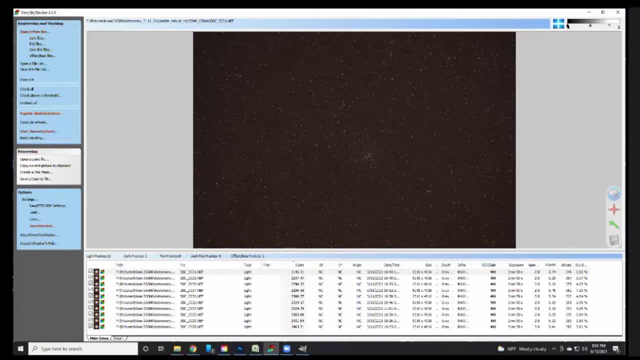 can see. the iso was at 400, they were three minute exposures, the aperture was 2.8 and, uh, i forget what these ones are. so, uh, if, if you're. if you don't remember what it was in lightroom, you can also find it here in deep sky stacker. i just always do it when i'm reviewing my images, that's just. 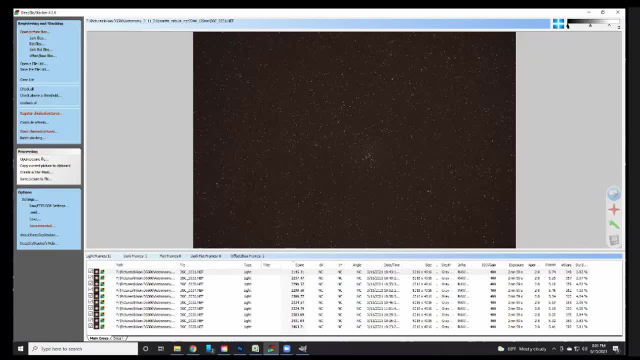 part of my work process and it does show you the pixel size of the image, so you can see this pretty big. uh, six thousand pixels by four thousand pixels, that's gonna be a pretty big image, uh, let's see. so that's pretty much that, um, so i've already checked all like i. 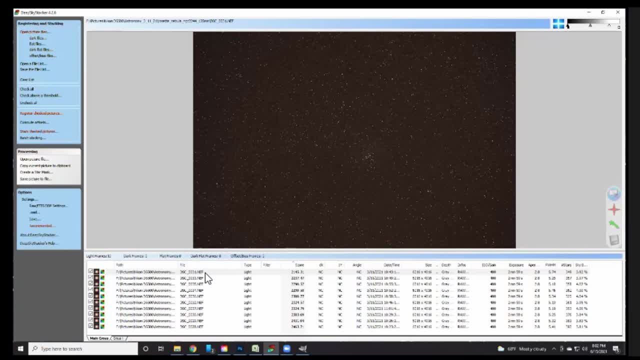 mentioned. so the next step is to: uh, oh, i forgot one thing, so let's say you find one. uh, this is something i just recently learned myself, so, uh, there's still stuff i'm sure i can learn about deep sky stacker. i haven't tried a lot of the really nitty gritty stuff, uh, so 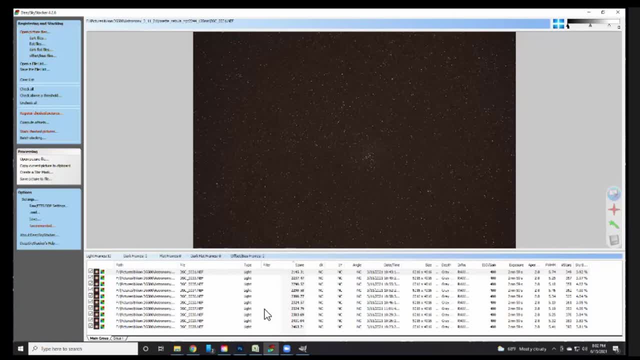 just but just saying this kind of going back to that question about, uh, the photoshop stacking. you don't have to do a lot of tweaking to deep sky stacker, it's already pretty much set. so that's why pretty much why i use it. i don't have to want to know what all these other things are. 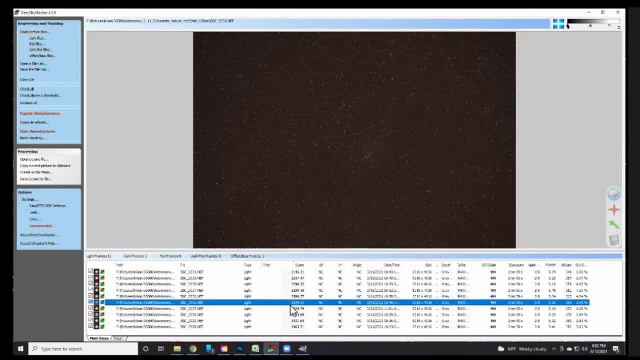 that i'll show you here in a second are. i don't want to have to know. i wanted to use it and get my image, uh, to the point where i like it. so, uh, one of the things you can do is, let's say, you have a. 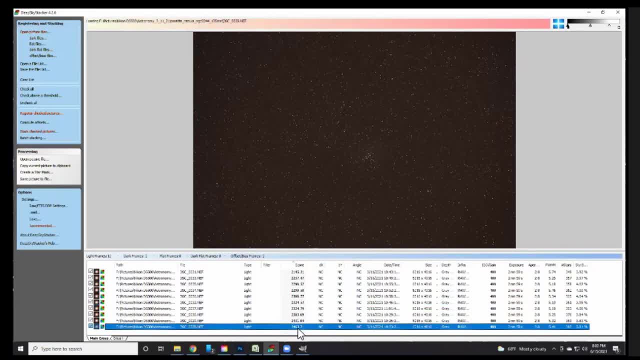 one that has a really nice high score like this: 2463. that's pretty high score. of all these looks like the highest and if you right click on it you can click and say: use this as the reference frame. so it's saying: try to align everything based. 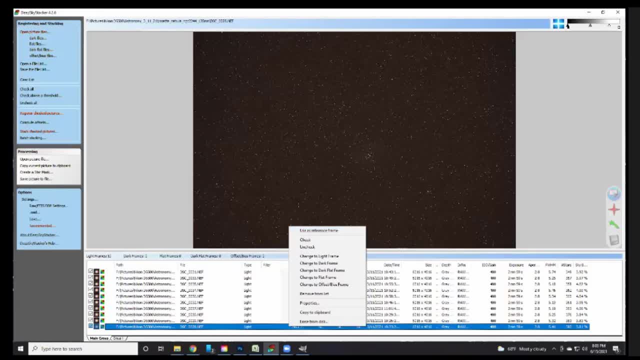 on this image. so that's the new thing i just found recently, and, uh, i don't always do that. i actually, like i said, i just learned it, so i didn't always do it. it seems to figure it out on its own, so, again one of those things i don't want to have to worry about, but learning that new. 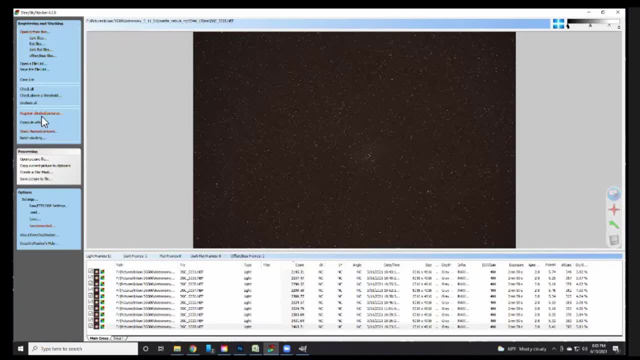 hopefully it's going to improve my image. so the next step as you go down the left side over here on the menus here is register, and this is kind of the the real crux of deep sky stacker. so what you're gonna when you bring up the setting again, these are those settings i don't like to. 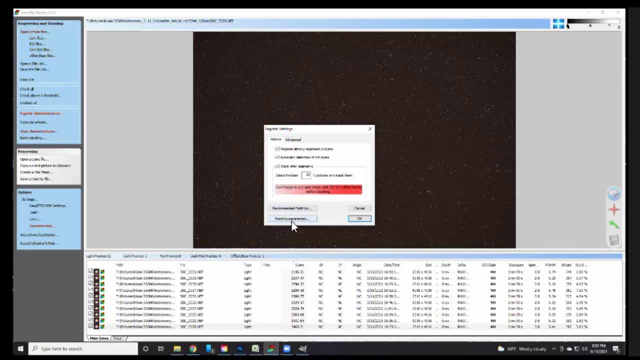 have to tweak if i don't have to. i usually use the recommended settings and i don't hardly tweak anything in here. the only thing i might tweak is if i have a few images, like i do in this case. i only have 10 images. i might switch this to use all of them, so i'll set it to 100. so i want to use all. don't. 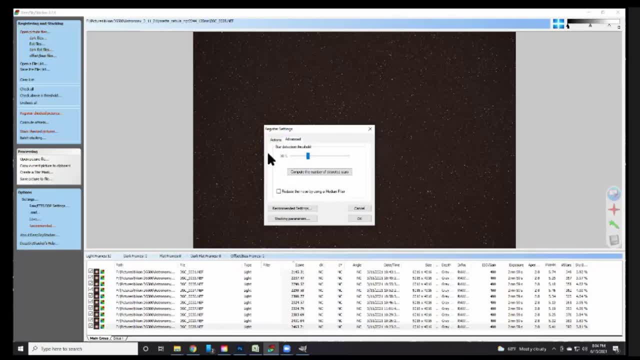 throw any out, and i already know they look pretty good. uh, so just to kind of show you though, there's: if you bring up the recommended settings, anything in green is what's already been selected for you. uh, that's um. again, i do, i use the recommended settings, i'm. 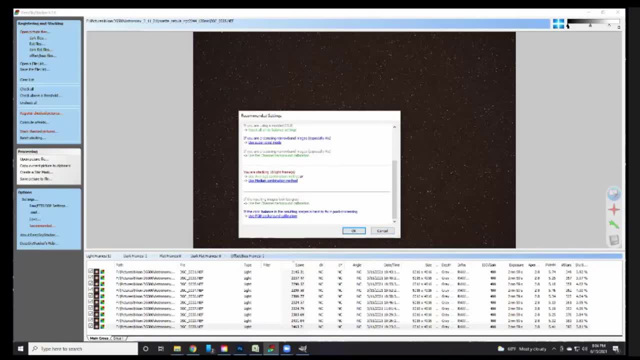 i've never really played with them. so there are other things. if you still aren't getting your image to come out the way you want, maybe if you tweak around with these it'll- it'll improve the image. same thing with the stacking parameters. uh again, standard mode for me always seems to work. 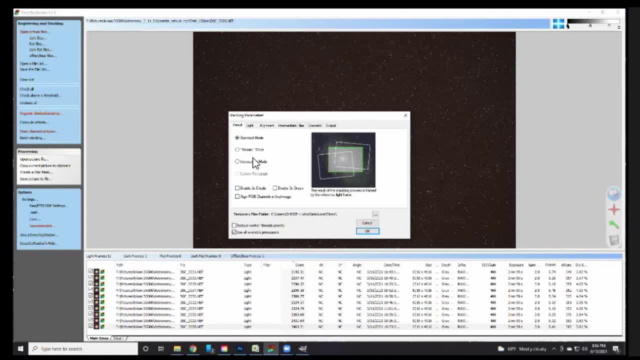 again the reason i review my images: to make sure that the images are almost identical. the stars that are in one image are in the same stars in the other image. i don't want to have to mess with this, this, this, these tabs, so you can just go through these and and just these. but again, i usually leave it as this: the. 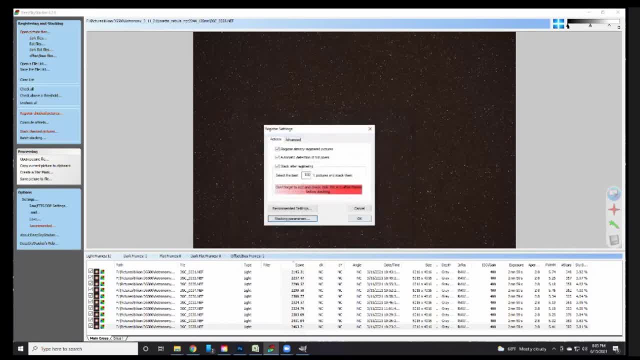 basics. i don't want to have to do extra work, and uh. so, uh, you can, if you've already registered them, like i have. like i said, i already had these scored. uh, you can uncheck this box so it won't do that step again, but for now i'll leave it. uh, just to show you how, how fast this works, and then. 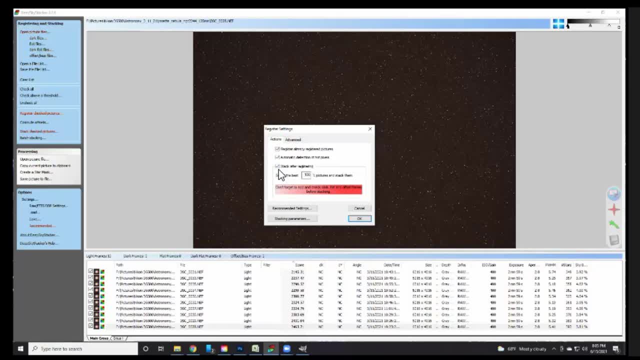 the next thing, of course, is stack after registration. if you don't want to stack right away and you just want to get the, the scores, uncheck that, then run this and it'll do this- uh, registration and not stack, and then let you go back and choose which ones you do and 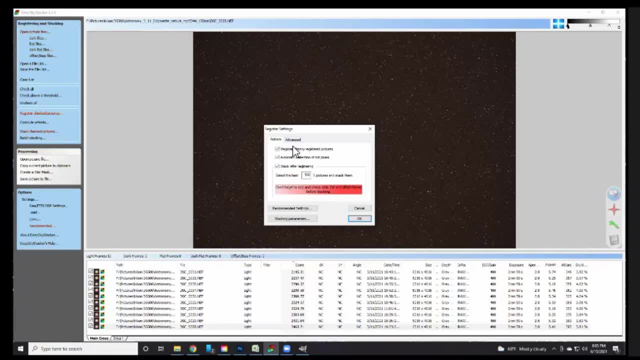 don't want to use, so for now, again, i'm going to leave it on. uh, go to the advanced tab though. this, this step you definitely need to do right away, and one of the first things you're going to do is this button right here. so you're going to say: compute the number of detected starts, and then you're going to also come up on results and check them right on advanced. 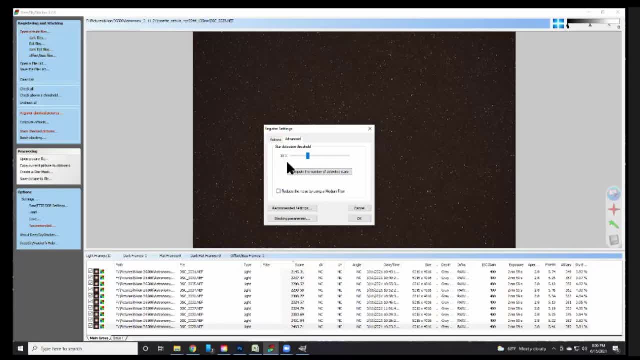 Now I have the threshold- the star detection threshold- set to 30% at this point, and that was probably because it was whatever I used on the last time I ran Deep Sky Stacker. So you can adjust this and what you're going to do is click that button and it's going to sit there and take that reference frame, whatever reference frame you selected, and try to find stars. And in this case it came up with 2,103 stars. Well, do I need that high of a number? Some people would say, yes, you want that many. For me, I'm like I don't need that many. 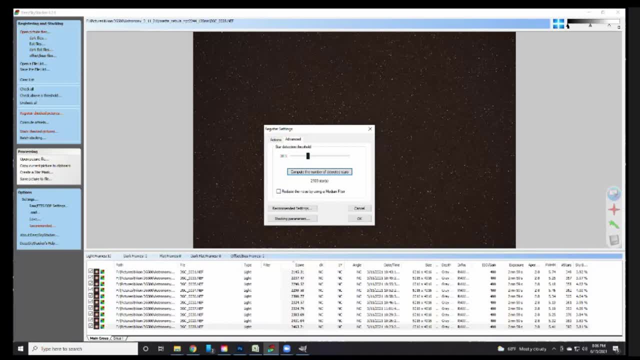 I think my picture's already pretty much aligned. So what I will do then is say: let's increase the fidelity of that alignment by increasing this slider, this threshold, to make sure I'm not picking any hot pixels, Because out of that 2,100 stars, maybe it was a hot pixel that you said: oh yeah, it's in that image, it's in that next image and that next image, and it's not really a star. 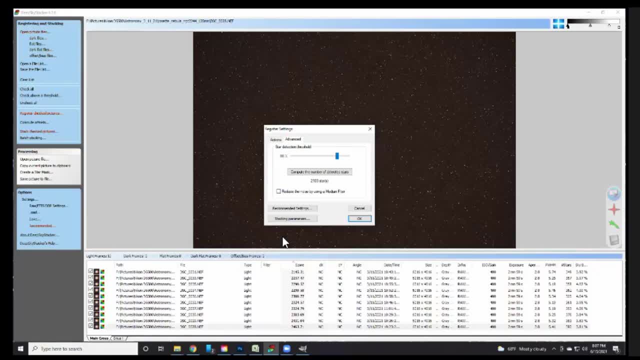 It's a hot pixel, So I increase it so that it says: no, I need to be more distinct about what exactly is a star. So then I click this again and you'll see that this count should go down quite a bit, although there are a lot of stars in this image. So 631.. I didn't even, I didn't even go higher. I'm like: no, you know what, I'm going to go all the way up to 90. I usually do whole, you know, 10 by 10.. And you can see it does it pretty quick. Now it's just doing one image right, So it's not doing all of them yet. So 400. Okay, So I typically go with at least, at the very least, 140, 150 stars. 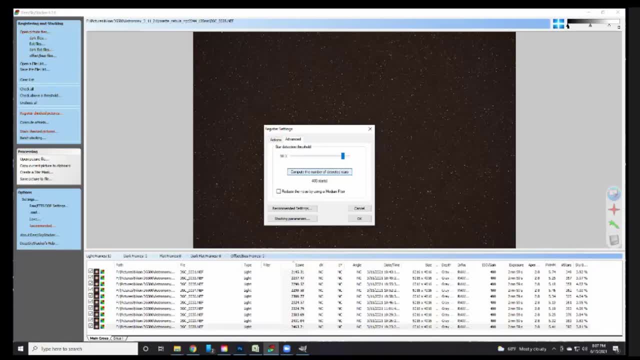 If it can at least find that many, that's pretty good. So there are certain images or certain targets that don't have a lot of stars around them. like some of the galaxies, You won't have a lot of stars right around them. 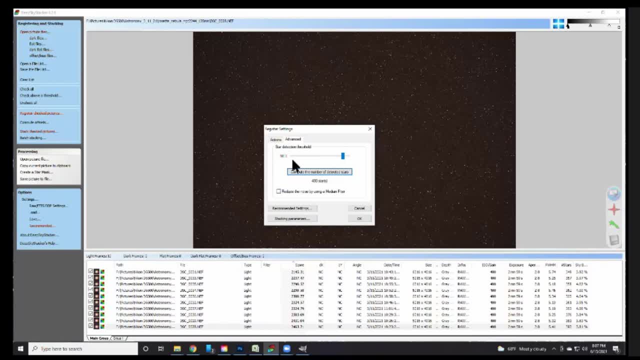 A lot of the circumpolar targets are like that. So what you will potentially do is end up all the way down here at 10%, And that's fine as long as you get around 140 stars. that it will use to do alignment. 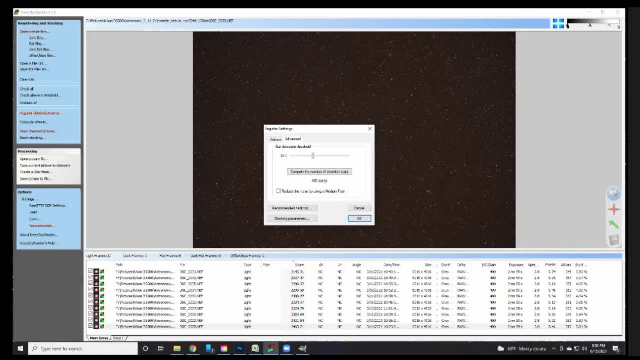 That's what you're aiming for. So, but in this case, you know, 90% is going to work. 400 stars, sure, Okay, that's fine. And so At that point, at this point, I would say, okay, I'm ready to, I'm ready to run DeepSky Sacker to start stacking these images. 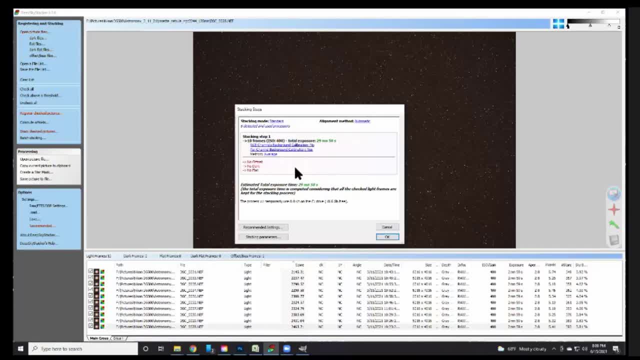 And it just when you click okay, it brings it up. It says, by the way, you're not using any offset, no darks, no flats. So it does remind you And again it suggests that you should use those. but it you know, it's up to you. 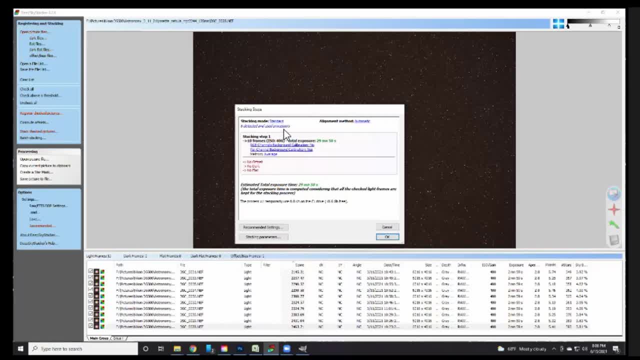 And what your quality of your images are. And again, stacking mode standard. I pretty much never change that Alignment method, automatic, sure, Again, I hardly ever change these things. My goal is every time I go out imaging is to get images good enough where I don't have to worry about changing all these settings to make something out of nothing. 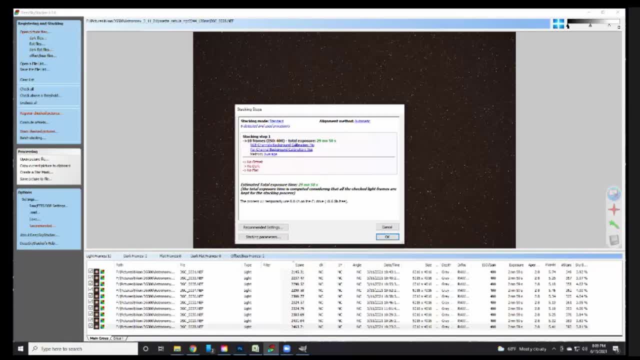 And I think that's probably every astrophotographer's goal. So one other thing it does tell you at this point. it tells you how many frames you're going to use- 10 frames- And it's going to end up with 29 minutes and 50 seconds worth of integration. 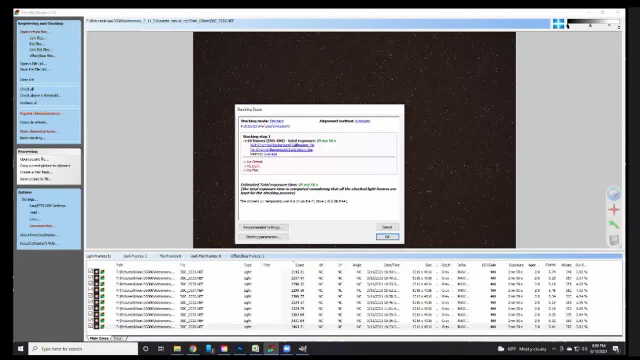 So what I've done is take 10 three-minute exposures, and what it's going to turn this into is one exposure that's 30-minute long exposure. So that is your goal. So it would be as if you had left your taken one image and left your lens, your sensor, exposed for 30 minutes, whatever sensor you may have. 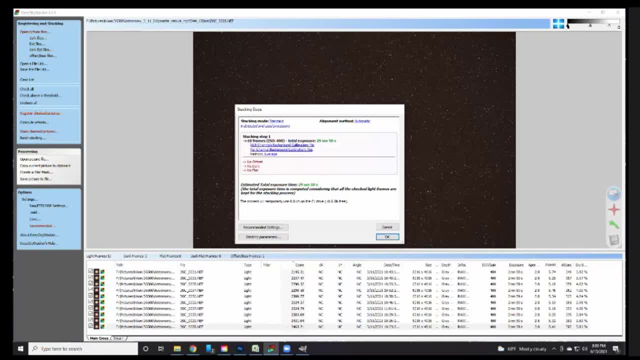 So that's the whole idea of stacking And again, some of the Some of the best things you get out of stacking is getting rid of grain out of your images that can come from having a high ISO. So if you're going after those deeps, those galaxies that I mentioned earlier, a lot of them, if you want to get a lot of detail, you may end up having to increase your ISO pretty high. 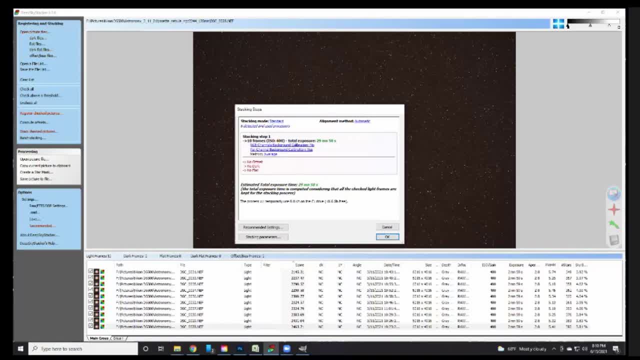 That can end up leading to grain in your images. So but if you do stacking, that should eliminate that or help eliminate it. I won't I'm not going to say it totally does, but it should help eliminate that. The other reason is that if you have light pollution again stacking, it's going to realize you know, hey, the dark background should be dark. 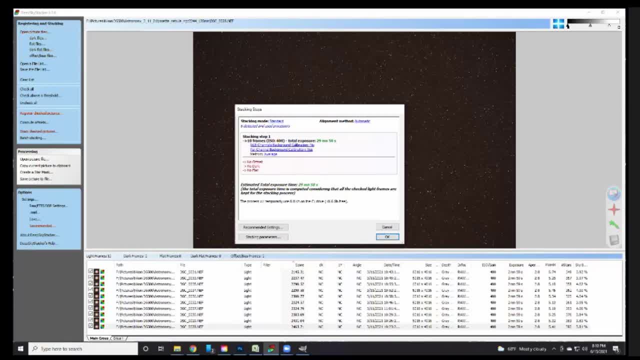 And it realizes that. So and again, it'll help create that darker background. And hopefully you don't over Contrast your images. Some people do. I know a lot of people who usually started out in the hobby do that. I used to do it. 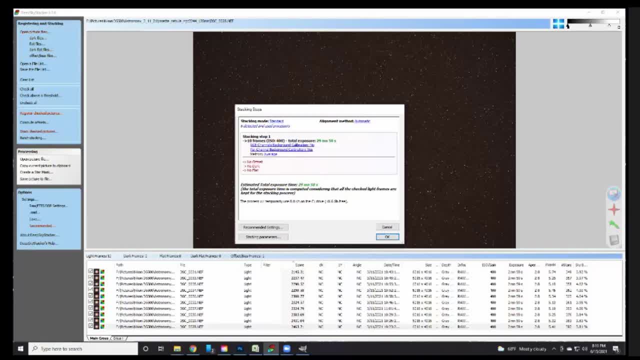 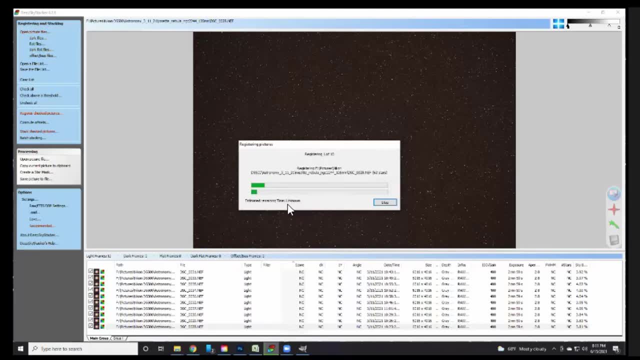 But actually you lose a lot of image when you go too high in contrast. So something we'll get to here in a little bit. So I'm going to go ahead and click OK at this point And we'll see. It does give you an estimate on how long it will take. 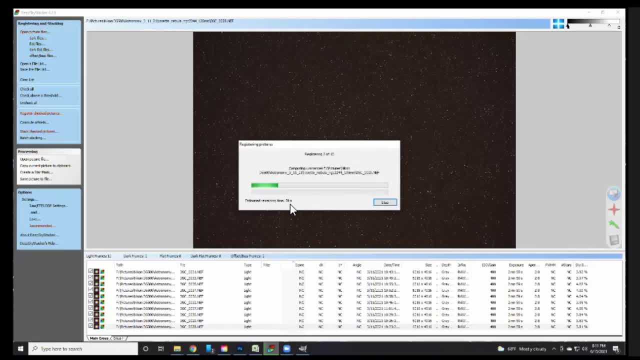 So right now it's registering all those images So this might take a little bit. So it's going to take a minute. it thinks Now, if I know, it's flashing up here pretty quick, but it did say it's using six core processors. 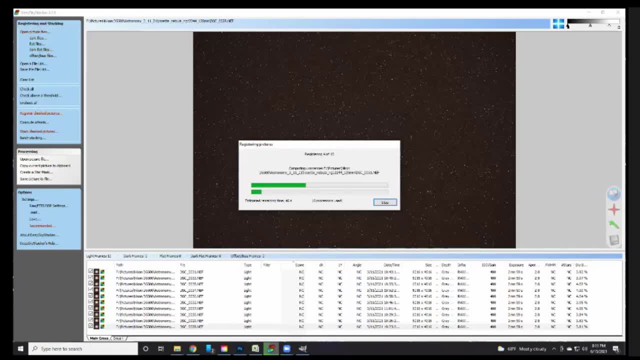 So this is a little bit of time for me to lecture about your hardware that you're using the software on. I've got a pretty beefy computer. It does have a lot of processors on it. It's got a decent amount of memory. 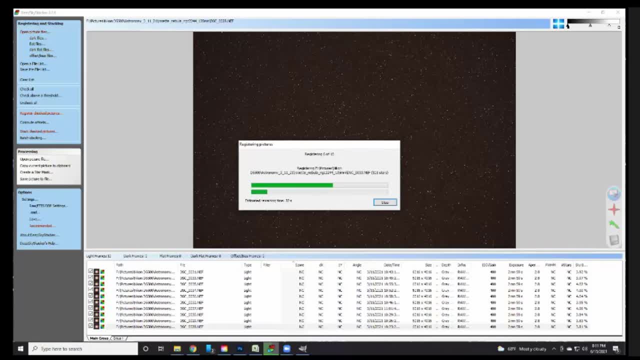 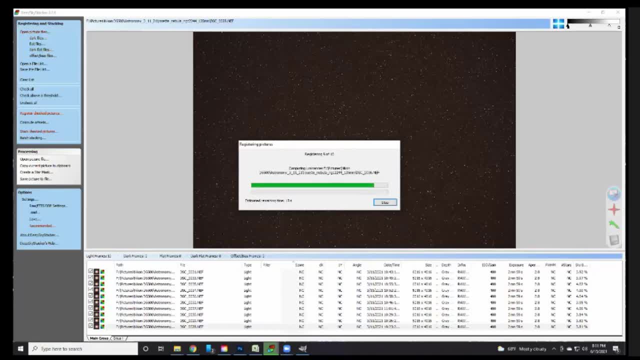 So you have to be mindful of whatever disk you're program prey on. It knows it points to the right place where you got some to do some of this ever the I've got a pretty decent video card in my system, so it it should handle this stuff. 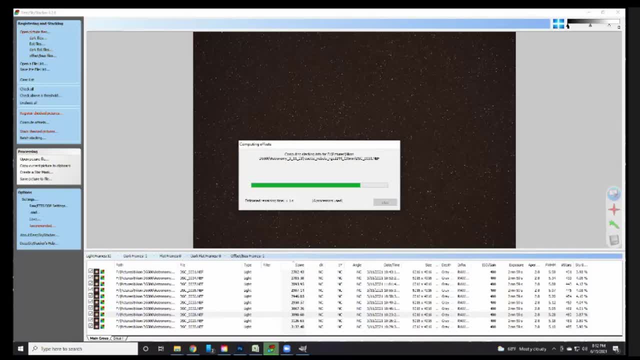 I mean, I've got a lot of apps running right now. so what I'm trying to say is the beefier your system is, the better it's gonna be able to handle these processes. So it takes only a minute to do those registrations. 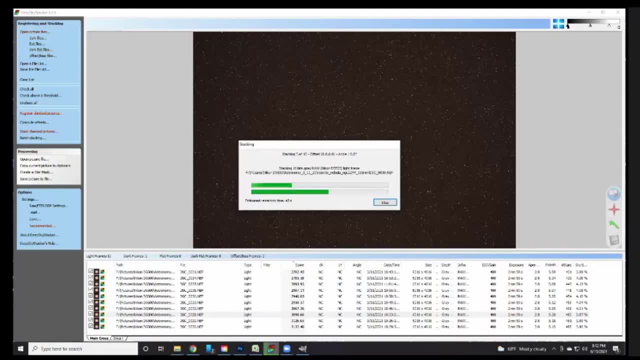 and now it's gonna take another minute to do the actual stacking and realize that's only with 10 images and with a pretty beefy system. So the other day I had over 300, almost 300 images of one target and I stacked and that took even on my heftier system here. 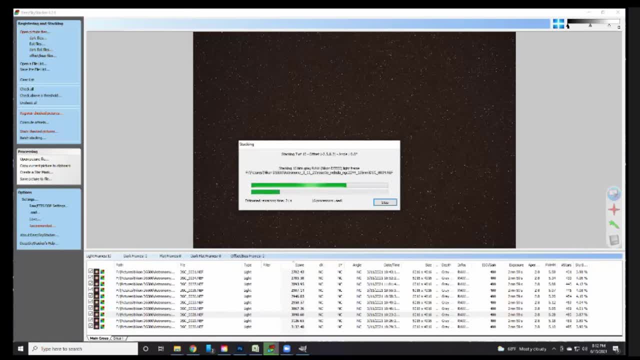 still took like 20 minutes to stack. So do be mindful that if you're gonna be stacking a lot of images, that it will take some time. So it's not something you could do on a live stream like we're doing right now. 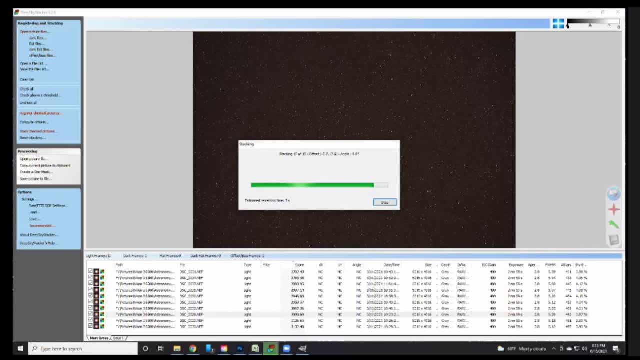 And that's kind of why I went with this target. It's only 10 images. It's something that will work pretty fast. Now, enough about the hardware. So the next step here you can see right now AutoStacker is creating what is called. 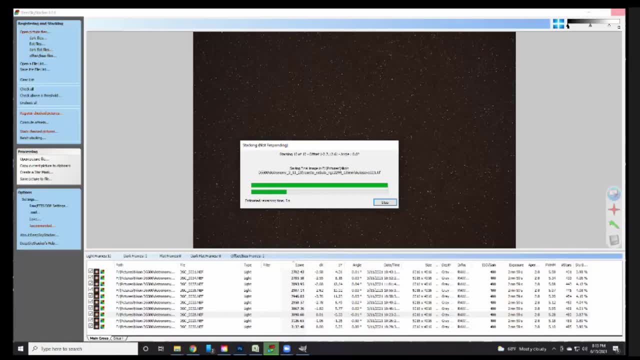 this autosave01.tiff. For the most part, you don't wanna ever use that file. You're gonna wanna. I'll show you the next step, which is you need to save it off to the resulting stacked image, to your own file. 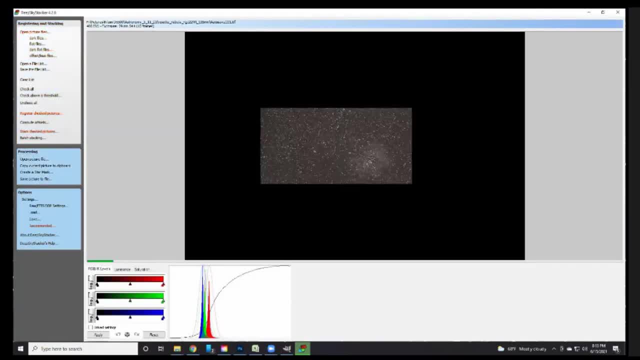 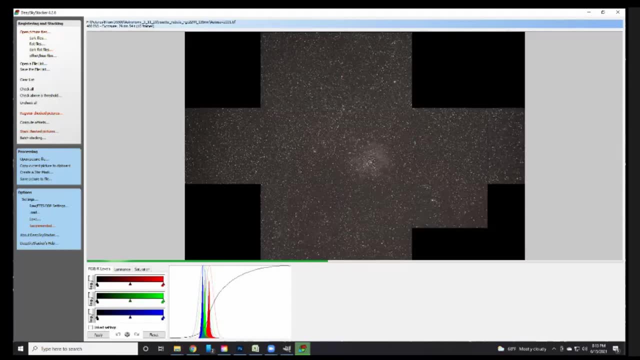 Most people say you should just throw away those autosaves right away because they're no good to you. You'll find they're stretched inappropriately and all kinds of things, And you can even do. as you see. it's slowly drawing out the stacked image now. 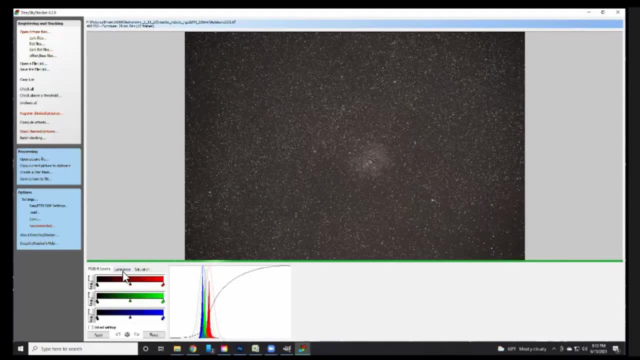 And you can even do some minor edits down here which you can, when you save, either save those changes or not. But again, I'm not gonna use DeepSkyStacker to do my edits. It doesn't make sense for me. 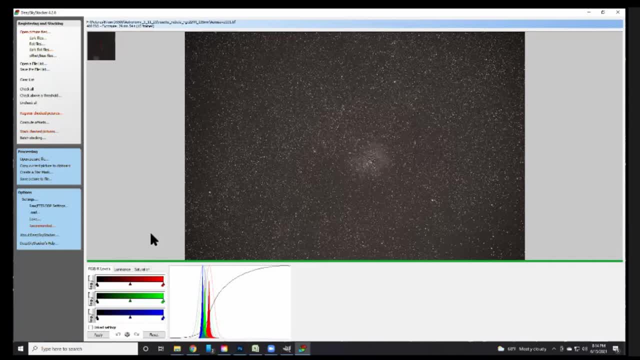 For me it makes more sense to go into editing software and do my edits there, But at least here what it's doing is at least showing you what it basically pulled out And if you notice, you can start seeing the rosette. 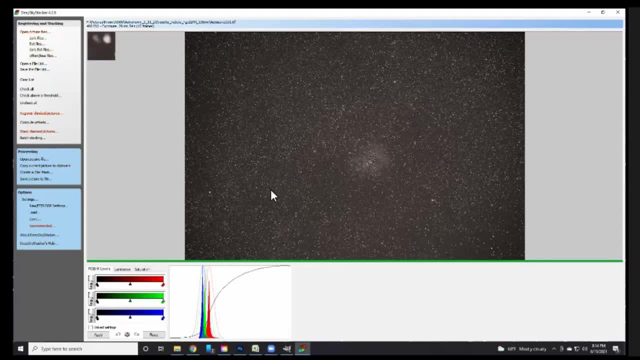 and villa showing up here. So that's at least gonna give you an idea that hey, at least I've got something to work with, And that's a good thing. But so what you'll wanna do then after that, after it's stacked, is do save picture to file. 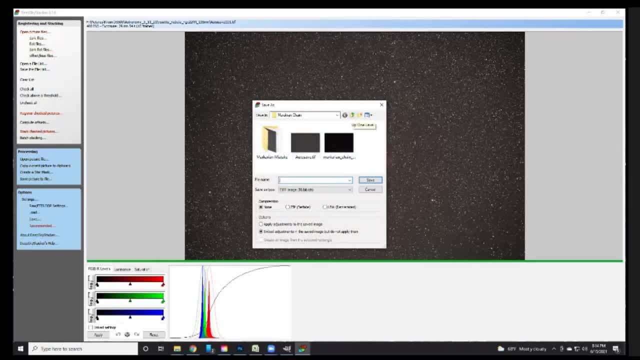 And so, like I said, I've already saved this, so I'm not really gonna do this, But the you can say what I do again. oops, Pass it there it is. So what I do is I normally name my file. 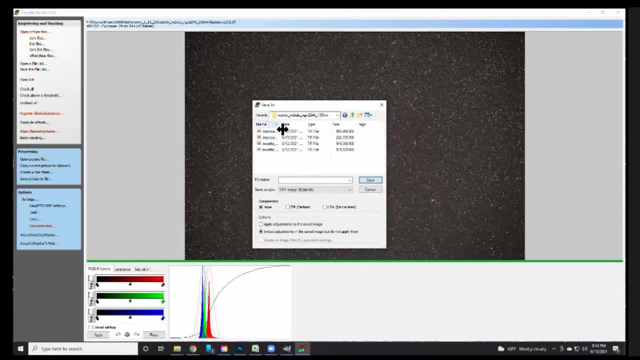 Sorry, let's put the details here so you can see the full name. I embed all that information I was talking about into the file name. So this is the rosette I used in this particular. I used a lens that I went and rented from Helix Camera. 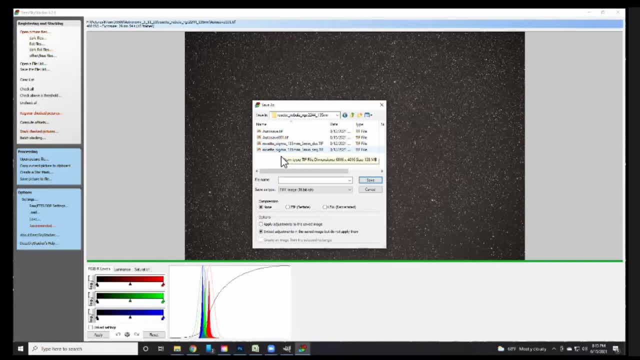 not to give them any promotion here, but I went and rented a lens that I wanted to use that allowed me to do 135 mils, So that's a kilometer shot 30 minutes. You can see that I once processed it in DeepSky Stacker. 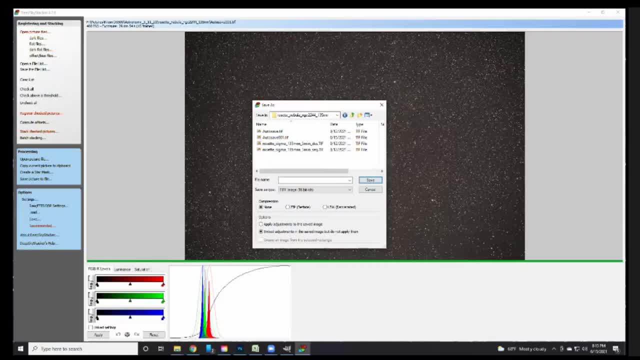 and one time I tried to do the second one. So I notate all that stuff in the file names. that way it helps me keep track of what I attempted if I wanna go back and try something else, something different. So that's so you'd wanna name it. 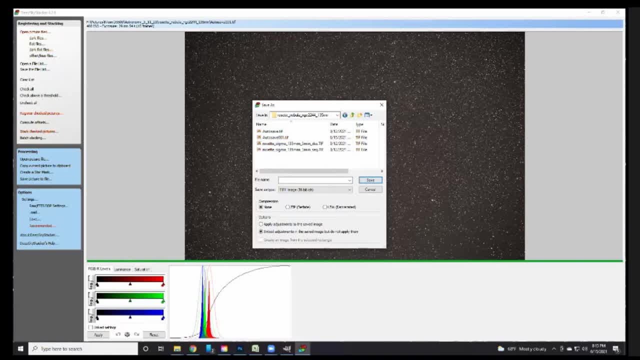 and it does create a TIFF image 16 bit channel. That's something you probably should leave and again, like I always say, I don't like to make changes. so So go ahead and check out the video description there. Stay tuned. 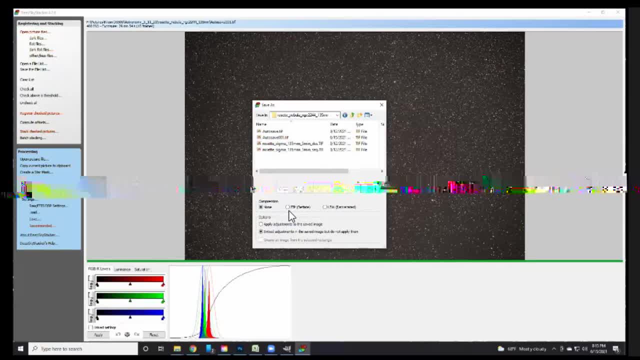 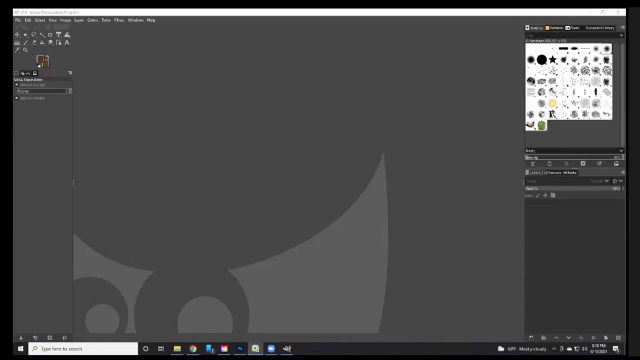 See you in the next video. Okay, bye-bye, Thank you, Thank you, Thank you. Astrophotographers are switching to PixInsight and that's a paid-for program. It's really designed for astrophotographers. is my understanding that when they first started developing it, they had astrophotographers in mind? 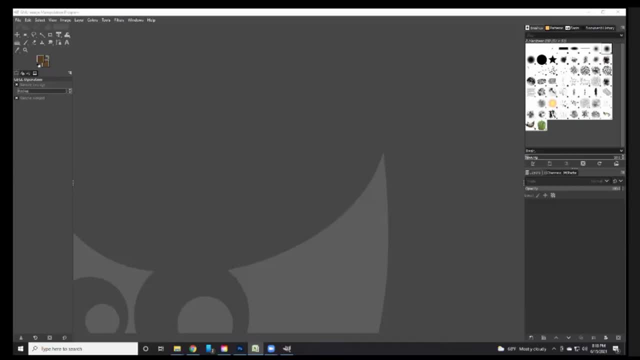 At least that's my understanding. I don't know. I don't know how true that is, so don't take that as gospel, But PixInsight has become really popular with a lot of the astrophotographers that I follow. There's a lot of built-in tools and automated processes for star reduction and star removal and stuff like that. 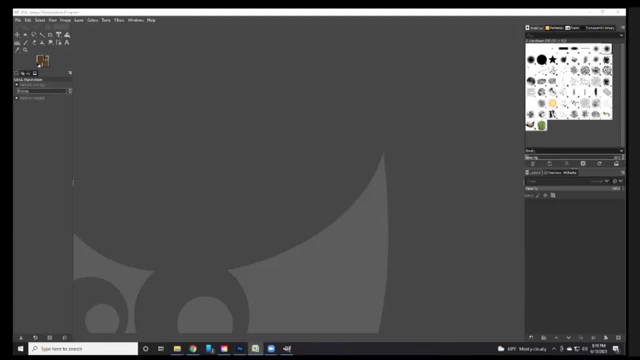 So, yeah, I'm already paying for a product. so I don't use PixInsight, but maybe someday I will, once I feel like my images are getting better, Maybe I'll pay the extra bucks for that. So for now, I'm going to close GIMP. 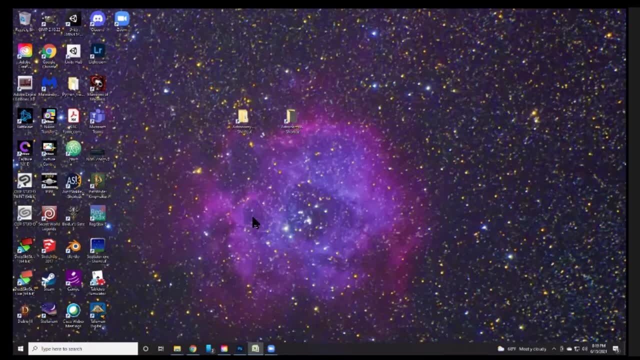 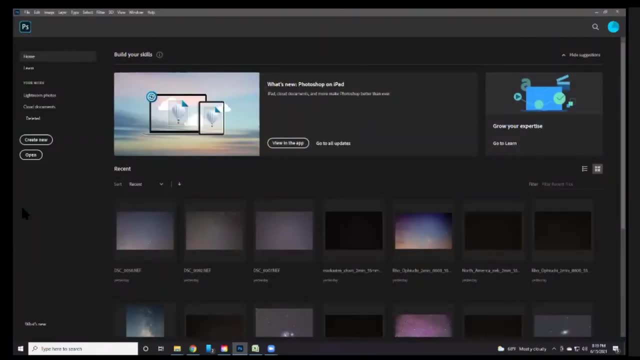 Again, if anybody has questions, I can try to answer them. about GIMP, I've used it a little, but not as much as I have on Photoshop, So let's see if I had any. I did forget to mention back when I do image review there's another Adobe product called Adobe Bridge. 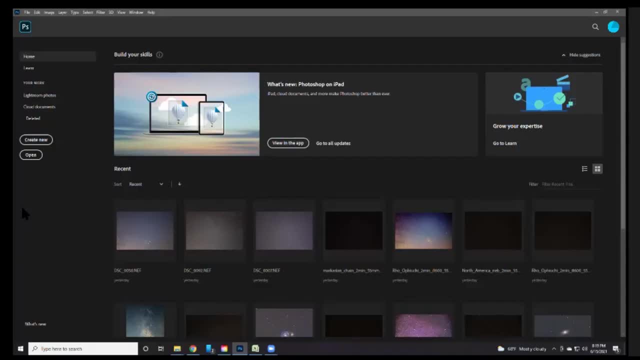 If your camera outputs an interesting raw image, it's going to be a good idea to use Adobe Bridge. If your camera outputs an interesting raw image, it's going to be a good idea to use Adobe Bridge. If your camera outputs an interesting raw image, it's going to be a good idea to use Adobe Bridge. 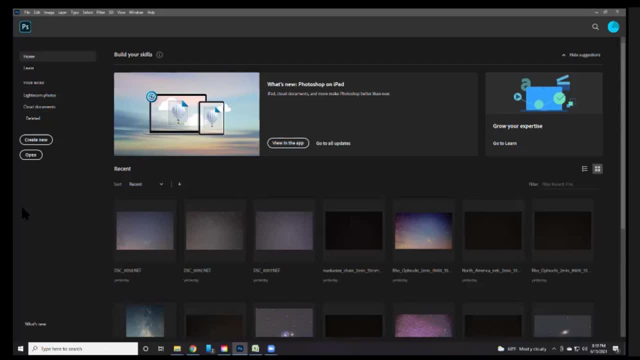 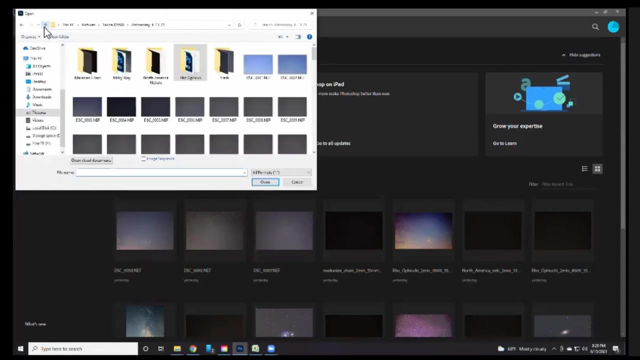 It might be something that allows you to do what it says: bridge it from your source file to a file that can be used by a product like Photoshop. So, anyway, let's go on here. So I'm going to go in and open this up, the file that I had stacked months before. 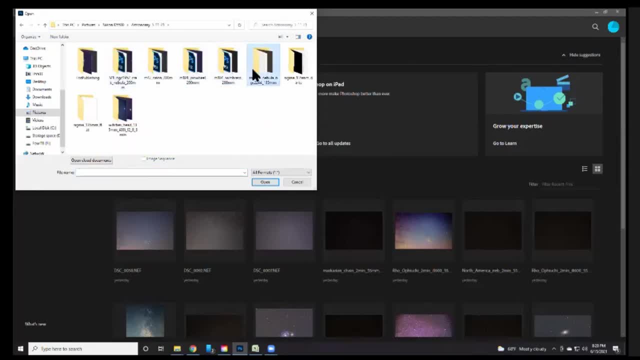 And we'll do that, And we'll do that. I'm going to go in here. I'm going to go in here. just this will be like a new version. i've processed this file a couple of times, so uh, yeah, it was a fun, uh, fun image, so uh to work with. so when you pull it up first, in uh, 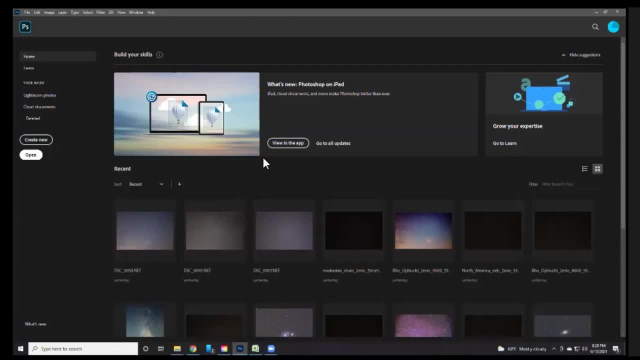 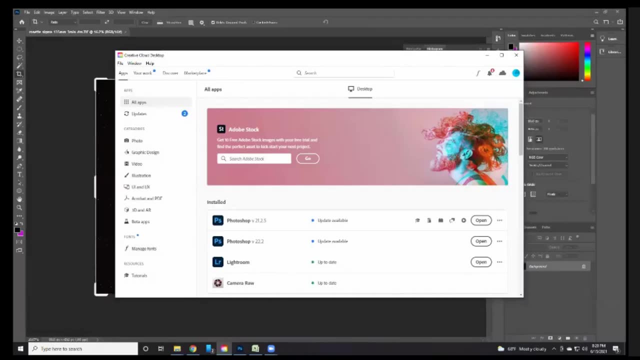 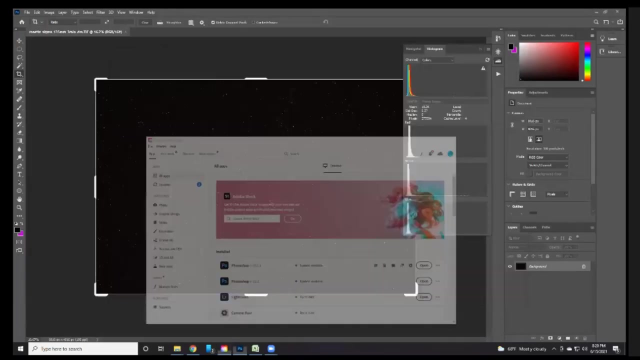 adobe photoshop. uh, now, i don't know how many people are familiar with adobe photoshop, but you get this product called creative cloud and you can open different versions of it, and, uh, i bought it when it was 21.25 and then they went on and upgraded and left me behind, so i have 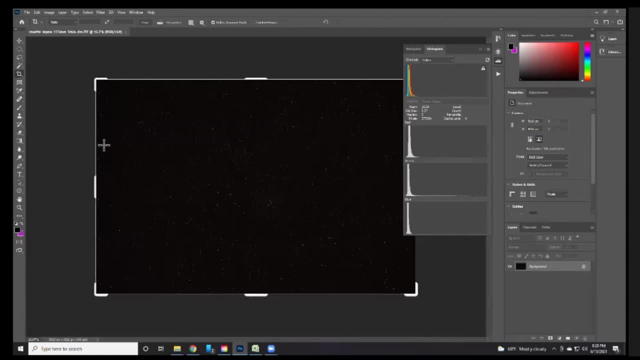 i still end up using 21.25. so, uh, in adobe photoshop there's a lot of videos out there that will teach, probably better than i'm going to teach even tonight, so, but i'm going to try to kind of go through the basics real quick as fast as i can. uh, hopefully not leaving people. 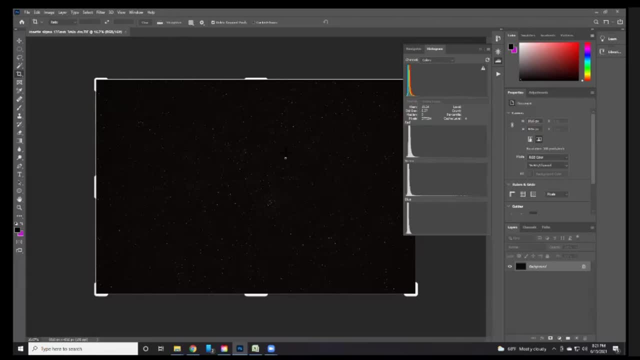 too fast or far behind too quickly. so one of the first things i do is, uh, take this layer- this is the layer panel over here- and your layout may be different. everybody can- you can- change this layout completely different. i've pretty much left it as the factory settings, basically, and so it should look very similar to the way i have it set up. so 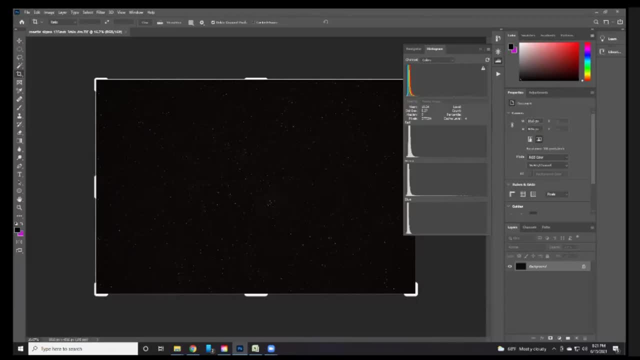 again. i guess i keep saying i don't like to make changes if i don't have to uh. so one of the first things, and i'm kind of following a gentleman who's named nico carver. he has a youtube site called uh nebula photos. again, i'm not trying to give anybody any extra free uh advertisement, but 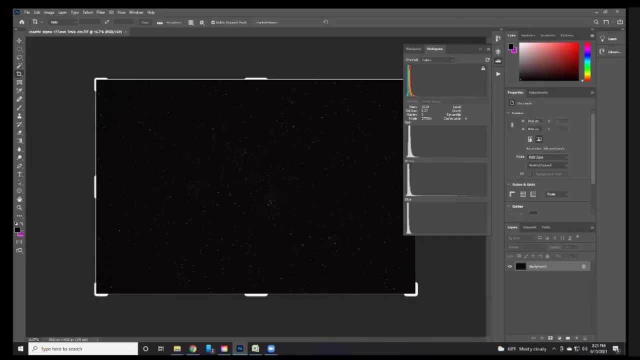 i do follow him a lot and i'm kind of following his process. so, uh, tonight. but there's other people's processes that i've adapted as well and use as well, so it's- it's a kind of mishmash of other people's work. so, uh, one of the first things i do is, uh, duplicate that layer just to um. 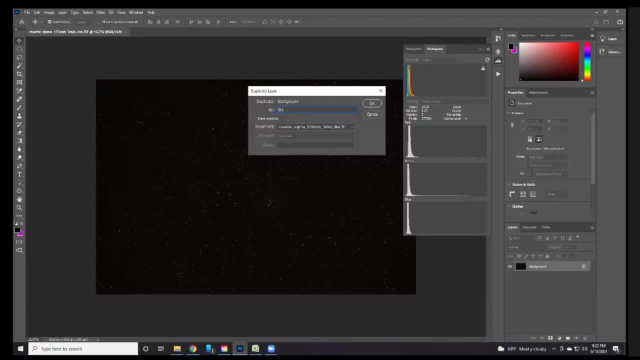 kind of keep track of the history, and i'll go over the history here in a second. so the first step here i usually is called. i call it first stretch. so what we're going to do is try to take this histogram. so again, this is found by clicking. 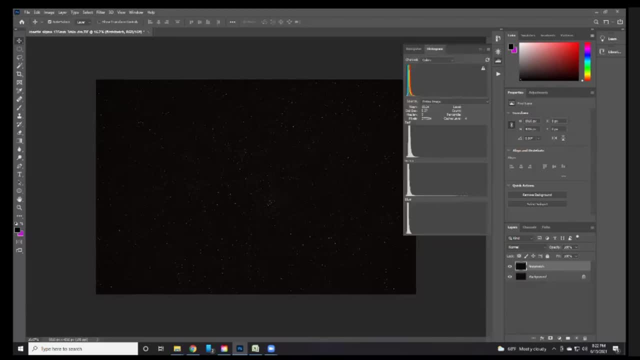 right here, this little histogram button, and it'll pop that window open. and this is kind of one of those things that i really like photoshop over again- where it shows you the different colors on this top histogram, which is the combination of these ones down here. these are the individual. 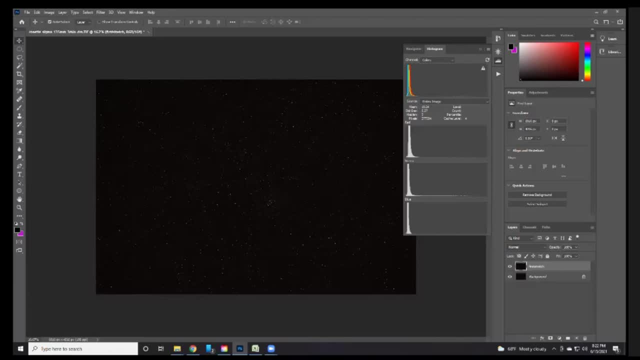 channels of red, green and blue. so it shows you the overlap with the colors and gimp, it just shows you a gray histogram. it doesn't distinguish the colors, and you'll see how that's going to come into play, uh, here in just a second. um, so, uh, one of the first things we'll do is try to get this. 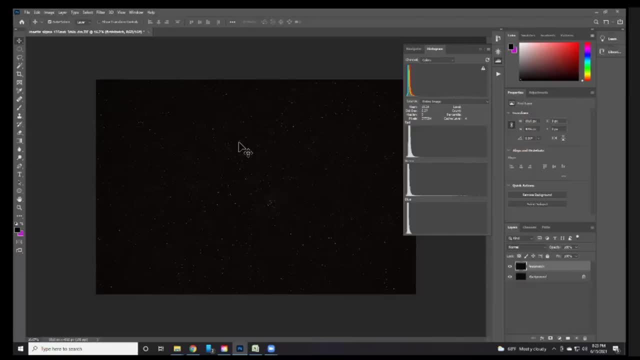 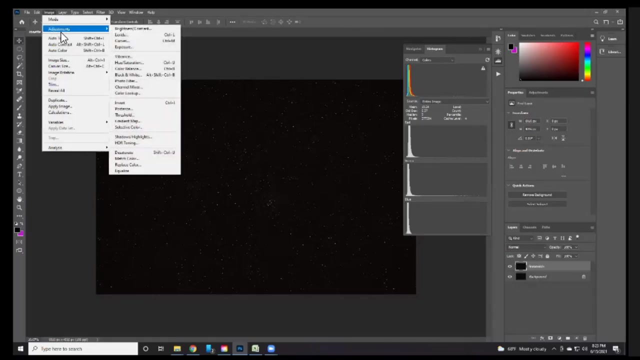 away from that left side, you can see how dark the image is. we don't even see the rosette nebula here in the center, like we did when it was in the sky stacker. so one of the first things that i'd like to do is go up here to image, go to adjustments. i'm going to try to go slow on. 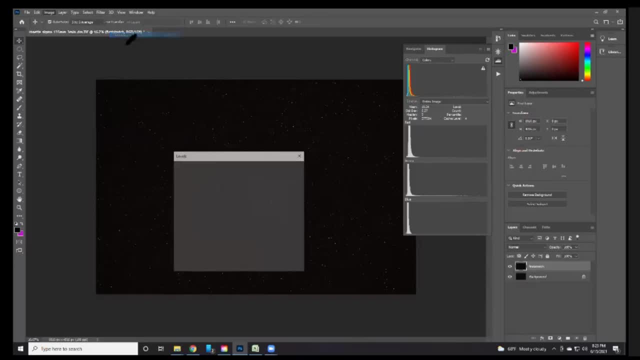 the menus, because i know most video people do it really quick and then go to levels here. so we're going to adjust the levels and we're going to start off by adjusting just the general rgb, which means let's affect all three channels at the same time. now on the histogram, again, this: 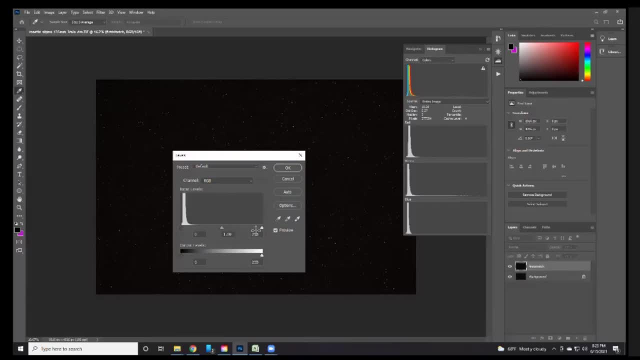 is where your data is, where that spike is. over here to the right there's no data, basically black image. so there's no very few highlights. the only highlights are the stars. so what you can do the first time is go ahead and stretch your image. this is called stretching the, the data, so it's a 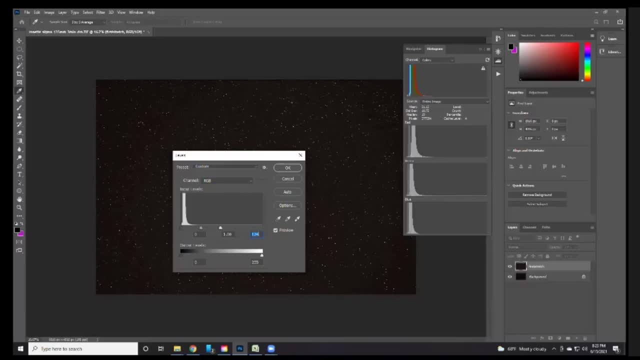 little bit fatter. you may see all those columns got fatter right away. so that's what you want to do if you're going to try to make those a little fatter so you can pull out the color out of the image. so i'm just going and now, uh, one of the things is the way i'm doing it right now is 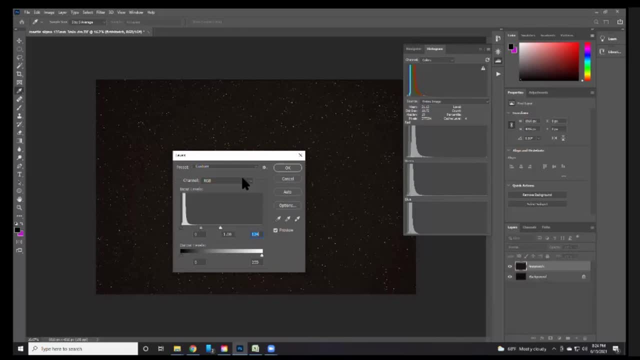 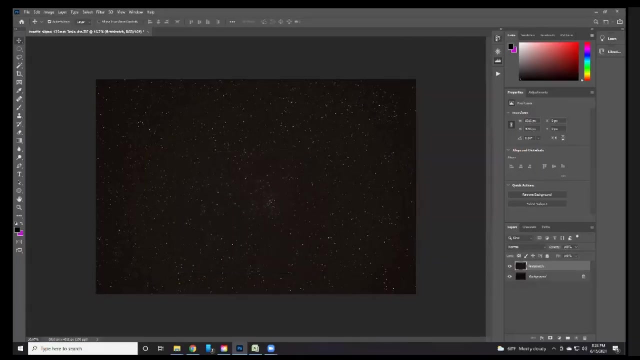 what's called a destructive. a destructive, uh edit. so once i make this change, it's kind of permanent. kind of permanent because, uh, there's a way to uh get around that, so i'm gonna go ahead and click. okay, so the way to get around that is through the history tab up here. you can always go back through. 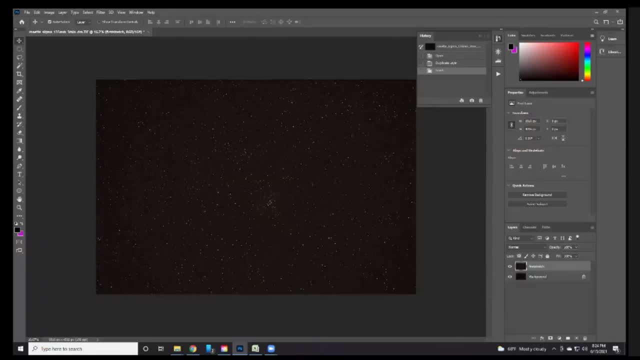 the history and delete your step, whatever you just did. so i can just go back and delete that and we'd be back to square one. so that's the way you get around it, but these what i, the way i just did that. levels edit is called a. 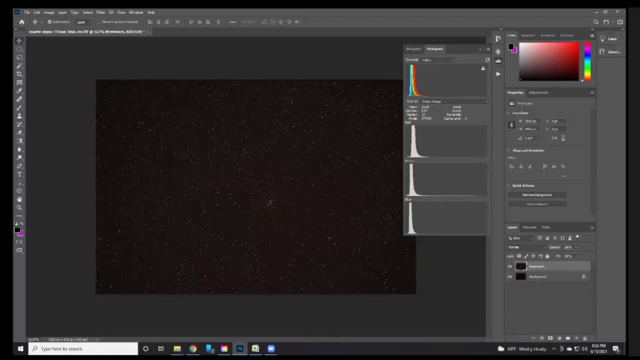 destructive because it's not something i can go over here to my layers and turn on and off. i can see what it was originally, but i can't see the individual layer or level edit that i did. there's there's no way to just turn that one particular edit off. so 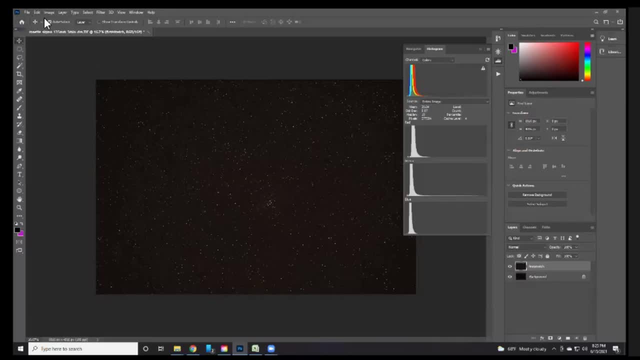 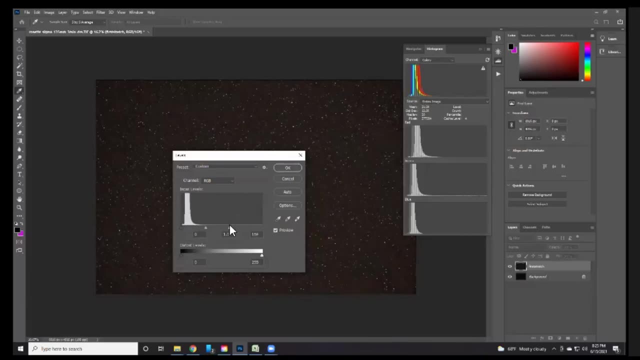 uh, that's why i call these destructive edits, so i'm gonna do that again. uh, that's that lightened my uh image pretty well, but still not very light, so i'm gonna stretch it again. just again, i'm trying to get some of that that those column, those histograms on the right side. 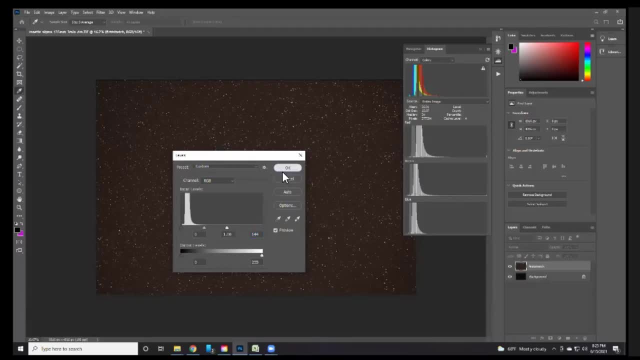 of this window to be a little fatter, so we're getting into the real data. so again, i just stretched and said yes, and then, if you notice, there's this little triangle here basically saying i haven't been updated the histogram properly, so i always click it just to make sure i. 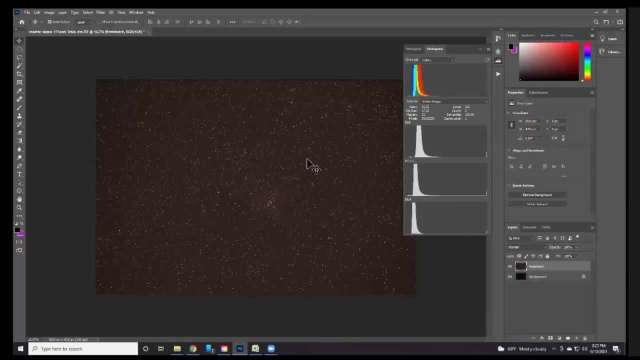 can see it. so i can see the histograms are updated. now one thing, uh. at this point you notice that the red channel is nice and fat, and it's the one furthest to the right, and you can see that clearly up here on the top as well. what i want to do to try to make this a little bit more balanced is: 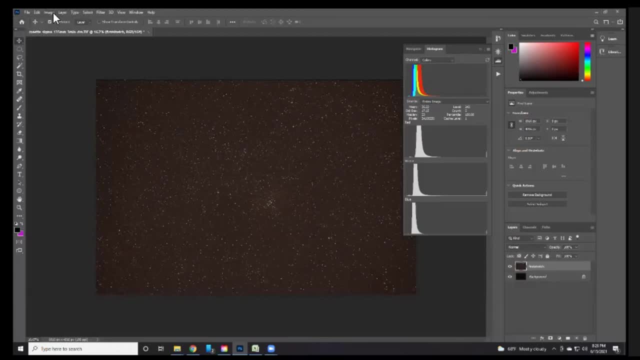 color balanced is by pushing these columns for green and blue to the right. so i'm going to do another destructive edit levels again, but this time i'm going to select- here i'm going to do a- which channel i want to change. and i'm going to change the green, and what i'm going to do is: 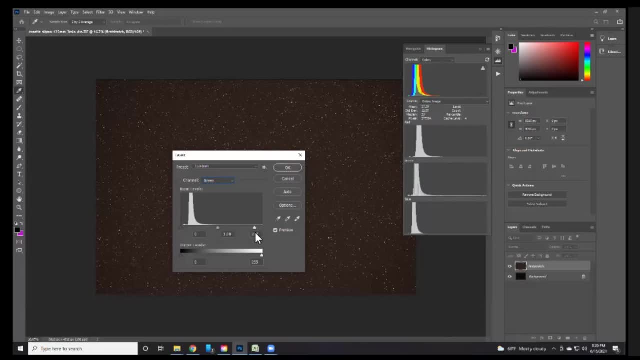 again. push this down. and if you watch the right side of my screen, you'll see that column is growing and moving right, and on top you can see that the yellow band is getting better, bigger because the green and red are mixing. so that looks good to me. i mean, it's pretty. 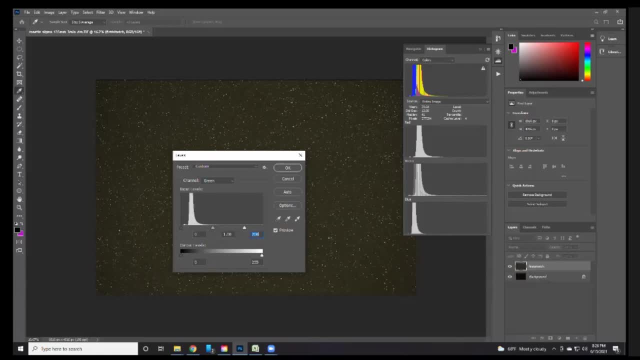 bad. it's not exceeding the green, isn't jumping out a little bit, maybe on the edge right here, but that's not bad. so i would say, yeah, that looks good. uh, so i'm gonna do that same exact process. i'm gonna try to push this blue column over. 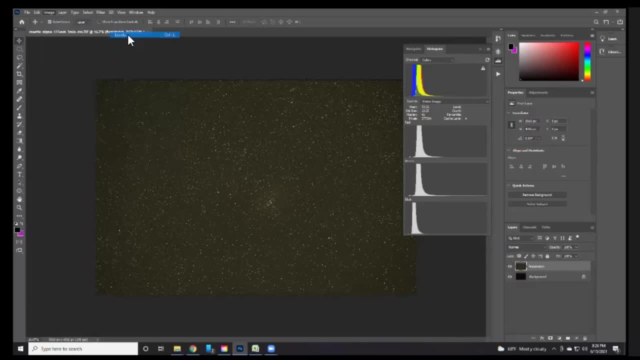 and and uh and get it uh to be more in line so that they are all stacked up. so push it over again. i'm grabbing the highlight of the blue channel and sliding it to the left until it lines up properly. now, i didn't switch the channel and that's why everything was moving. 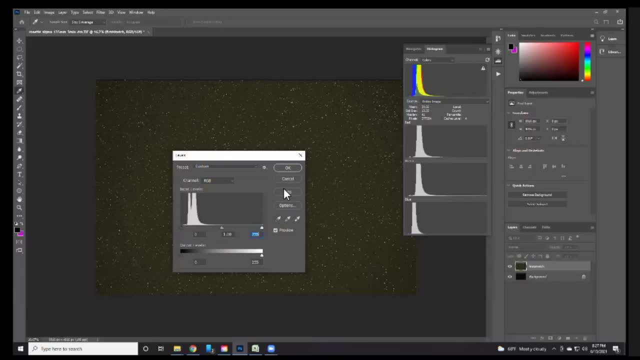 so if you start doing that, you see that something's really crazy. you can always cancel, which is a good- another great thing- but uh. so what i forgot to do, though, is change my channel so that i'm only editing the blue channel, and now you can see only the blue one's moving, and again. 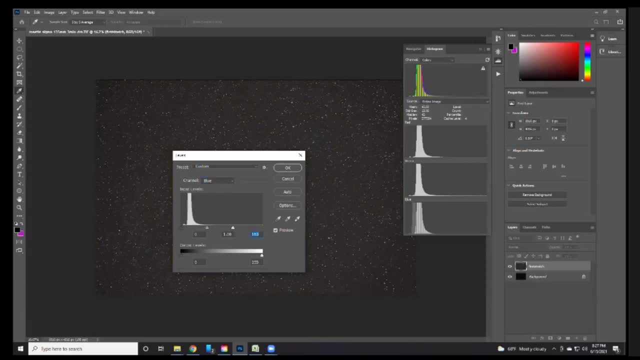 i'm going to try to line it up so that that blue channel is right underneath, all lined up, and up on top there's no separation between the different colors. so click ok, say yeah, okay, that looks pretty good. now you notice the image has gone pretty flat colored and you can start to see some vignetting. 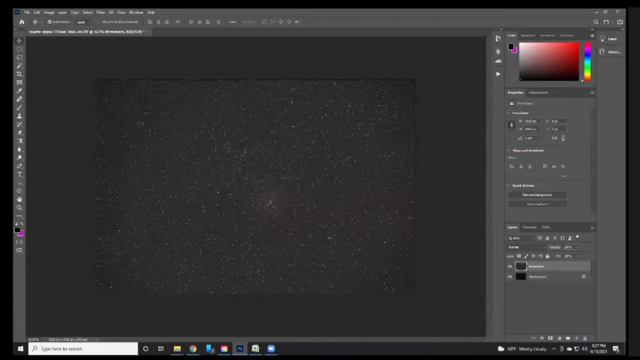 on my image and that's a. you know, that's a result of my imaging train, so that's something we can take care of right away, which you, i may as well do right now- which will go and prop it. so i don't have that information interfering with my histograms, so i'm just going to use the crop tool up here. 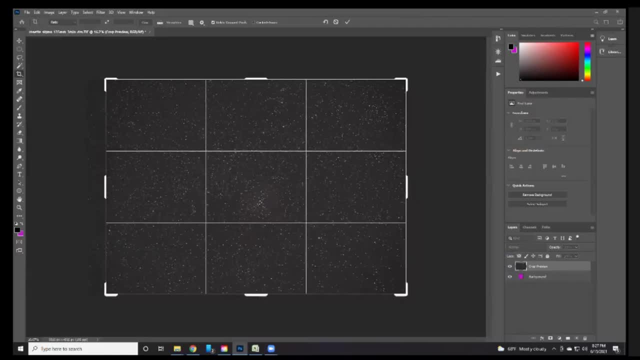 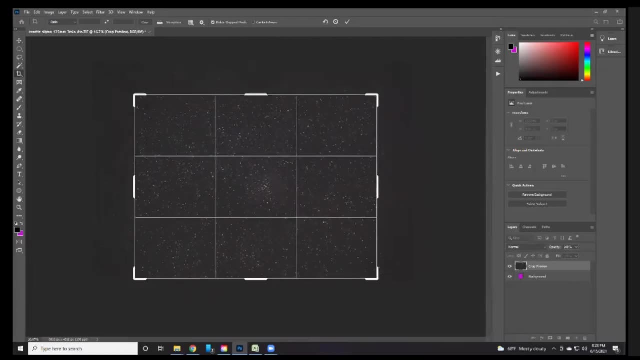 it's pretty standard tool in most imaging editing softwares and i'm going to get rid of those corners because i can see my targets right there, and i'm going to bring it down. and i'm going to bring it down to this point. you're going to start using your eye, your artistic eye. 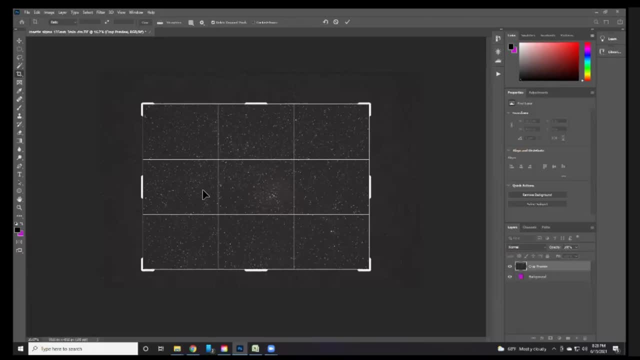 at this point, because the reason they split this crop tool up into these segments or these quadrants or no quadrant, whatever it's segments on this segment- is because of the rule of thirds. there's a third up here, there's a third here. so what i try to do is i either try to center my 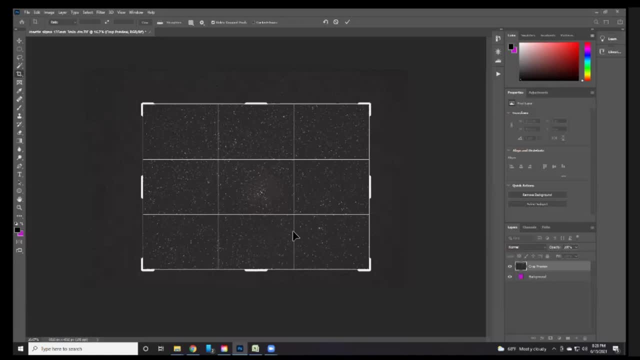 object. but let's say i have a bright object, like, let's say, this bright star here i want to balance with, maybe, negative space. so this is where, again, the artistic side of you can come into play and you can try to frame up your image exactly how you want it. let's say you wanted this extra. 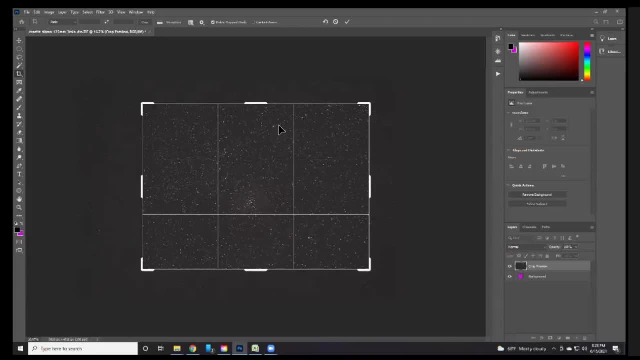 bright star up here for whatever reason, okay, or there's some more nebulosity up there. so the only challenge with doing a crop at this time is: maybe you don't see everything that's in that image, so actually i will go ahead and back out so you can stop that process. you can say no, don't do. 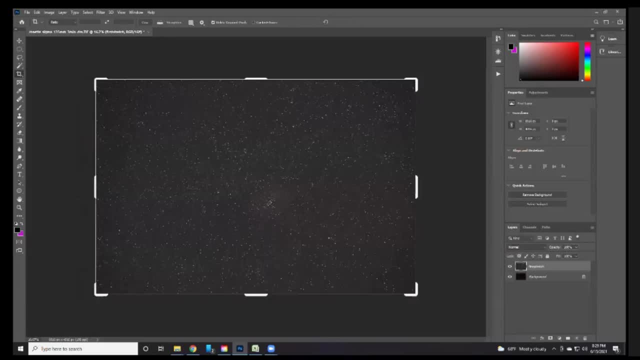 this. you can hit escape. i can hit escape at this point and it'll back out and not do that edit. so let's go ahead and move on and, uh, or you could have used your history. if you did end up hitting okay, and then you realize you cut off some of the nebulosity around this target. you could always go. 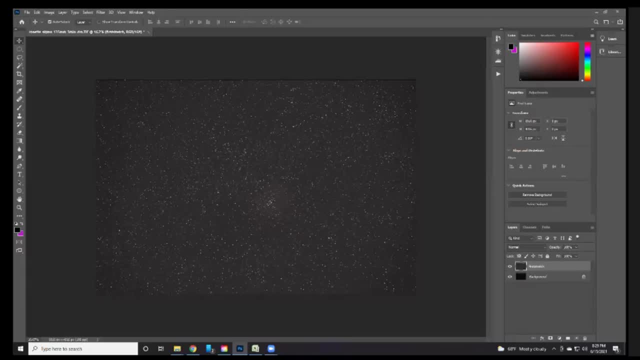 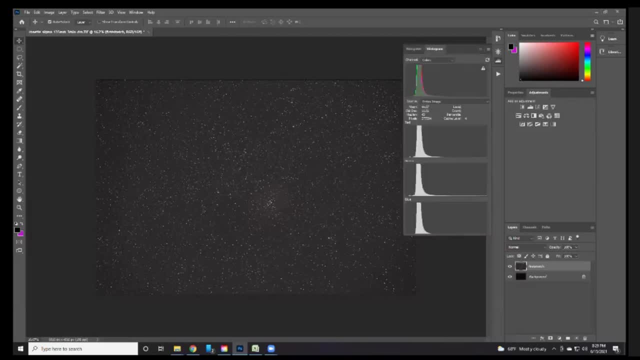 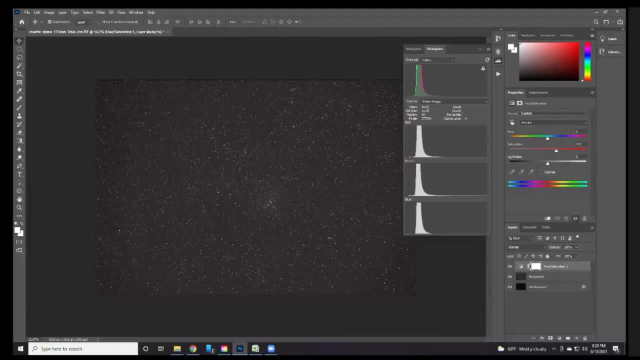 saturation a little bit here, uh, just a little, just to try to get, get, get those uh histograms to fatten up a little bit. so that looks good now. this is a non-destructive edit because i can sit here and turn it off and on and see if i like the change. so what it did by doing that. 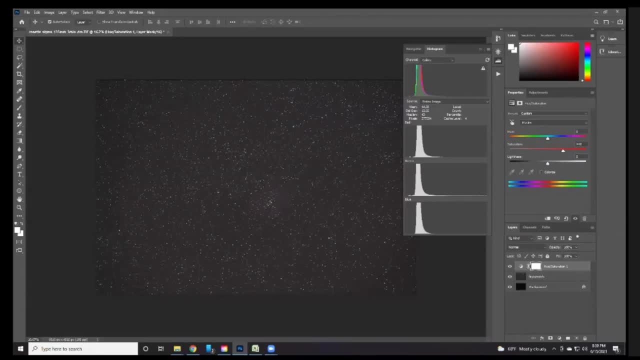 increasing that saturation. it did add some red hue to the entire image and hopefully you all can see this on your on your screen and uh, so that looks okay. but i can, uh, if i didn't like that red hue that it introduced everywhere, i can go into the color balance and adjust that. but to be honest, i don't need to do that because 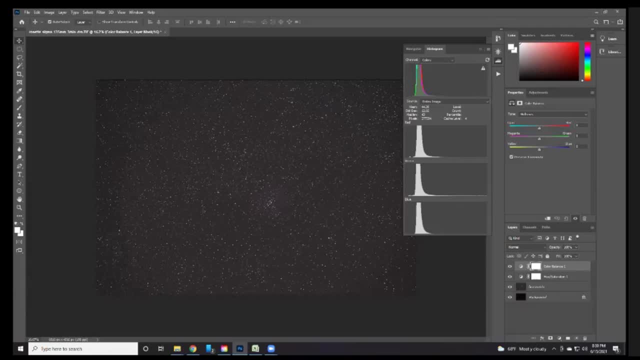 this is a relatively red object, so i'm not going to do that. i'm going to go in and i right clicked on that layer and now i'm just going to leave that layer. instead, what i'm going to do is i'm going to add a curve, so the levels 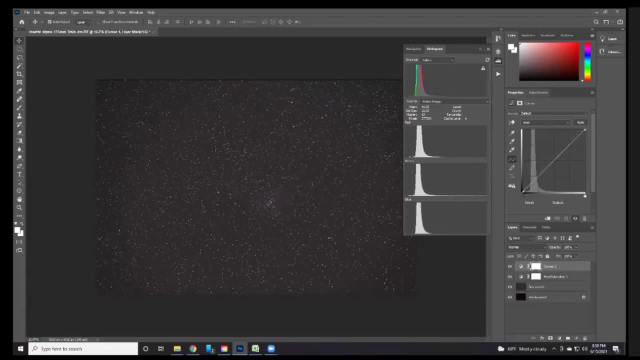 curves, color balance and hue and saturation, or this vibrance tool. those are some of your primary things that you're going to constantly be using to try to get your images to pop out. so in this case, i'm going to go back to my curves tool and what i'm going to do is what's called an astro. 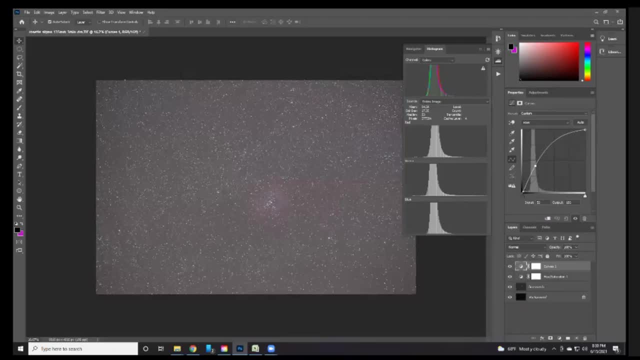 curve, which is basically this: now, you don't want this line to go all the way to the top, because you're going to start clipping data, and you don't want to do that. you don't want to clip data, you want to keep as much data as possible. so there's that, um. 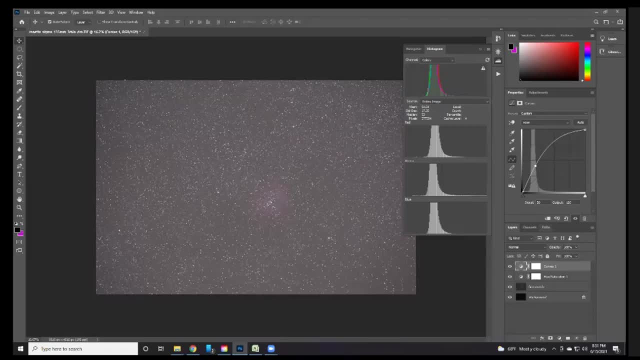 you can see how it increased the brightness of the whole image. so if you're at, if you're pulling up, if your point that is created on the line is over, here you're high, you're increasing the highlights. if it's down, here you're changing the darks. 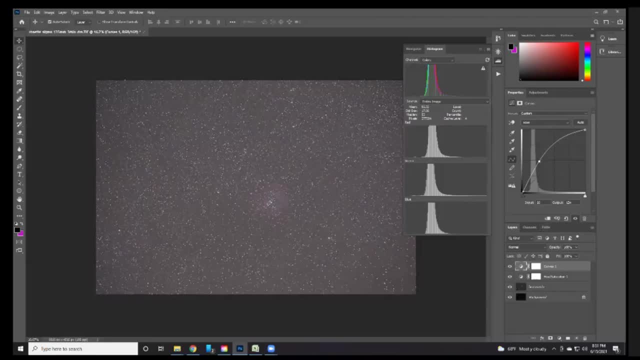 so what i did was kind of, in the middle: increase the whole image. i want everything to brighten up, so that pretty good. now what i might do at this point is go ahead and say i want to create a second stretch, i want to adjust these now. some people go through a really long process of creating a mask to 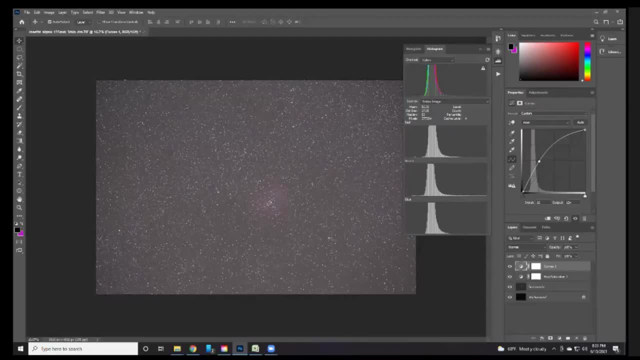 identify highlights and blacks and all that stuff. but i'm not going to do that. that's really involved, so but i'm going to just kind of. i know i'm already getting long, so i'm going to do what's a keystroke here. it's called control alt. 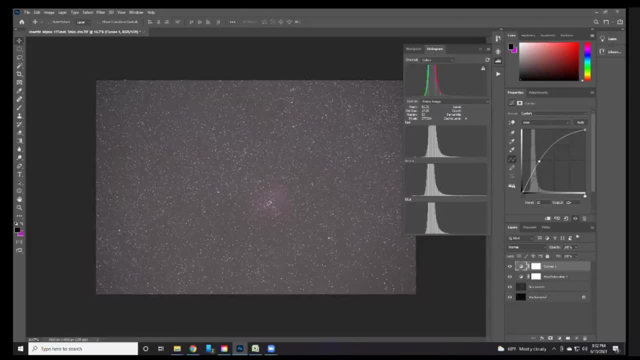 shift and e is an echo, and that what that does is to say, take what's on the screen now and give me a copy of it, and it creates it as a layer. so there's a, there's a menu way to do it. i've just learned the shortcut key, uh. so my apologies for that, but uh. so i'm gonna call this my second, uh. 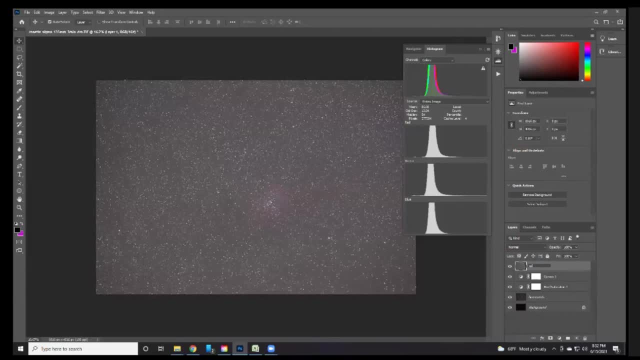 i'm gonna call this my second stretch. i just double click to get that and i'm gonna mess around with those permanent edits again. uh, with my lulls. so i'm going to try to speed this up a little bit. sorry if i am going too fast. first thing, i'm going 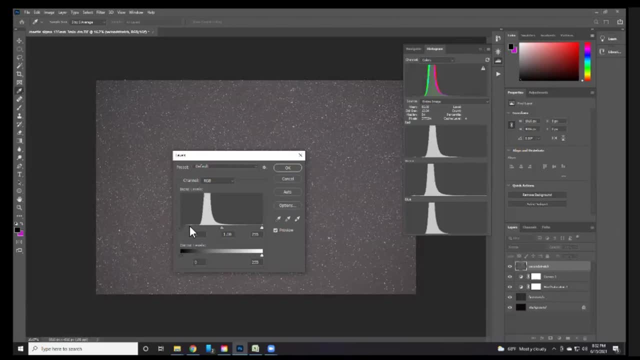 to do is set my blacks and you can see this black is not even in the data, so i'm going to reset my blacks. i'm going to slide this over, pull those bumps back over now. i might be losing a little bit of dark data here because you can see there's a little histogram, but for the most part it's. 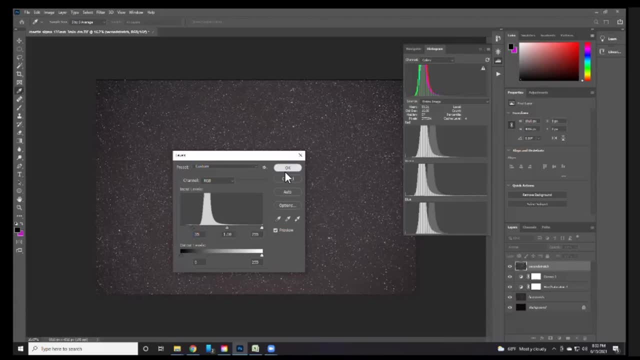 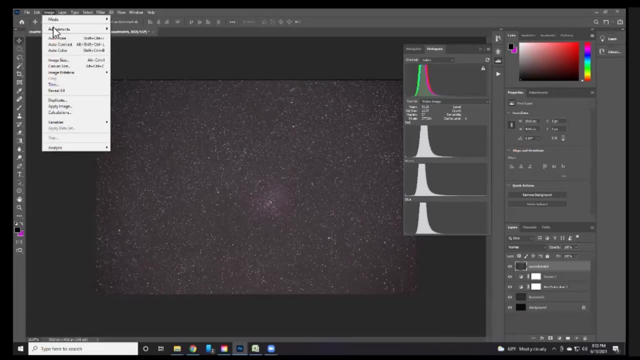 probably not important, and it could be coming from my vignette, so i'm not going to worry about it. so i'm going to click. ok, you can see there's a little histogram here. see how that got pulled over. okay, and again, i'm going to speed this up a little bit more. 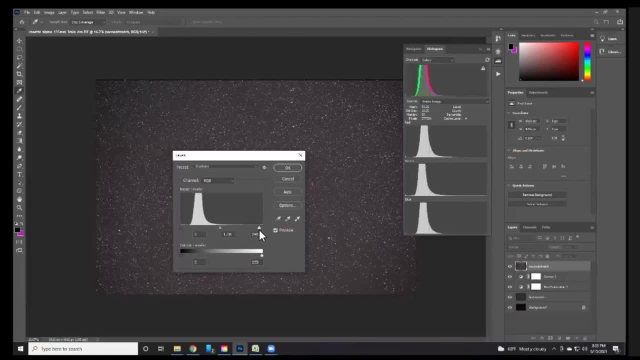 adjustments. again, same thing, over and over again. i'm going to pull this over, try to lighten the image- now that i just darkened it- and try to get more of those colors to show up. so i'm going to click ok, and then i'm going to hit my triangle here again to make sure my histograms 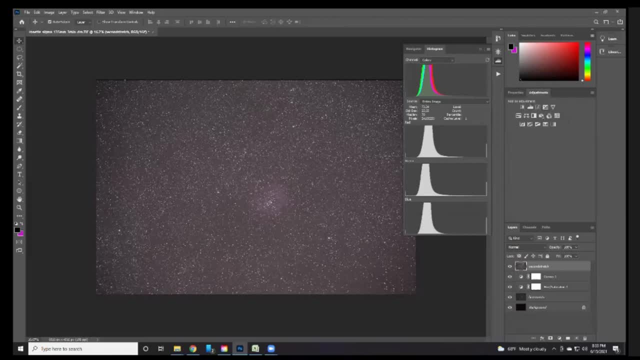 are updated properly looks pretty good. now i'm going to go back to non-destructive uh changes, so what i'm going to do is add some contrast. so this is a typical curve edit. so you pull down the blacks, you want the darks to go down, but then you pull up. 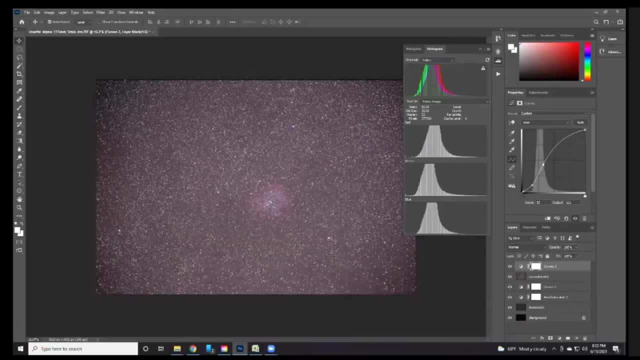 the mid and the high highlights, and this is called the s curve and it is used for not just astro imaging. it's used for most image editing that is done on and adds contrast to your image. so now my represent is really starting to pop out. there is a little nebulosity outside there and i'm 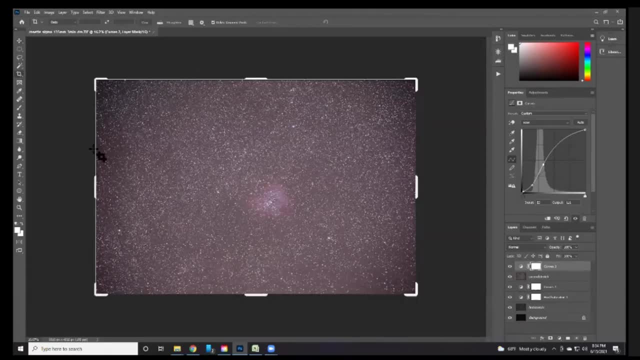 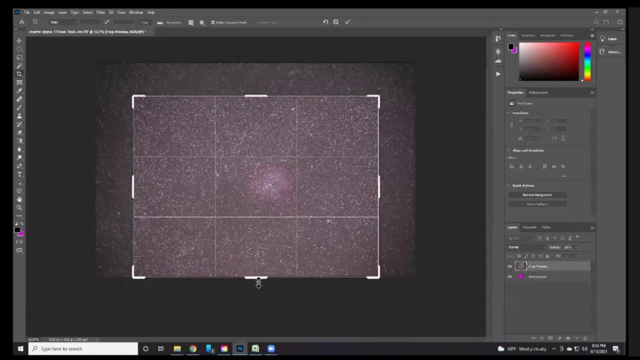 going to get over here and add a little bit of contrast to the edges there. so i'm just going to paste that around the edges so that it looks more like a black exposures. so i think i might have cropped it earlier, but at this point i am going to crop it just to get rid of those edges. 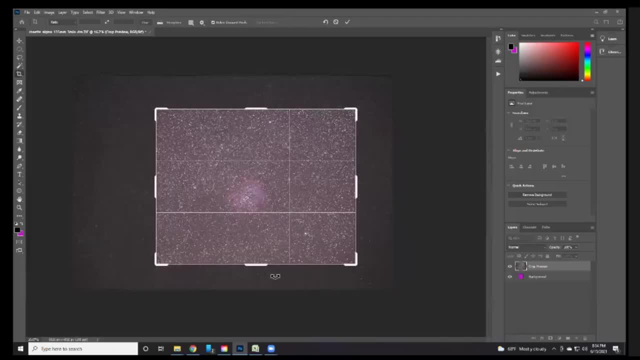 that i don't want. i don't want to worry about my- uh, my- vignette, and i'll try to frame it up how i want so that looks good. i'm not going to take long on that, so that's uh, you know where i propped it. 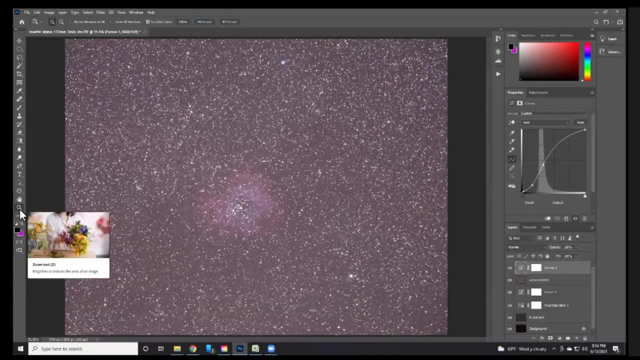 too a little off from center, trying to hurry up a little bit here, i'm going to fit it on screen, so so that's the magnify tool. uh, at this point there's two quick things i'm gonna show you, and then i'm gonna kind of try to wrap things up because, again, you can do this all day long. 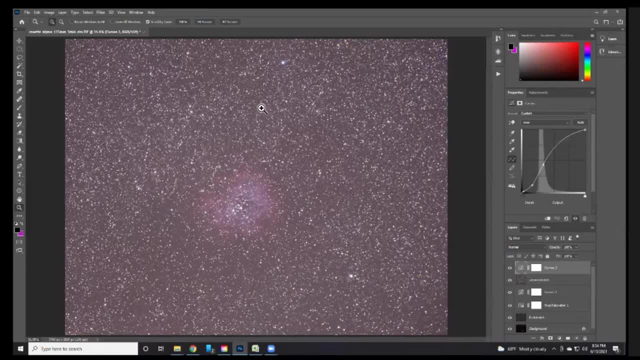 you can let your creative side come out and do this: uh, keep twerking, tweaking each little channel. you can go to these other tabs and really start working with things. you can create masks, you could do all sorts of things, but these are some high level edits that you can do again in 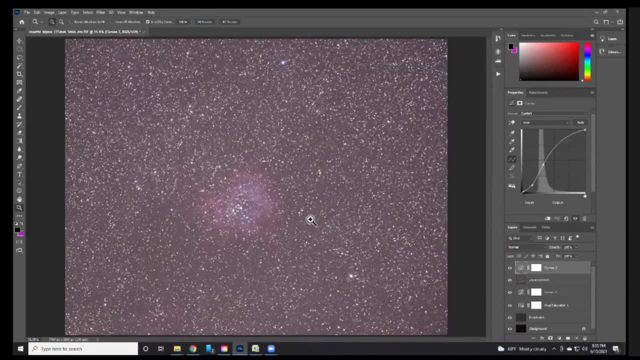 gimp or all your other editing tools that should do basically the same thing and get you similar results. uh, the. so my next, uh change. actually, i am going to add quick vibrance and saturation. i want to make that object pop out quite a bit. it's getting much better. and then what i'm going? 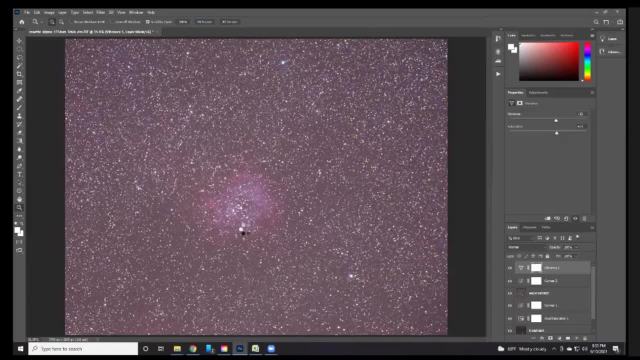 to do from there is go and create another layer, that keystroke action that i was talking about, and i'm going to call this one acr. that's what nico does. uh, it stands for adobe acrobat filter, which is up here. so you go up here, you go to filter and you go camera raw filter. 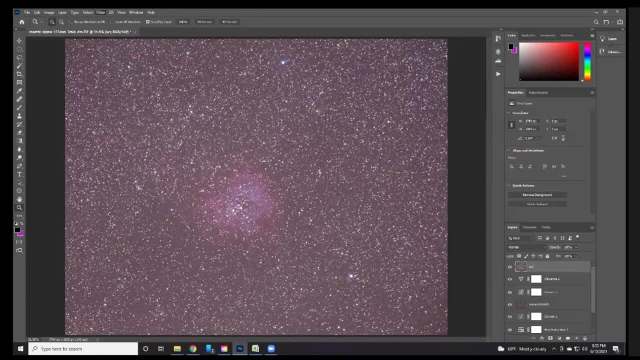 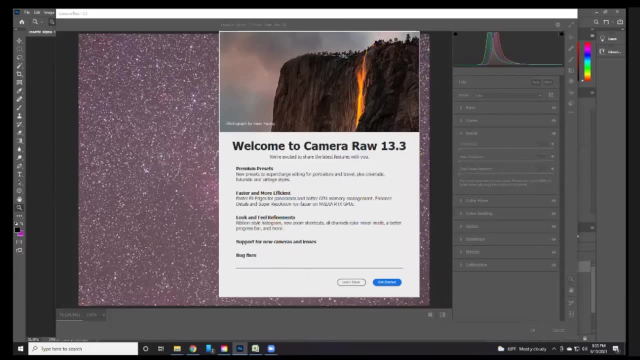 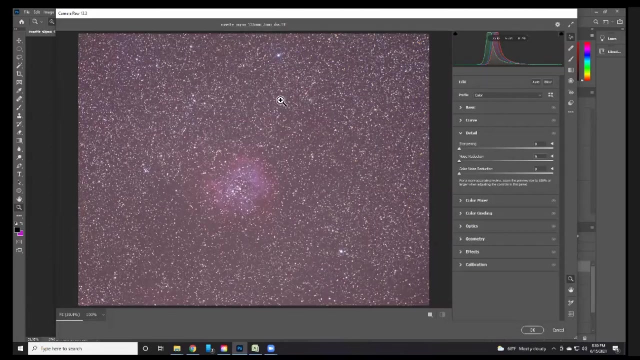 so what that's going to do is bring up another element. it's almost going to bring up what's exactly like: um, uh, sorry, i don't know what that is or why this popped up. um, so anyway, uh, that's been a new update: the. the sliders are very slimmer, similar. 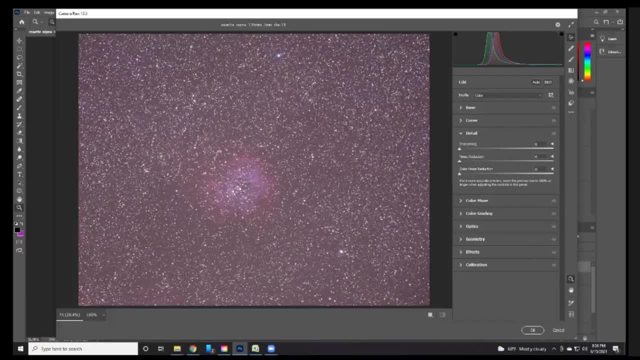 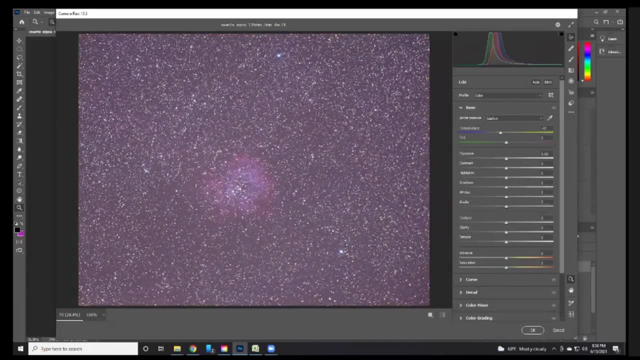 to the light room edits. so at this point i do want to do that type so, but i typically only use this for some basic edits. first, if i want to warm up my image, i could warm it up by adding some. well, warming up would be this way: cooling it off. 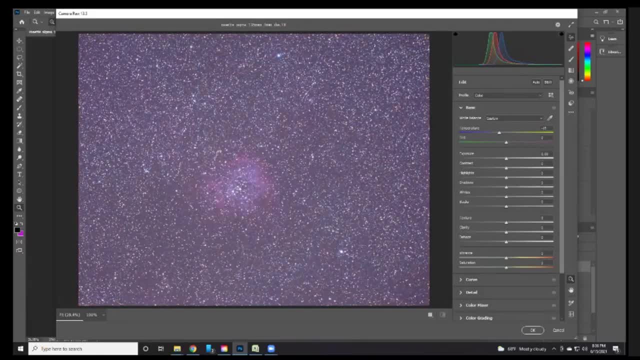 it's going towards the blues, to bring that blue color out a little bit. i like the blue or purple. uh, adjust the tint a little. maybe a little too purple. uh, maybe you want to adjust your blacks to make them a little darker, but that looks a little too contrasty to me. 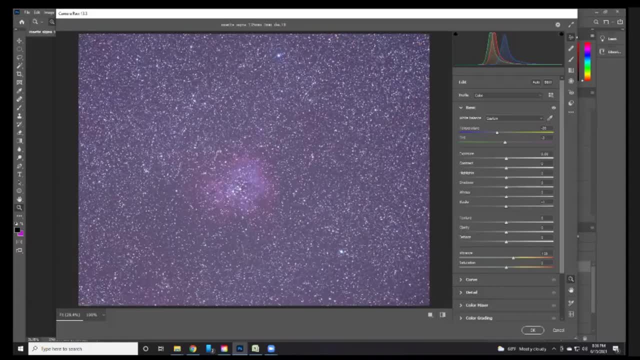 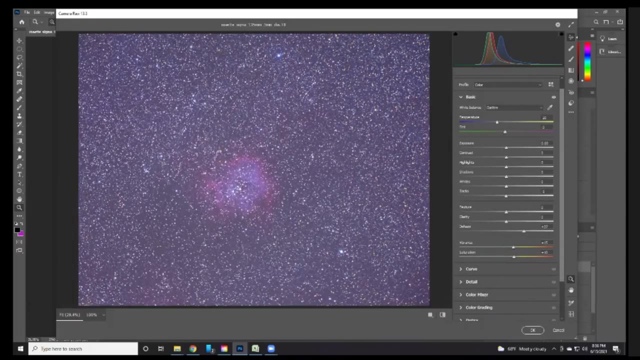 uh. another thing is, of course, again moving with your playing, with your vibrance and saturation. again, you're using the same edits over and over again. uh, d haze is a great slider. uh, yeah, that looks pretty good. all right, and you can play with all these sliders and uh. 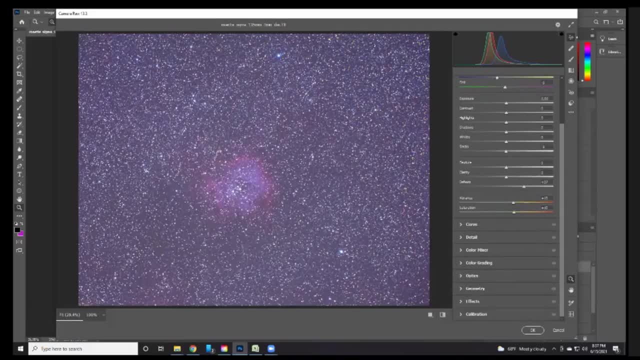 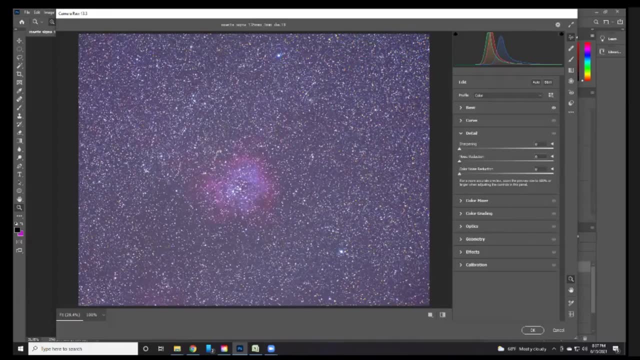 but once you do it, you'll be able to apply that now. the main reason i use this filter is because of the detail, so why i'm in here. if you notice, it switches to this. uh, my cursor is turned to a magnifying glass if i zoom in. there's not too bad, but it's, there's some. 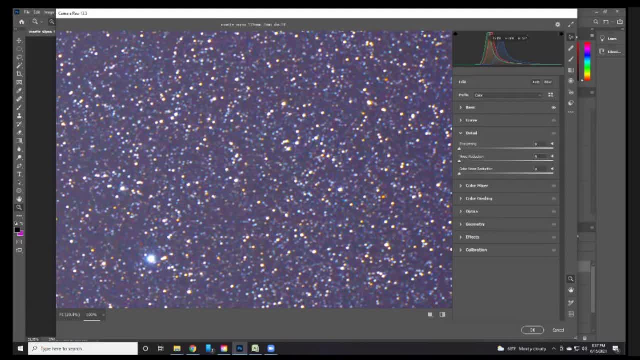 uh, grain and color noise coming through. not much on this image, because it's a pretty decent image, uh so, but i usually do use the noise reduction and the color- uh noise reduction, so you may lose a little detail doing this, especially like when working on galaxies. but 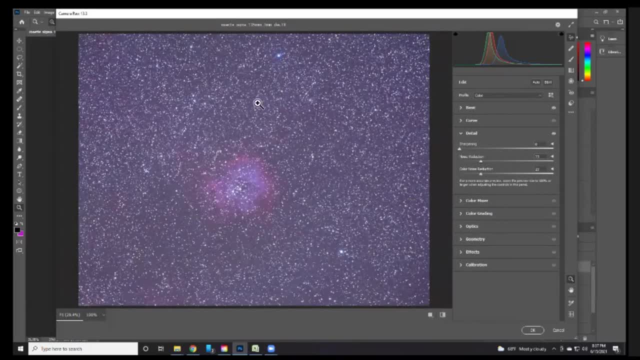 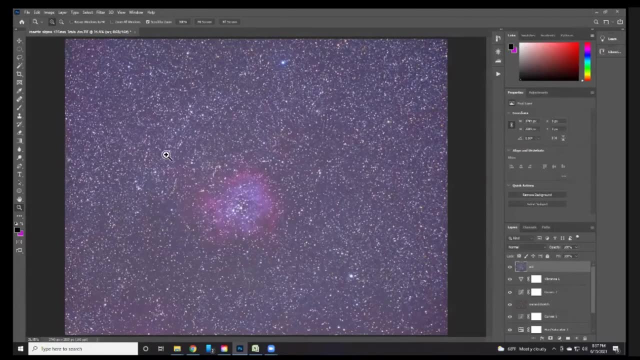 on this image. it should be okay. so those, that's what i typically use that, uh, that tool for. so then you just click ok, and it comes back here and you can see that changed it dramatically. but again, if you didn't like it, you're like: wait, do i like it better there or there? 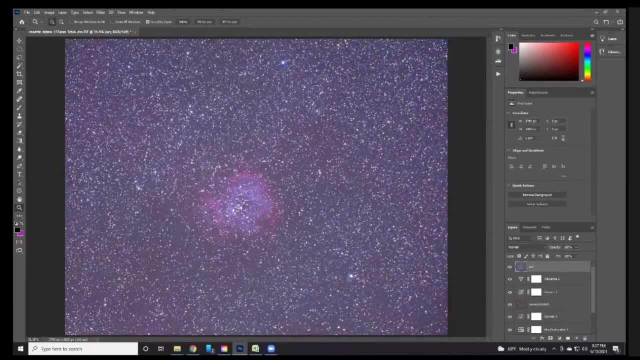 i like it better there, so, uh, that's why again, these layers the or you didn't like how strong that edit was. you can adjust its opacity on this particular layer by selecting this layer and then just adjusting its opacity. let's say, i don't want it to influence the. 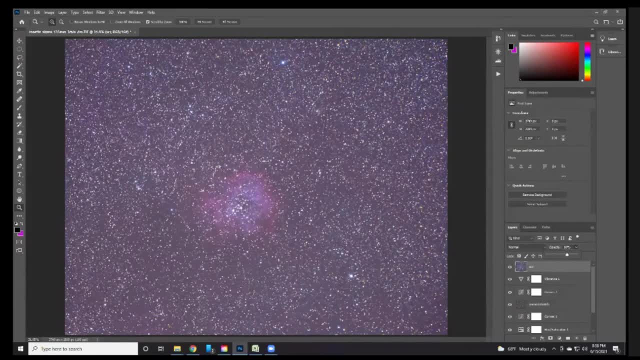 image that much, so i'm going to slide it down a little bit, let's say down to 66, and now it's affected it, but not as much as it originally did. yeah, i like 100, so i'm gonna leave it there. um, let's see. at this point i would 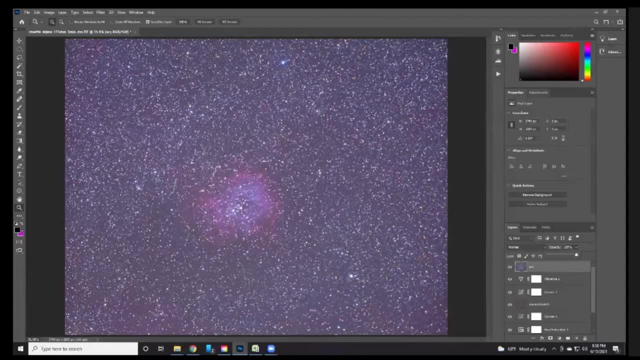 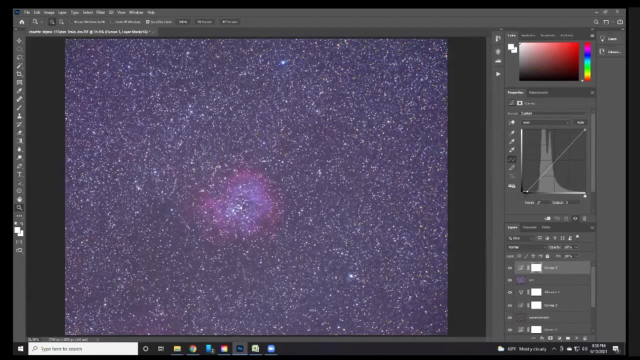 probably do a little bit more stretching and some more curve edits. let's throw another curve edit in there. i'm gonna move my black a little again. i'm gonna just grab the little triangle at the bottom. there's my blacks. do another s curve, add a little more contrast, but not much. 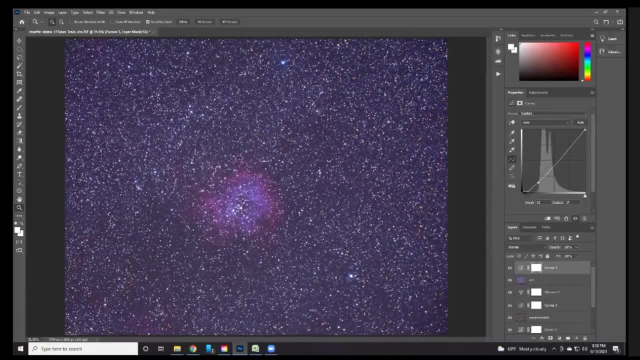 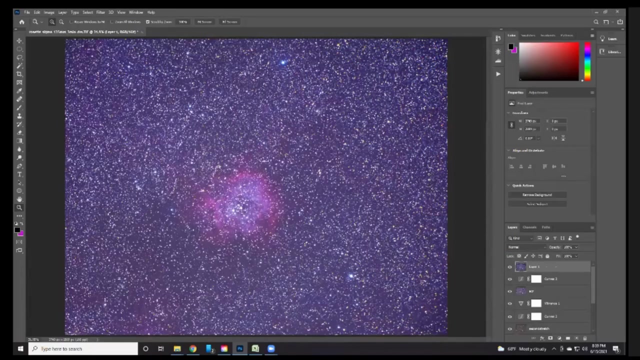 no, that's way too dark, so like that. but now, if i bring up my highlights, there we go. so there we go, all right, so that's pretty good, i'll leave that alone. now one last: i'm gonna do a little bit more um dimensioning, i'm gonna do. i'm gonna go control alt shift b. i'm supposed to turn on my key cast. 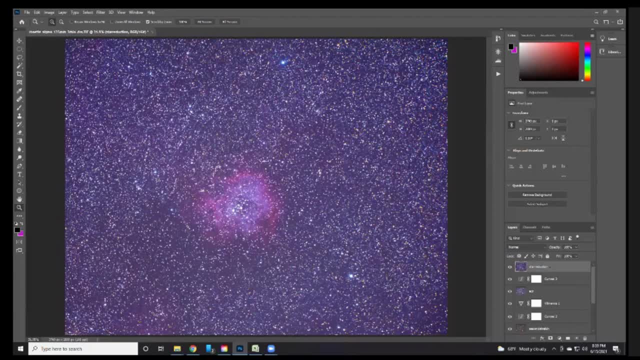 so you can see that i'm gonna do what's called a star reduction, because there's a lot of stars in this, on this target, uh and again. now there's a tool, an outside of photoshop tool, called starnet. if you can get it working on your system, it does a great job on something like a nebula star net. 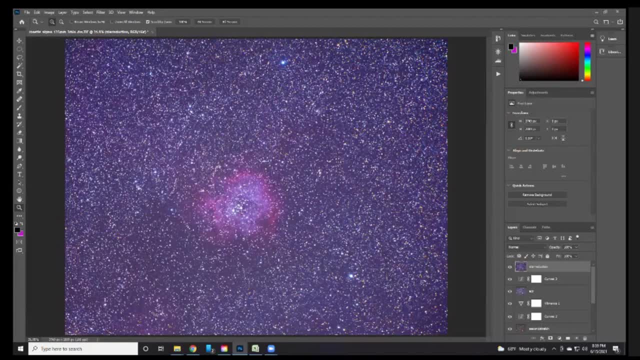 pls plus. so get it to work on your computer. i couldn't get it to work and it will eliminate the stars from your image so that you can work on just the nebula. so i don't i don't promote that product because, like i said, i couldn't get it to work on my computer. but i can do it another way, which is: 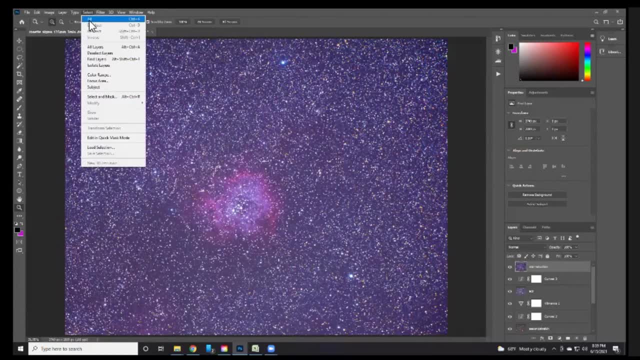 what i'm gonna do right now. so i'm gonna do it again. i'm trying to speed up because i know i'm probably going long here. so what i'm gonna do is, uh, what's called color range selection. so i'm trying to select all those stars and try to kind of knock them down on intensity. so what i'm gonna 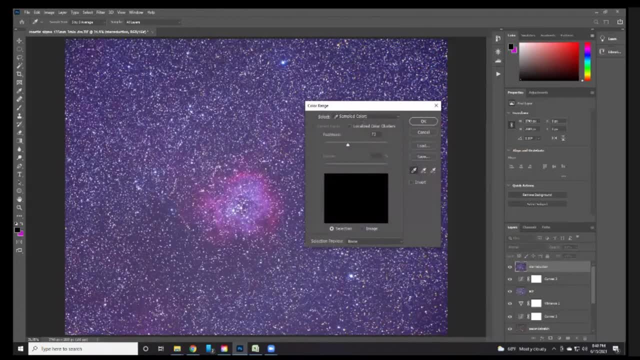 do is a color range and what i'm gonna do is, normally you can use the eyedropper tool to select what you want to affect or select. but what i'm going to do, to make it simple, is go down to here and highlights, because the stars will be the highlights and you can already show it, shows you. 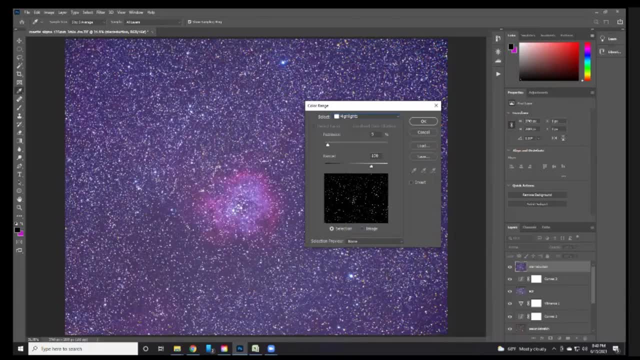 a little bit of what it looks like. you can adjust these things sliders to say, yeah, i don't want that many, or, you know, you just go, that's too much. for sure i don't want to affect those stars. i don't necessarily really want to affect those stars. 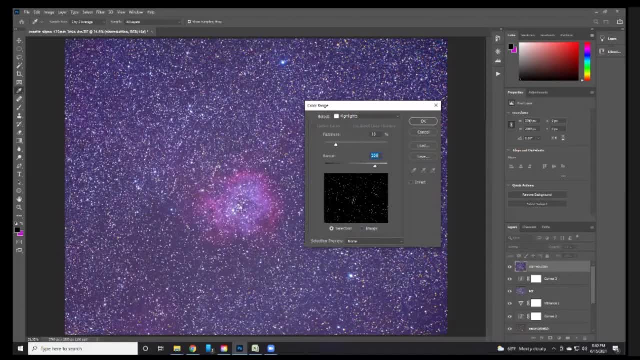 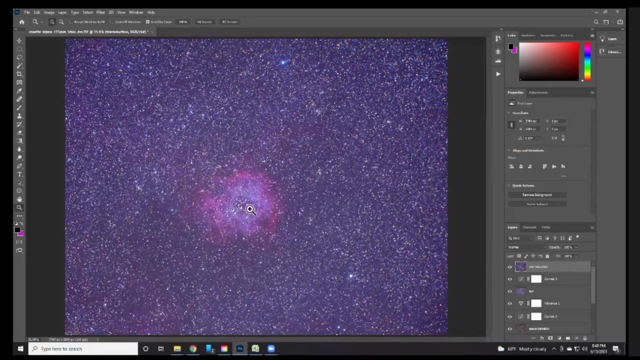 in the heart of the nebula, but why not? and again, you can just keep adjusting these sliders a little bit here and there to get the amount of stars you want to get rid of. so this is just selecting. so it's nothing destructive, you're just selecting. so now you'll see what's called the marching ants. 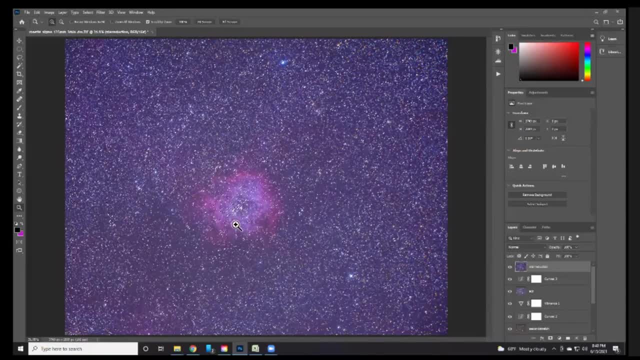 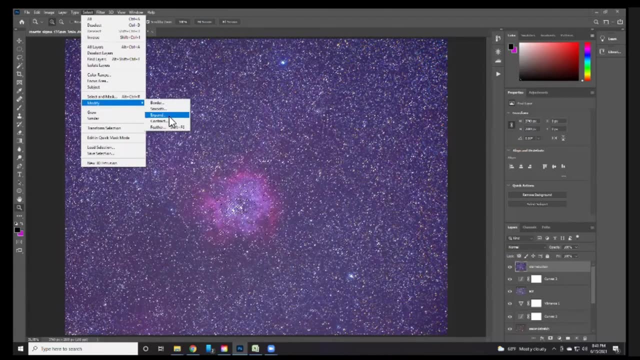 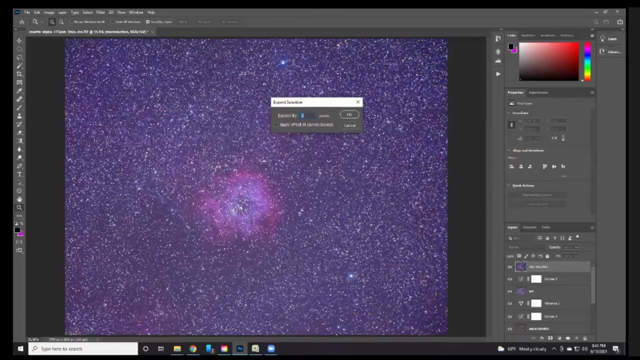 show up, but if you in, you would see that it's really specific on its selection. so what most people do when they're doing this in photoshop is they go in and modify it. so they typically expand the selection so it grabs a little bit of the area around that star. i'm going to do, yeah, two pixels is fine, i guess. 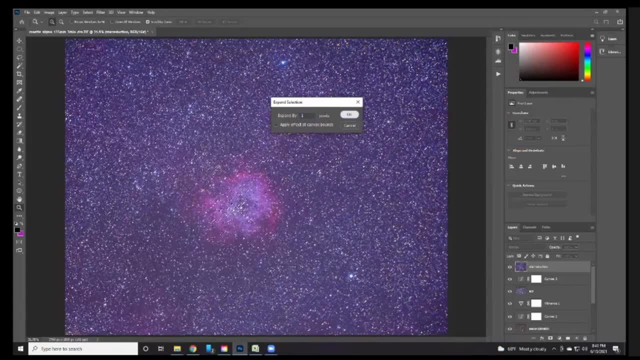 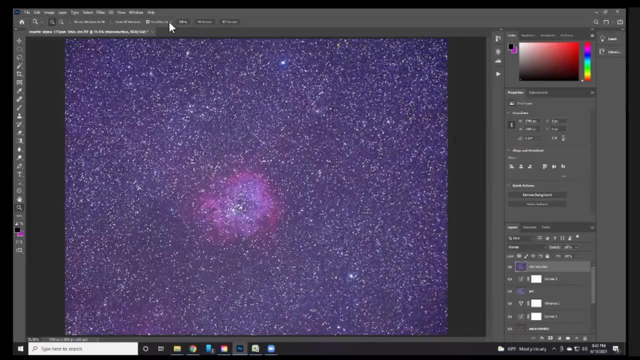 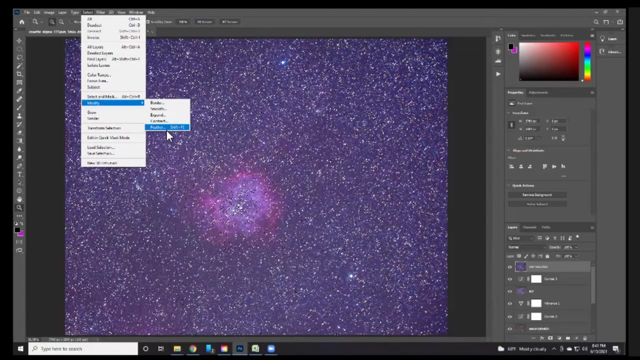 maybe actually i'll go down to one pixel. so it's going to expand my selection by one pixel. so now i've made my selection just one pixel bigger in around what it selected. the next thing is i'm going to do what's called a feather, so again i'm changing my selection settings. so i want to. 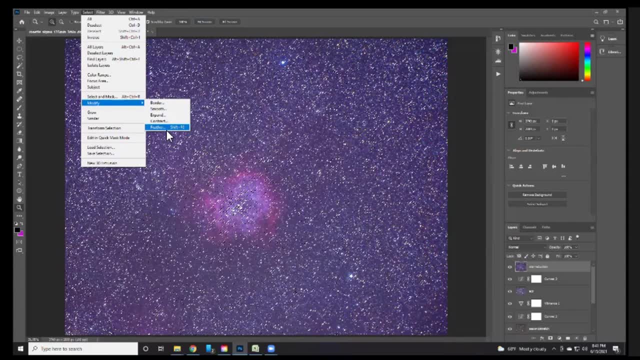 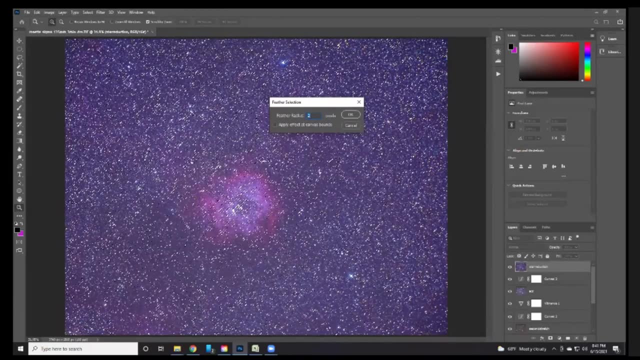 feather now. feather means i don't want a really sharp drop off from the selection, i want a gradual drop off from this selection. so i'm going to feather it by two pixels, sure, okay, that's fine. so i'll say okay, and then i can simply go into now that i've got my 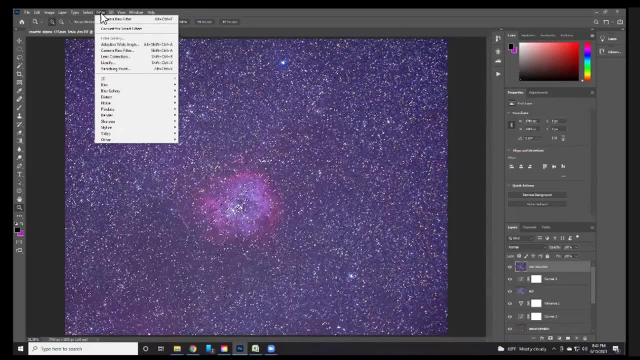 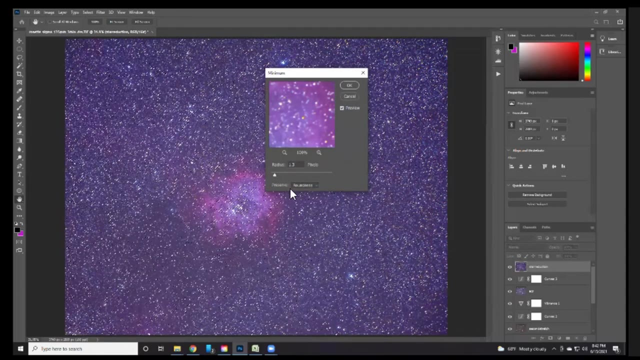 selected that i want to affect. i can go in here under filter and say other there's again. different programs will have them in different places. i'm going to do what's called minimum. it's going to bring up a window. it's going to show me a sample of what i'm doing. one thing you want to do is 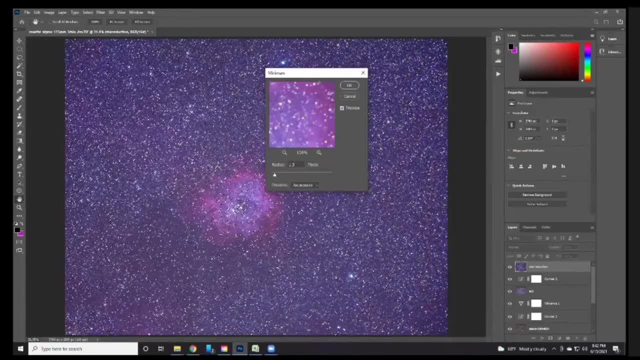 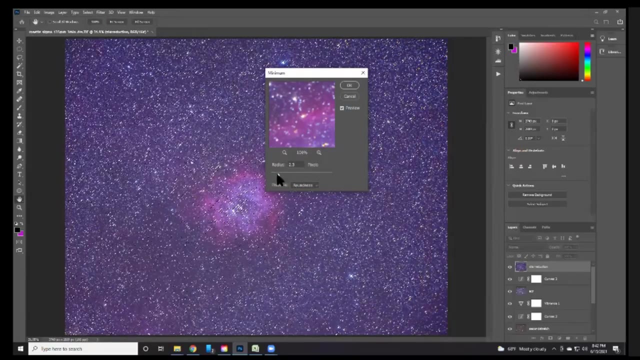 make sure it says: preserve roundness, which of course we want round stars. and then, uh, this slider will show you how much it's really going to affect the stars that you've got selected. so let's try to get to a bigger star. there we go, some of these bigger stars, so you can adjust this as much as you. 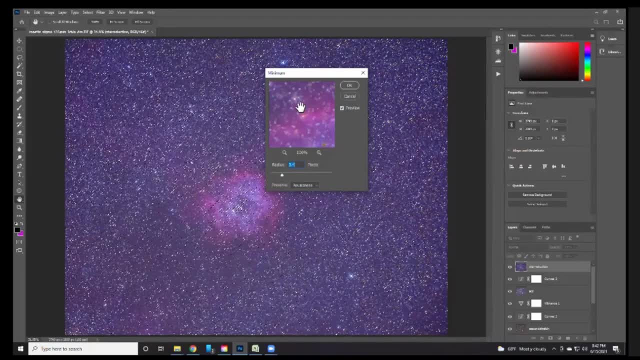 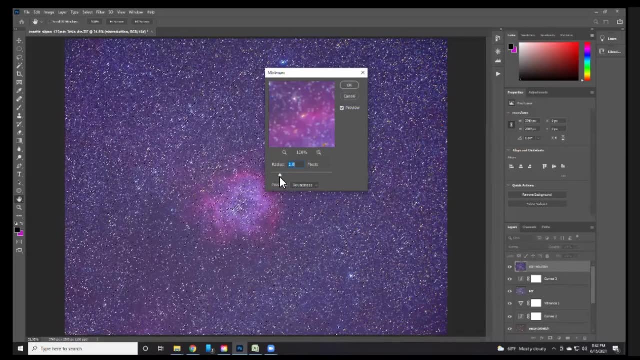 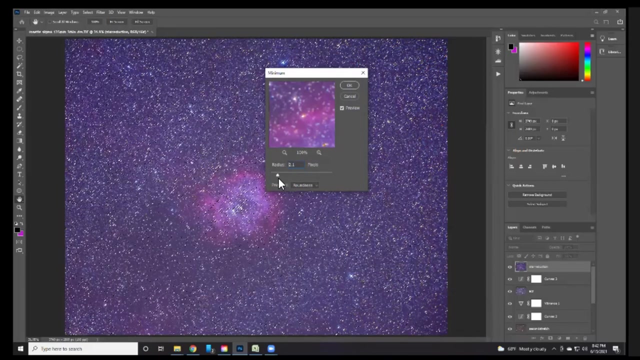 want. you can almost knock them out completely, which is not really probably what you want, because then it'll you'll see that it gets muddy, it muddies the image. so we want to keep a little bit of that star there, not as much as that maybe. yeah, it's probably still too high. i should pretty. 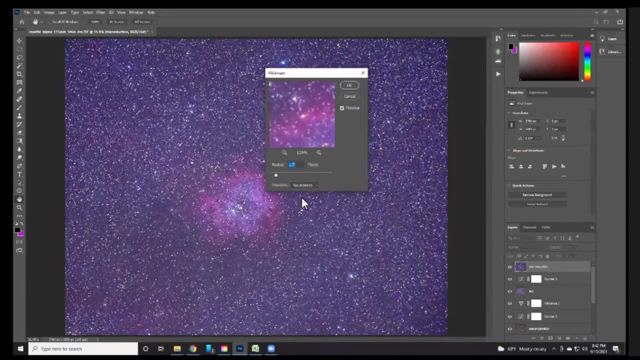 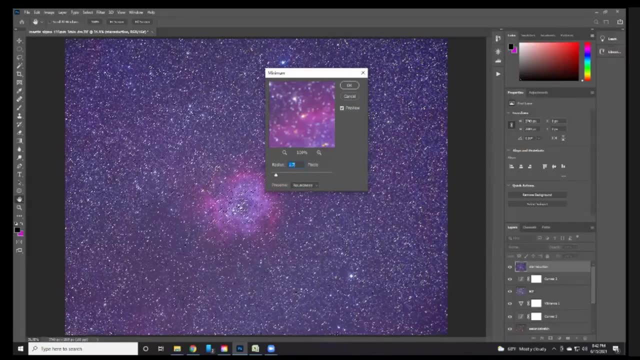 get where i started at 1.7. okay, that's close enough. so i'm going to say that's good enough and uh, you can use the zoom in and zoom out to uh, look at certain parts of the image. so, and of course this is shown in preview, so you click ok and make yeah, it didn't take too long. 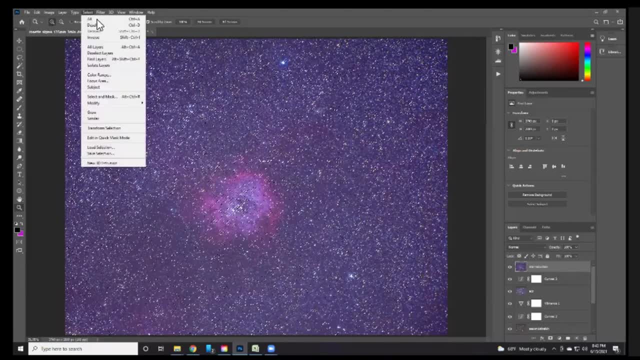 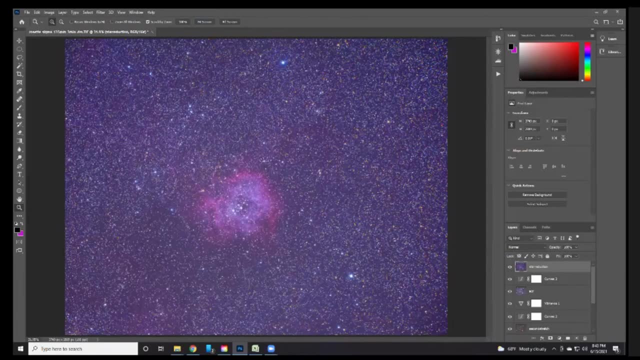 so now you've still got the marching ants going, so you need to turn that selection off. so we go up here to select and then deselect, and there you go now. wow, now i can really see my nebula much better. i've de-emphasized those stars. i still have some stars, some of the bigger. 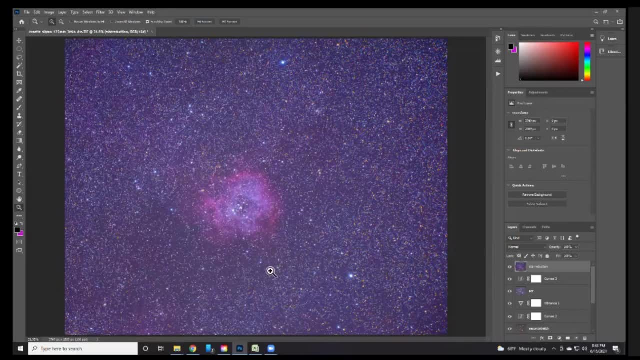 are obvious. So if you're trying to focus on the nebula, that's how you do a quick star reduction. if you can't get some product like StarNet++ to work to do it automatically for you. So again you would think me being kind of the lazy guy who wants to do everything. automated would get. 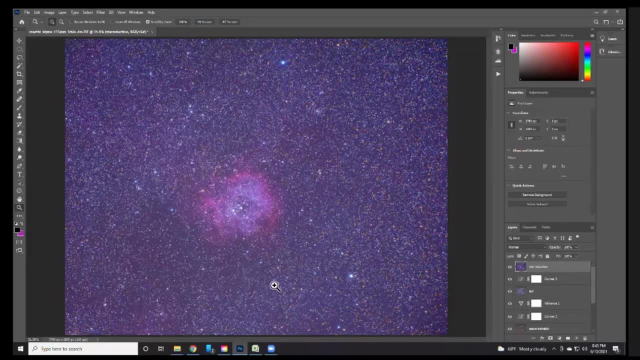 figure out how to get StarNet++ to work, But I found this way to do star reduction and it worked for me, or at least to the point where I'm satisfied. So again at this point, any further edits are going to be almost iterations of what I just went over. Those are your basics Levels. 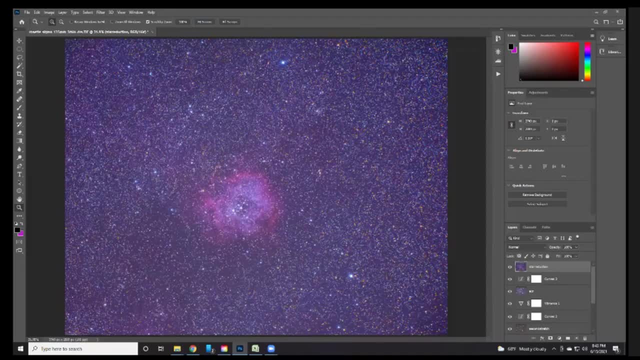 curves, vibrance saturation, hue, color balance- I didn't even do a color balance on here really, but it doesn't really need it on this one. And then the Adobe Camera Raw filter. I almost always use it just because it's got the nice easy to use sliders. And then, if the target 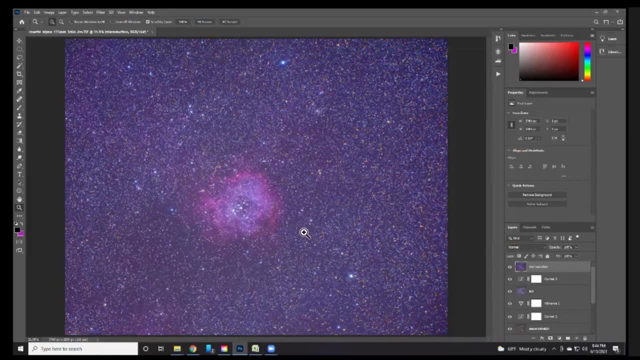 has that many stars around it, like this image did, I would do a star reduction. I don't always do a star reduction because, again, like when you're photographing, let's say, M101, something like that, there aren't a lot of stars around. Well, it's not overwhelmed with stars. I should. 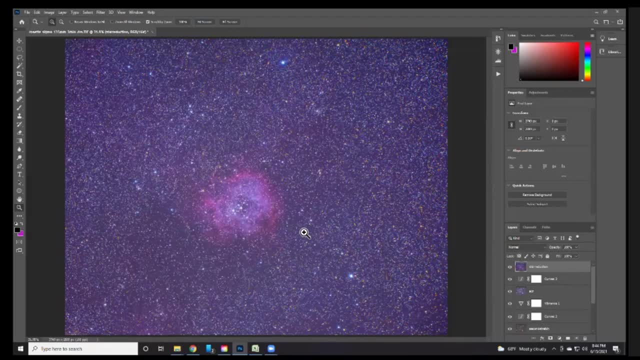 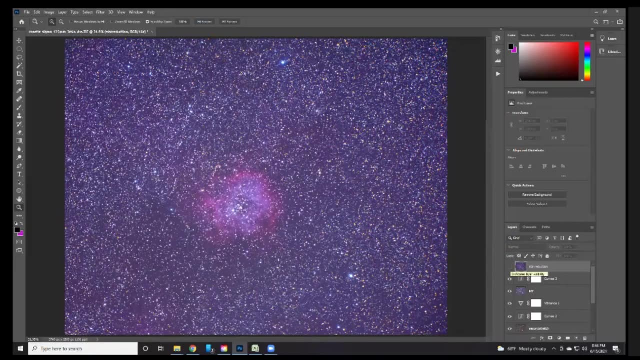 say: And you don't need to worry about them. So you may not always do a star reduction process. And again, even just to show you the difference, you can turn off that. That's with the stars and then star reduction, there's with the star reduction. So that's why doing all these layers and having 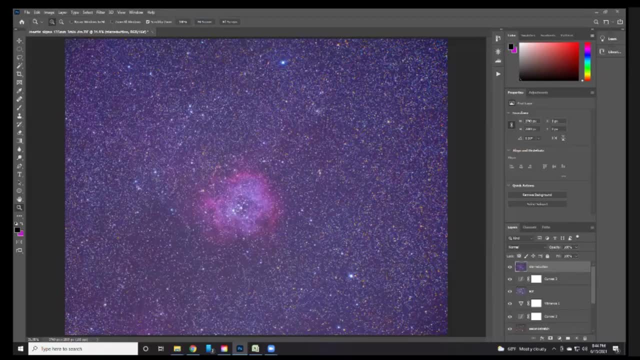 layers available to you is nice. So, going back to the original product, I showed you the one right that comes with your camera, like for me, it's the Capture NX. It may let you do some edits, but it's not going to let you have this amount of control, And that's what you need. 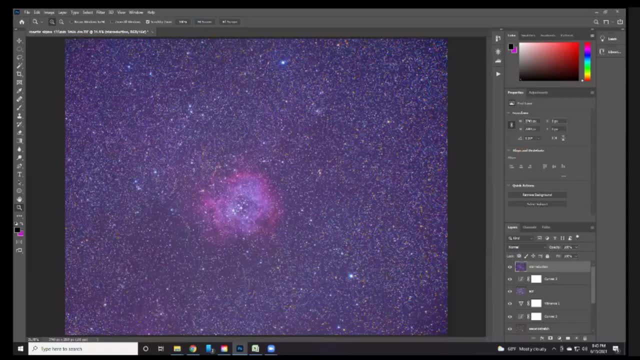 And why you need to do all your pictures in raw format so that you can do this much manipulation of the data that you have, And obviously the more data you have, the better you'll be able to manipulate it. So I would probably crop this down and save it off, And what I typically will. 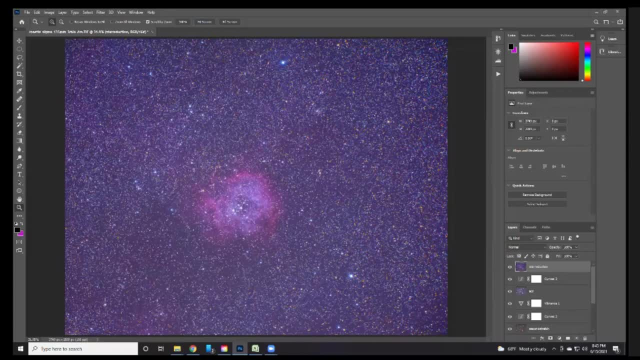 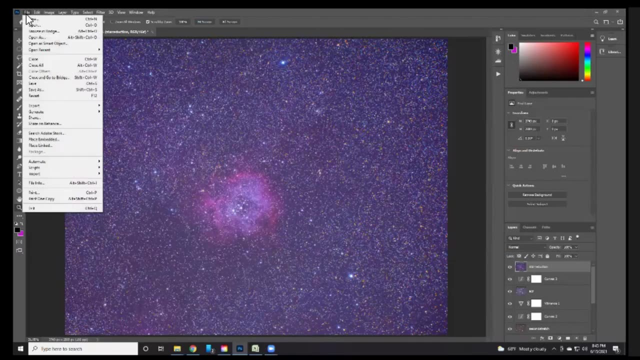 do is save it as a Photoshop image so that I could come back later and tweak all these layers. But then I also almost always export it. So I would go up here to file and export and save it for legacy, for web legacy, So that'll create a JPEG out of it And that way you can post it to. 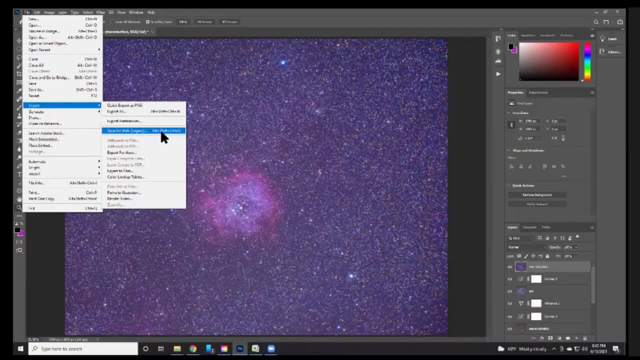 Facebook, like I usually do, or whatever other site you might want to send it to, So that way you can have also a smaller file. if you want to send it to friends and your family and your emails or whatever, You can create a smaller JPEG image out of this. So that's typically the process I go through to. 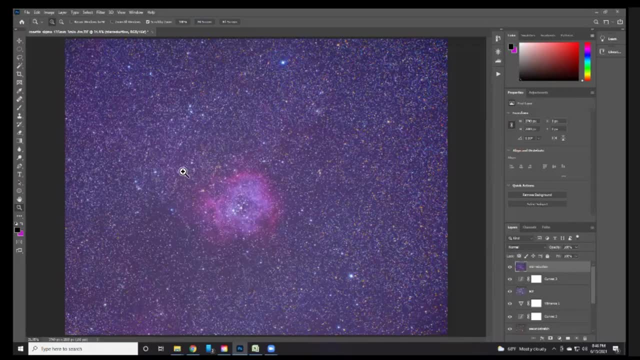 get my images And hopefully you can see how just those basic edits will get almost everything out of your image that you want. Like I said, you can go to extreme levels where you're isolating the individual channels and manipulating those individual channels. But for me, if it looks, 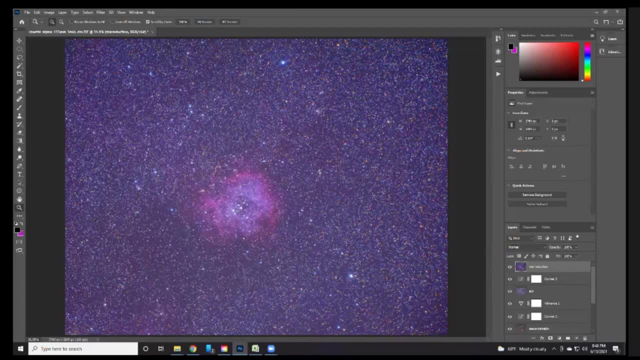 good to my eye. I'm happy with it. So my final processing is what we just basically did. It's called reprocessing. So those cloudy nights and winter nights, you know when it's you don't want to, you want to do something- astronomy. 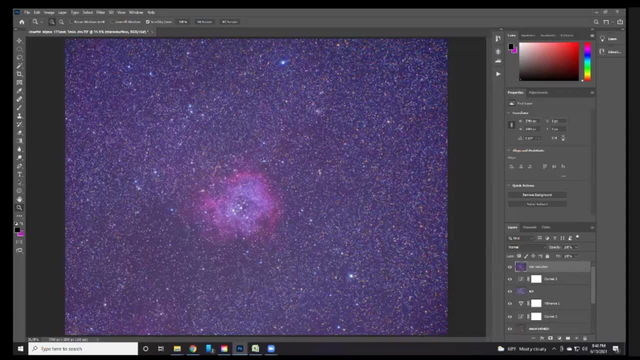 related, but you don't want to go out and freeze, So what I will do is pull up some of my old images and reprocess them. You saw that I had done this also through Sequitur. I stacked it and I pulled it back in here and edited it, And then, almost every time I reprocessed, I had to do it again. 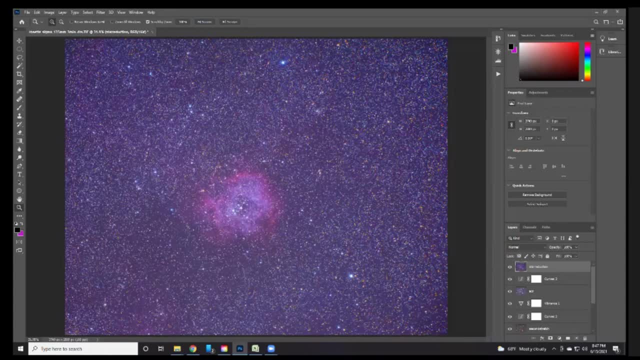 So that's why it's called reprocessing. So that's why it's called reprocessing, So that's why it comes out different And one time it has a much more red hue, Sometimes that maybe have more blue hue to it. So it's something you can do to go back And again it's kind of one of those reasons. 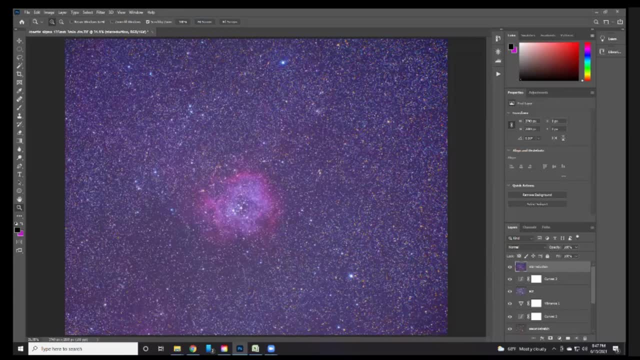 why I keep all those files, so that I can do a restack of the raw images, raw files. Some people, once they stack it, they throw away their raw files because it does eat up a lot of disk space. So that you know, obviously is up to you. 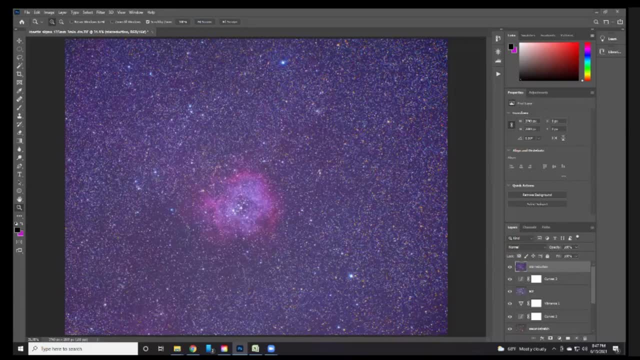 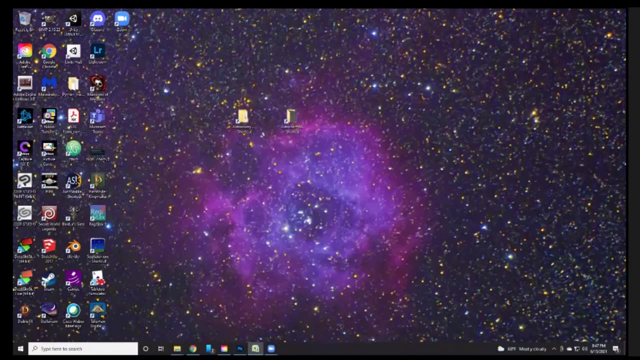 And how much disk space you have. So this image, if you noticed early on in the presentation, is my background. I did save it and you can see it looks quite different- Look how much yellow the stars are in the background on this one- than what we just did. So I would say I almost like 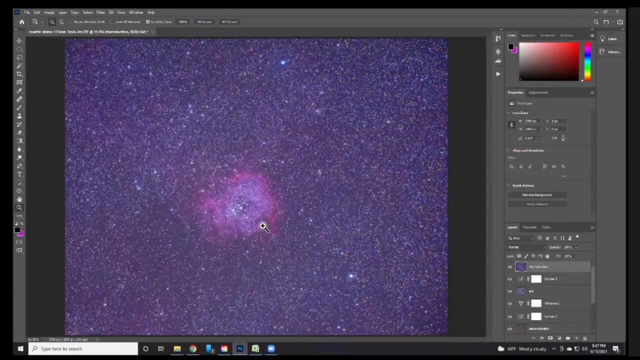 this one better than the previous one, So maybe because it's just cropped a little bit differently. So that's my final step is what I call reprocessing. So, Drew, or whoever is managing things, do we have any questions? or We don't have any new ones that have popped up in either of the feeds for me. So 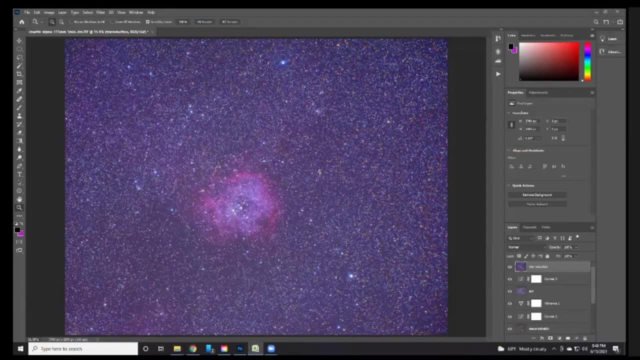 I think we're doing it. I guess I had one question, if you don't mind, Sure, Yeah, no, go ahead Along the way. I've done a lot of computer work and a lot of image processing of various sorts over. 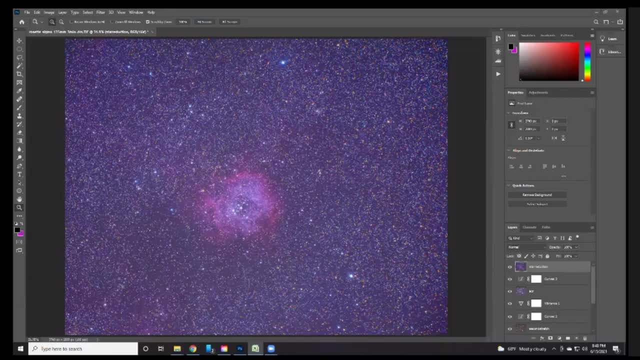 the years, And I know that you might just think of it as the automatic thing that Photoshop does, But I was wondering about if you have a practice of saving your files along the way while you're doing things. Again, for some people it's just like if you have Photoshop set to automatically. 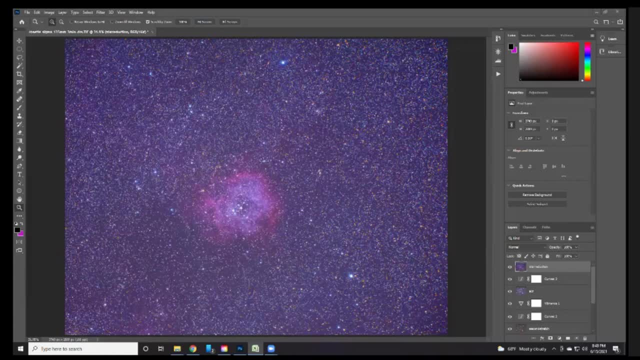 save for you periodically. it's something it's doing, But in some other programs it might not have that. So, Yeah, Yeah, And actually it's funny you mentioned that because, like I said, they just recently did an update to the Photoshop version I have and it's been crashing more often. 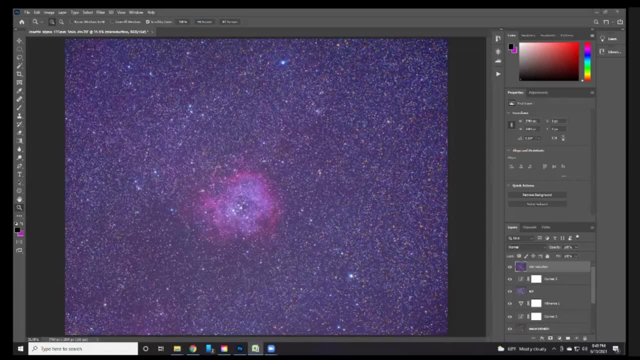 And I did lose my entire edit that I had done up to that point. So it's for me- my edits are simple enough where I think, even if it doesn't save in the middle of my edits, that because I don't think I have automatic, automatic saving set on here right now, mainly because I just I want my processor. 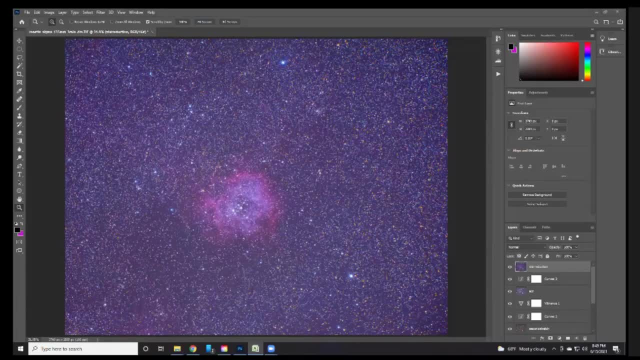 focused on what I'm doing, not what it wants to do or what some program wants to do. So, yeah, I mean it's definitely something you should be mindful of if you're, if you're working on a slower system or system that's not as beefy as mine. Yeah, you probably do want to save quite. 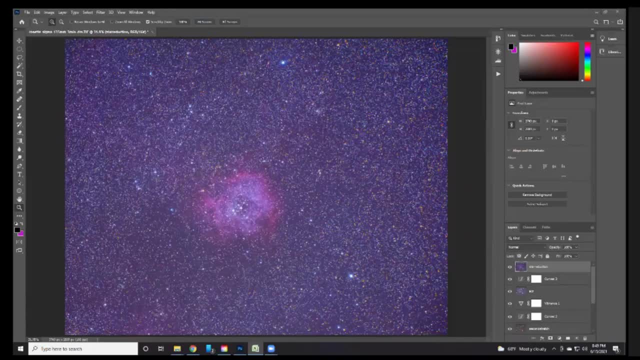 frequently because you know trying to get it back to the exact point is it can be really hard because unless you're writing down numbers, I mean you can do that, You can. you know, you can pull up the eyedropper and say: tell me what exactly this area of the image is. 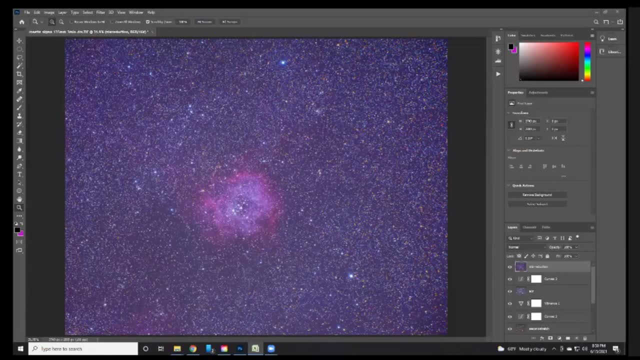 That's what. what's the RGB values of every little pixel in there? And you know, if you're to that level of editing, yeah, I'd be constantly saving, But for me, if it looks pleasing to my eye, that's for me. Again, I can redo these edits. 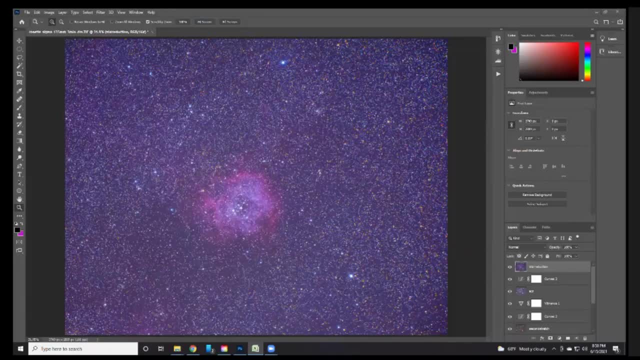 pretty quick, so I don't necessarily bother with it. But yeah, I know some people do save quite frequently, So otherwise you're just getting compliments on the good talk. So that's what's popping up. Oh well, I appreciate those who are watching. 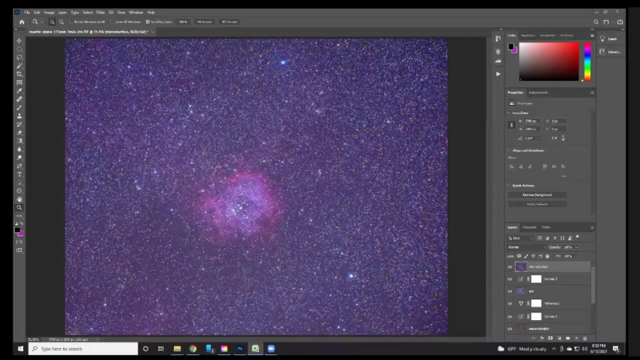 And I hope you know, once we do post this up to YouTube, that people will go over there to the NAA SWAB channel and to the video and subscribe and like our videos. Okay, well, thank you very much, Chris, from all of us out here in the audience. We. 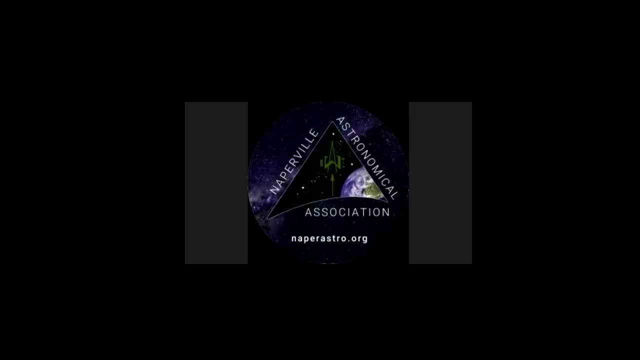 really appreciate you sharing your experience and your expertise with us. No problem, I guess we're ready to sign off folks Again, as Chris just noted, if you're watching us on YouTube, hey, you know, subscribe And you'll get notices when we post new videos.